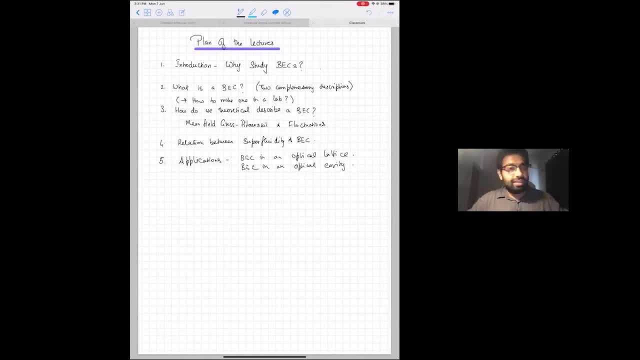 So we'll begin with an introduction. The introduction will be, of course, the key question for anything that you start studying or learning about: why the hell do you do it right? So, with that said…. But the point is be students, because if you didn't know anything about, 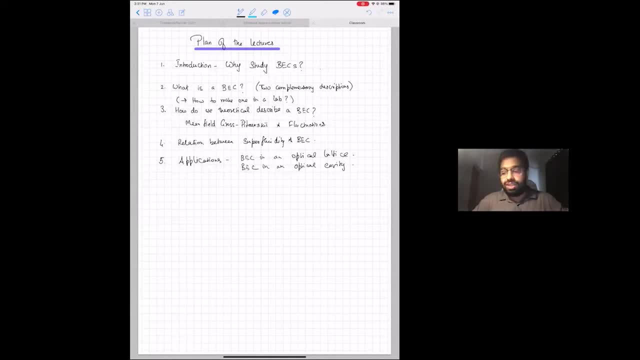 this. no one would need to. So let's get started and get going. So let's get started, So you will have the necessary ID in your ID, And when I do mnemonics or gib- And if you're new here, you might already know how it works actually. 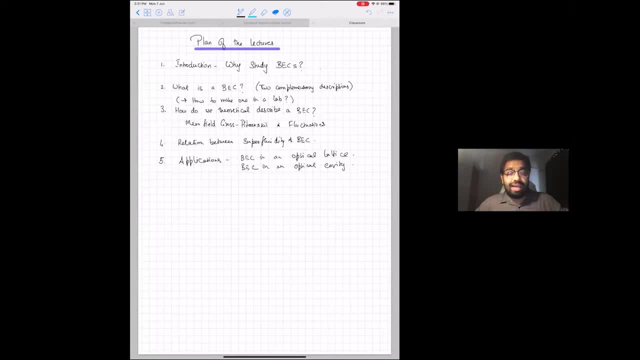 So I will. so I'll get those people will give me some information. All right, I will take a mediterranean shot point where we will begin our sort of theoretical description of a cosine strength condensate and we will go into two slightly complementary descriptions, one of which might be somewhat. 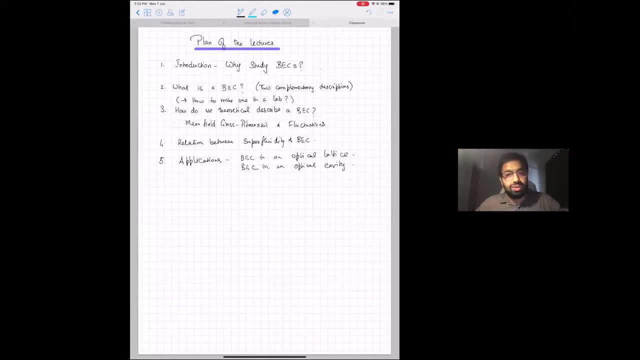 familiar to you if you've taken a graduate course or MSc course in statistical mechanics, and a slightly less familiar version of it, which will introduce some of the mathematical machinery needed to go on to the third thing I'll talk about, which is: how do you theoretically describe 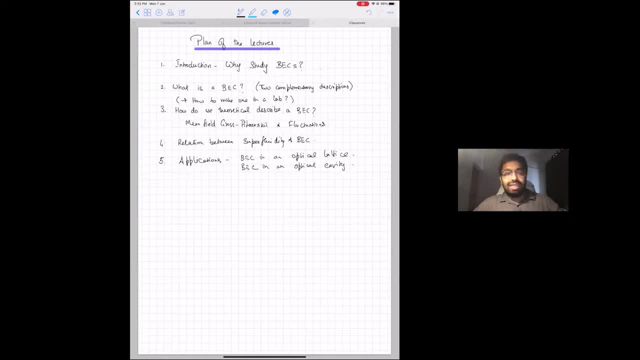 a cosine strength condensate. There will be two descriptions I'll try and cover. one will be using what's called a mean field theory or Grosbe-Taweski equation, and then a little bit about fluctuations, about this mean field. So my hope is that I would get. 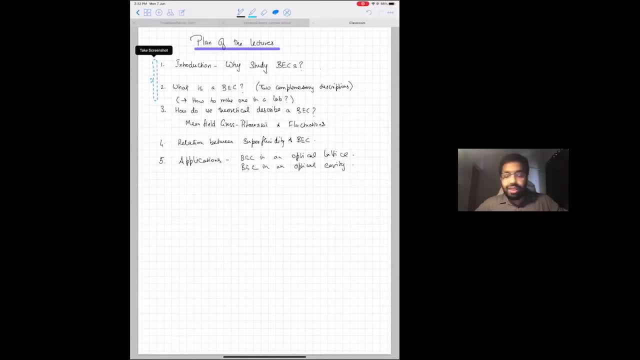 through these two topics by today and somewhat around half of tomorrow, and then we will begin this sometime late tomorrow and, if there is some time, by the fourth lecture we will. I'll discuss a little bit about the connection between superfluidity and cosine strength condensation, which is a very important topic historically and also now more current. 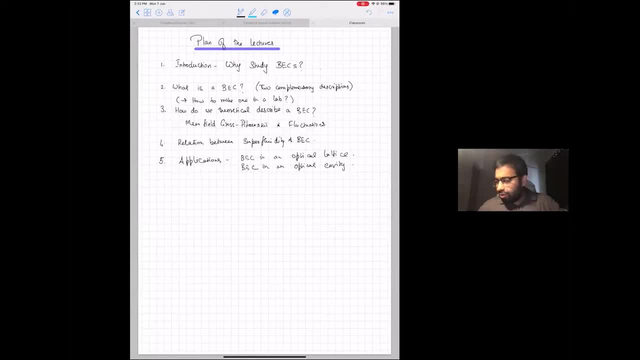 experiments that have been going on And irrespective of how much of the theoretical machinery and the theoretical background I covered by the first four lecture, I will. I would have enough sort of we would have enough background at the point when we finished four lectures to have. 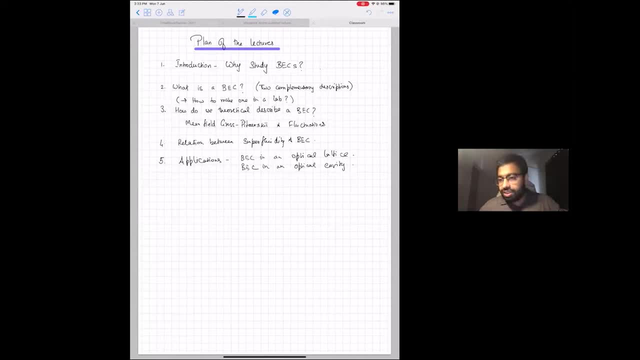 a fifth lecture which will be a little bit different. It will not be a chalkboard or like writing, like I'm going to be just writing on this iPad. it will be a different type of a lecture. The last one will be a little bit like I give a talk, essentially covering a couple of very important 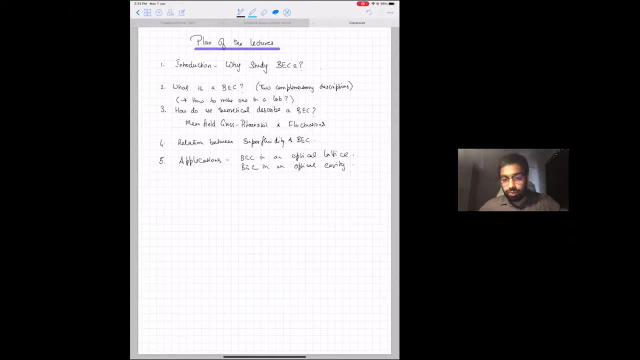 experiments, one of which is regarding one set of experiments regarding Bose-Einstein condensates in optical lattice and another one concerning Bose-Einstein condensates in an optical cavity. So the former is historically really important and it's one of the big success stories of Bose-Einstein. 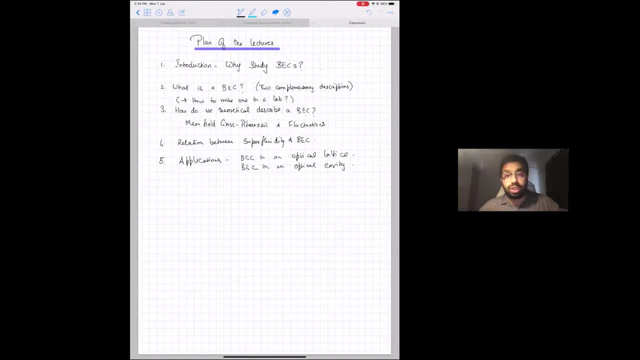 condensates. So it serves to give you an exposure to what are the possibilities with Bose-Einstein condensates. The second one is essentially again something that is very close to my research interests and hopefully that will be inspiring for some of you to get in touch with me. 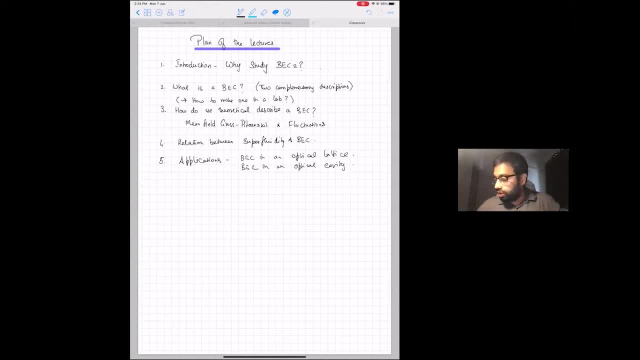 if you're interested in, you know, talking more physics or working with me. Okay, so that's the rough outline. so with that, let's move on, and let's start with the first part. what is okay? so then, one small thing I forgot to tell you is how I would like to run the. 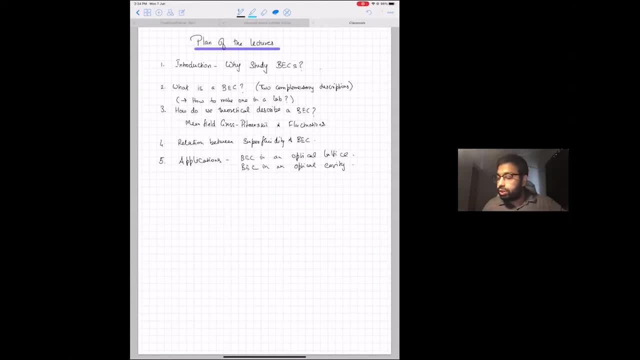 run the lectures. So what I'm going to do is I'm not going to talk longer than 30 minutes at a stretch, whatever happens. so it would be nice, irrespective if it will be 30 minutes or less, if there is a logical point of before 30 minutes which I can stop and ask. 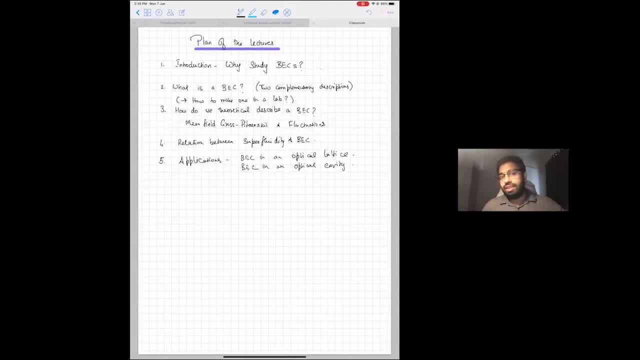 questions. ask you for questions. I'll do that. if not, definitely after 30 minutes, wherever I am, I'll just stop and then we'll have a, we'll have some questions and that that would be very nice if some of you can ask questions, because that will keep me on my feet and also it will make things more. 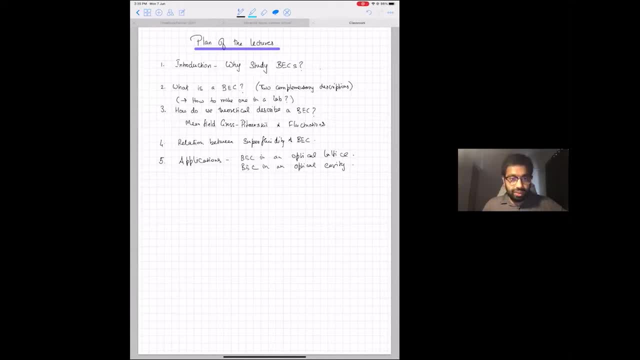 interesting and, as always with everything that I do in terms of pedagogy and teaching, the goal is not for me to, you know, tell everything that I plan to tell you, but it's more to use whatever I'm saying as a point to hopefully excite you. 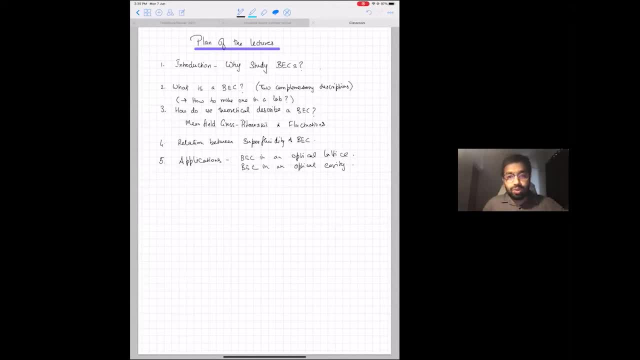 regarding this field and- or even better bonus- have a good discussion. okay, so both are welcome, and that's what I'm looking forward to, and I hope that that will go well. okay, all right, so I'm going to ask this first question: why do you want to study BECs? okay, so now to answer this. 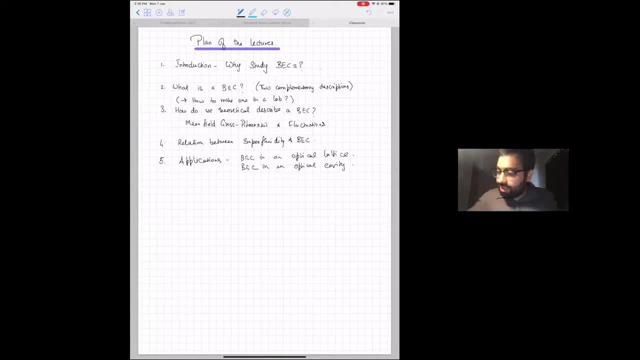 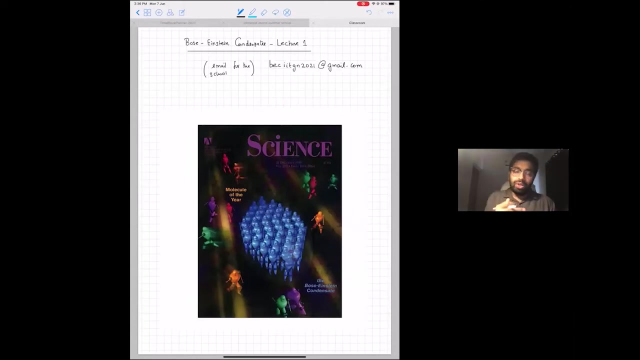 question. of course, you have to have some idea of what a BEC is, without which this question is somewhat opaque and meaningless. so let me begin by saying what a Bose-Einstein condensate is. I'm going to start literally with very cartoonish definition, and you will get more and more specific. 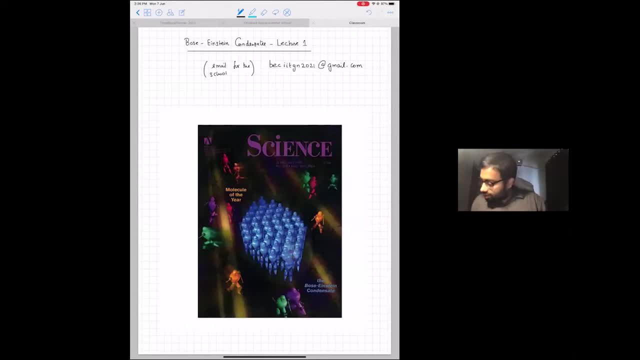 and rigorous today. okay, so here is a picture: sometime in the 90s, when the first atomic Bose-Einstein condensates were realized. this is a picture from the cover, as it says, of the science magazine, and what it is showing you is basically a cartoon version of what a Bose-Einstein condensate is. so a Bose-Einstein 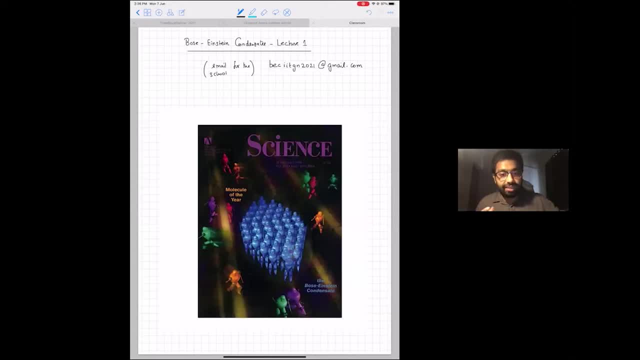 condensate is a very interesting collective state, collective quantum mechanical state of matter, where many, many atoms, many, many particles- I'll be using particles and atoms interchangeably, please do not mind so- many, many, many particles occupy the exact same quantum state. when you cool such a collection of particles. 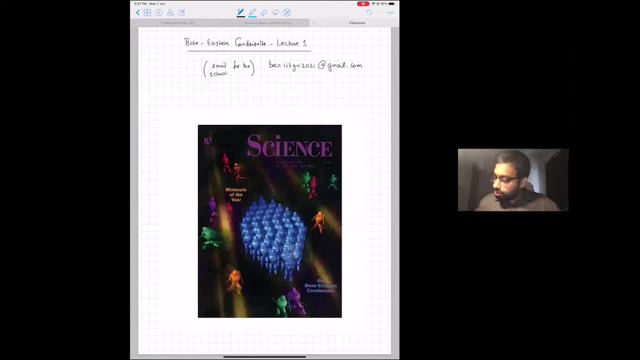 below some critical temperature. so in this cartoon, these blue particles or these blue soldiers, are supposed to signify all the atoms that have completely gone into the same quantum state. so if you know, a quantum mechanical state is like a wave and you can see that each of these atoms, these soldiers, are moving lock in step, which means they 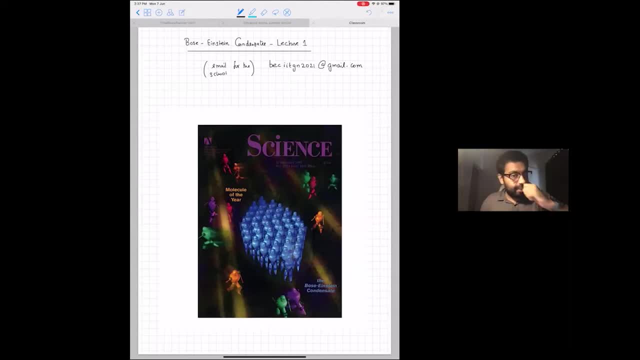 have the same phase. they are exactly in the same quantum state. now, these other particles of different colors that are moving around helter-skelter- you can see that these atoms are in blue color, which means they are colder, and these atoms, that are, all these particles that are running around, are basically a background gas. 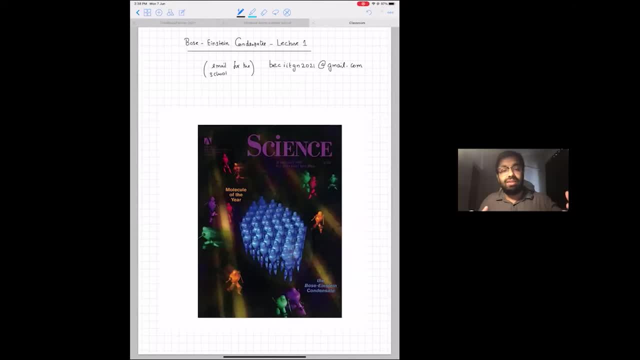 that is in a regular thermal state with some Maxwell-Holtzman distribution and they are still there. but you basically have a macroscopic fraction. this is a very large fraction of the total number of these soldiers here. they have gone into this ground state and this is a Bose-Einstein condensate. 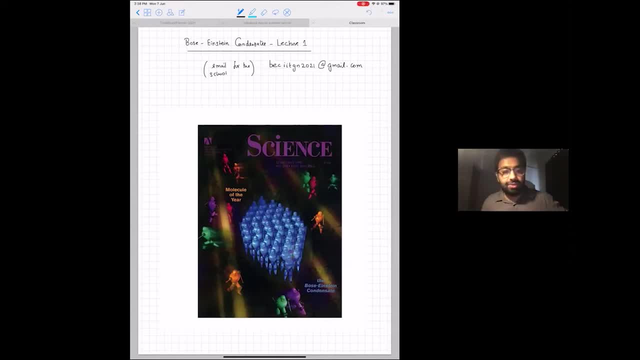 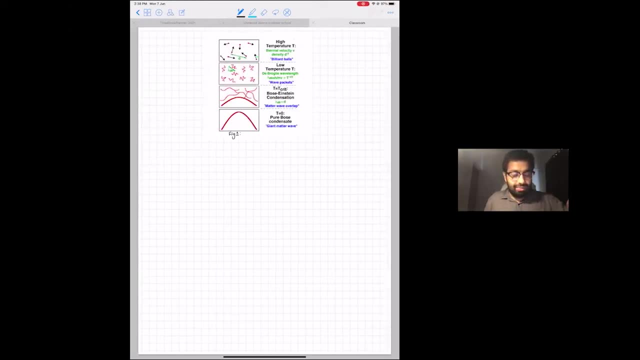 okay, so this is like a very naive definition, cartoonist definition, and so let's move on and look at slightly more uh, specific definitions. okay, so now, as I said, uh, there is. so the idea for uh, for Bose-Einstein condensates is that you keep lowering the. 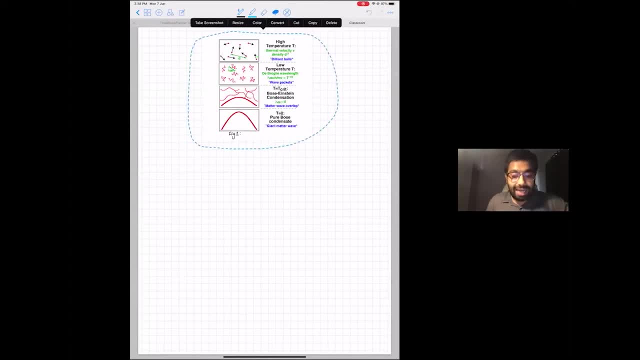 temperature of a collection of particles that have a particular statistics, which is called Bose statistics. so bosons. and when you cool these particles below a certain critical temperature, you have a critical temperature. a macroscopic fraction of them occupy the same quantum state. so what is this? in that sense, every atom is in the same microscopic state, which means, for example, if I 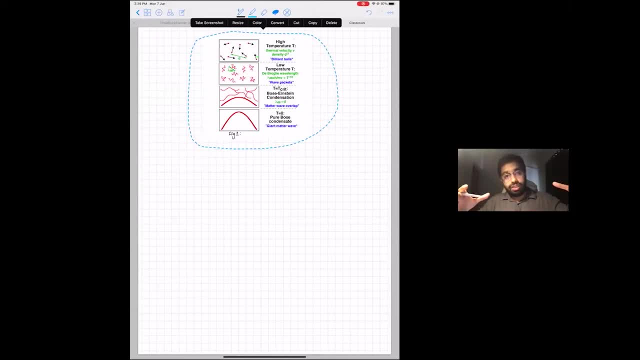 have a box that is without any potential, a three-dimensional cubic box, all of my atoms will go into the zero momentum, or a large fraction of my atoms below this critical temperature will go into the momentum zero state and suddenly stop moving. on the other hand, if I have a harmonic oscillator, as we will see most of, 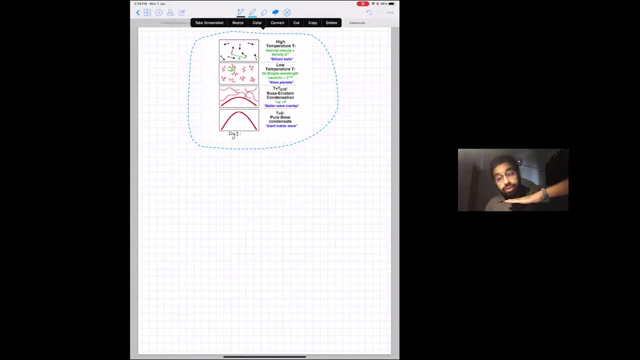 my atoms will go below this transient temperature into the ground state of this harmonic oscillator. okay, so when this happens, since many, many of these atoms basically occupy the same quantum states, you essentially get a very large atomic matter wave right, or a particle wave, and this effective macroscopic state is quantum state, is called a Bose-Einstein condensate and already. 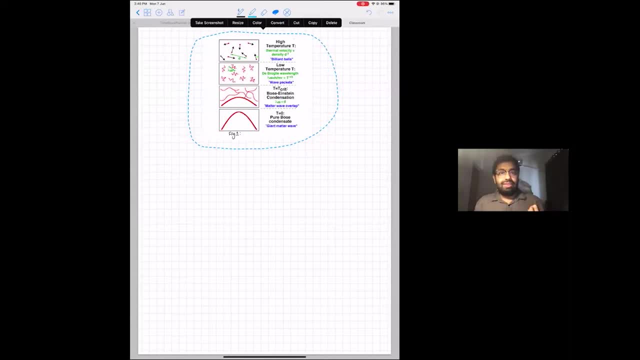 there is an idea for why is this interesting to study such a state? basically, if you think of how you learned quantum mechanics in school, in sorry, in your courses in your first year undergrad or second year undergrad, you would have learned about a single particle in a hydrogen atom, an electron. 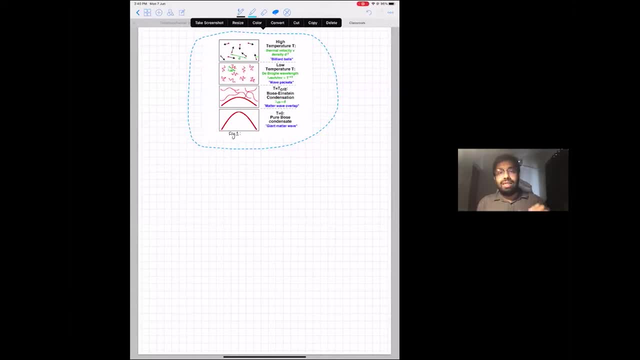 in a hydrogen atom or for some very small number of particles, typically in some very special conditions. they obey these laws of quantum, or at least the they obey the laws of quantum mechanics at all conditions. but your manifestation of quantum mechanics is never at very large scales. if you're looking at macroscopic systems, you do not see an very simple manifestation. 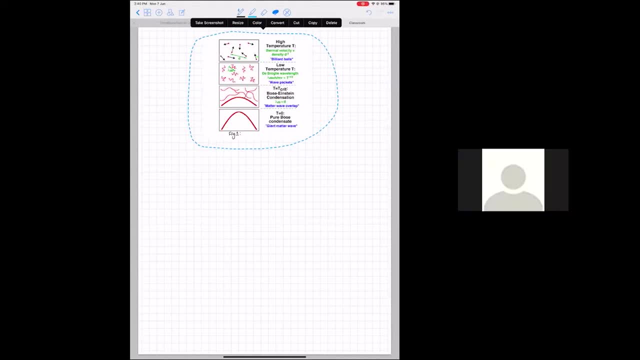 of quantum mechanics. but this Bose-Einstein condensate is in some sense like a direct counter example, where your quantum effects are amplified precisely because many particles are participating and collectively occupying a quantum mechanical state. so you will be able to amplify all the non-intuitive features of quantum. 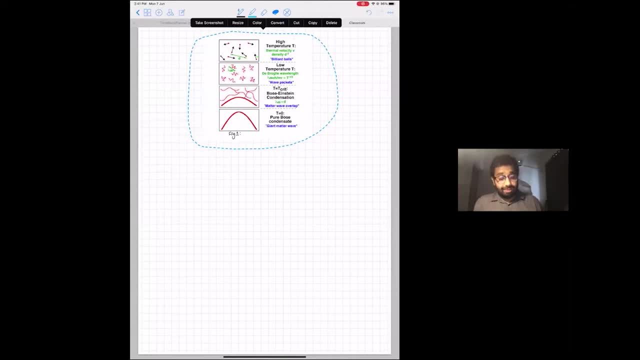 mechanics. so that's sort of the idea with these, with these Bose-Einstein condensates. so now let's first make and back of the envelope, uh, understanding of when do you have Bose-Einstein condensation and what do you mean cooling, and how, how does it come about? okay, so to do that, I'm again putting up a 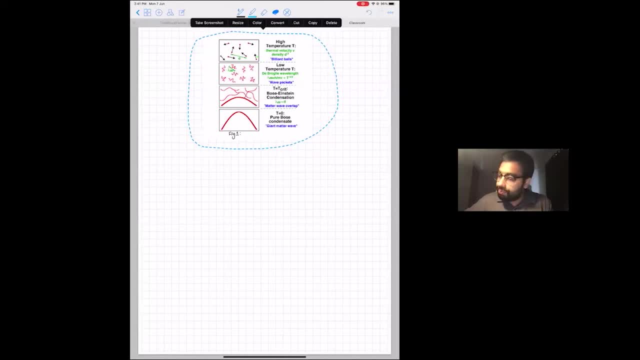 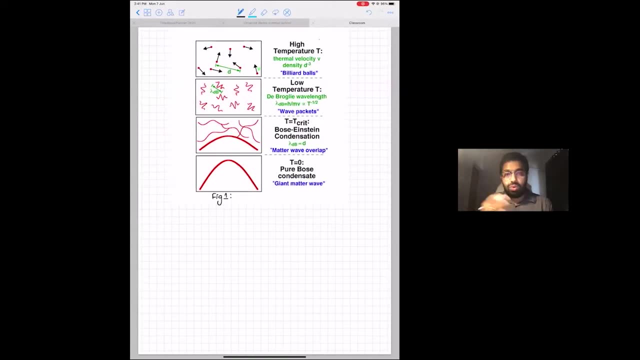 cartoon here. so let me just resize this a bit and then I'm going to describe: uh, what's what, what, what? how does a Bose-Einstein condensate come about based on this very simple cartoon picture? so, uh, what, what is this showing? this is showing basically what happens to a gas of uh. 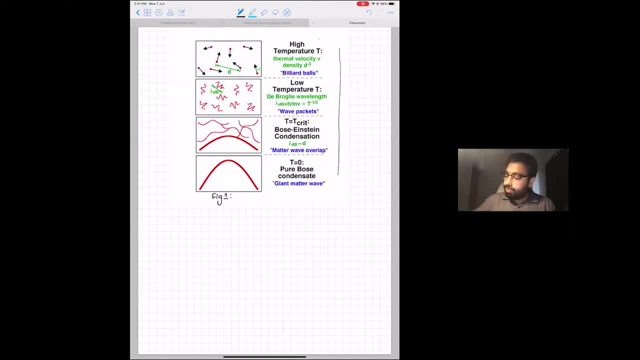 atomic particles as you keep lowering the temperature. temperature is going lower and lower here um, and at very high temperatures you essentially have very uh. basically we understand this part really well. it's just uh, Maxwell-Boltzmann distribution of atomic velocities or, if you want, just simply ideal gas. these are completely non-interacting bosons. so you can think of. 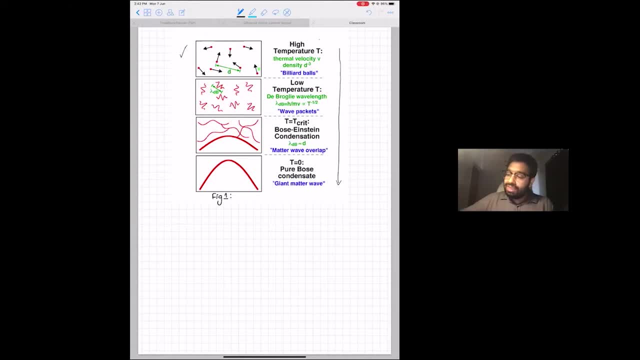 these particles as just billiard balls. but one thing that is interesting is, as you keep going to lower and lower temperature, uh, the de Broglie wavelength of these particles will increase. so let us define what do we mean by this de Broglie wavelength of these particles? so what we are talking about is a very particular 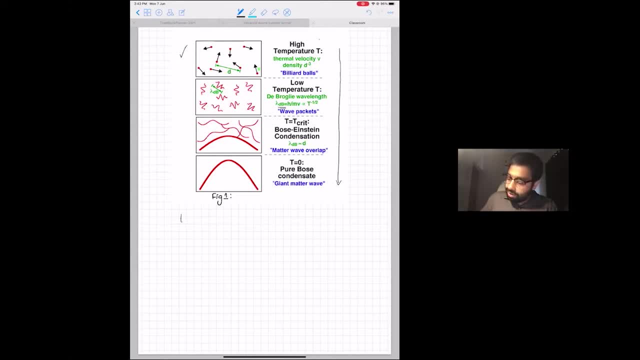 kind of de Broglie wavelength where which is called the thermal de Broglie wavelength. okay, because we know that, at the end of the day, what we know from the Broglie theory is that all matter, all particles, have a wave nature and the wavelength corresponding to that wave. 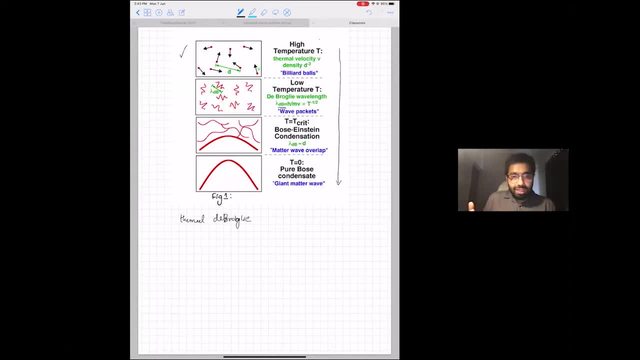 nature is fixed by the momentum of the particle, and the momentum of this particle that is at some temperature T, we can estimate it very nicely, okay, by just using- if this is just a box uh of free particles, no potential, nothing. the average momentum you can estimate by taking 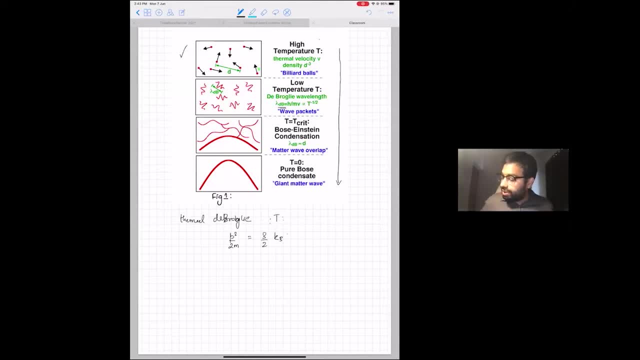 P squared by 2m is equal to 3 by 2 kVT. right, so just simple thermodynamics or or even statistical mechanics. then your P, your average momentum scale at some temperature T, is nothing but square root of 3m kVT. okay, once you give me a momentum, then I can actually write a corresponding. 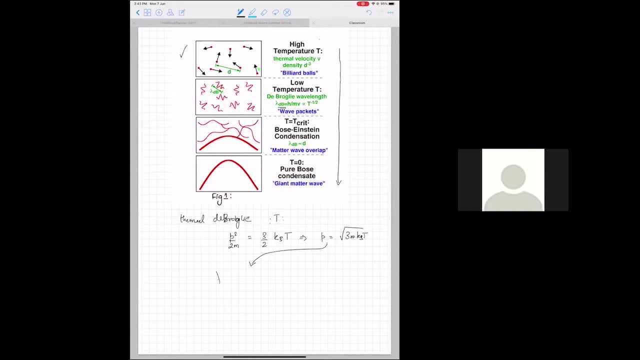 de Broglie wavelength corresponding to this momentum. this is my thermal de Broglie wavelength, H over T at some temperature T. so when I write it out it comes to roughly H over square root, 3m kVT. okay, of course. uh, in some conventions there might be some other factors floating around. but for 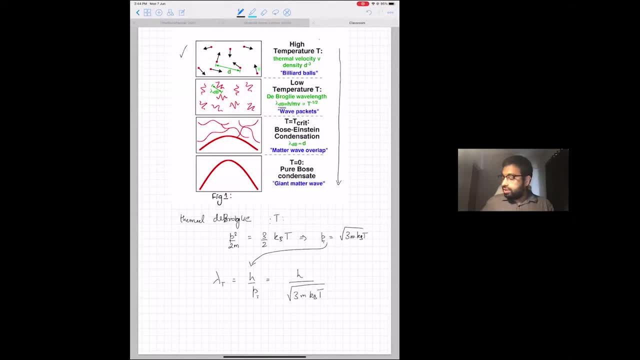 simplicity. the most important thing is it goes as one over the square root of the mass and one over the square root of the temperature. okay, so now this cartoon. what it is trying to describe is basically the very interesting and important fact that, as I keep lowering my temperatures, my de Broglie wavelength keeps becoming larger, and 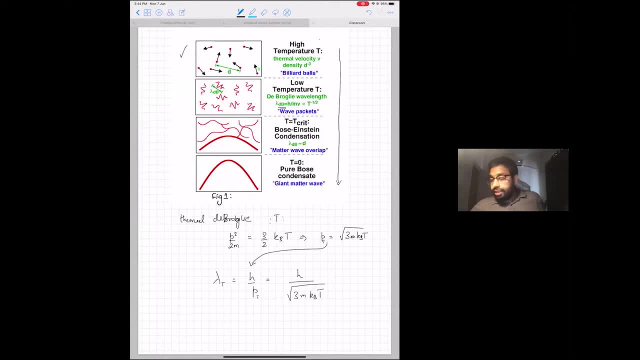 larger and larger. at some point the inter-particle spacing becomes comparable or even lesser than the de Broglie. essentially, when the de Broglie wavelength becomes extremely large, much larger than the inter-particle spacing. basically, then, you cannot distinguish between the atoms and you. 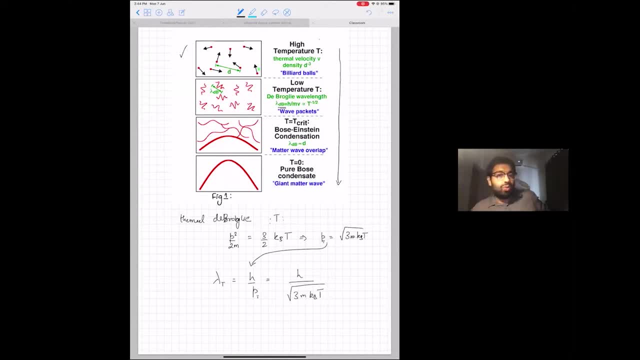 get a wave right. and this giant matter wave is what a Bose-Einstein condensate is. and this giant matter wave, complete giant matter wave, you get at T equal to zero, but at some intermediate temperature scale- called this critical temperature- already a large collection of particles. stop behaving like 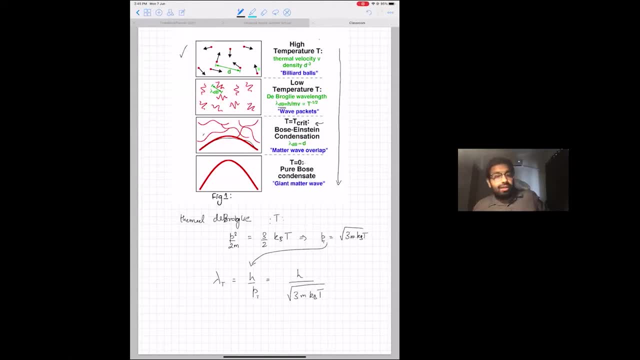 individual atoms but behave like a matter wave, and the temperature at which this develops is called the critical temperature, and below this point we say that part of our particles have gone into a Bose-Einstein condensate space. okay, so let's, let's estimate this thing a little bit to get a sense of numbers as to how and 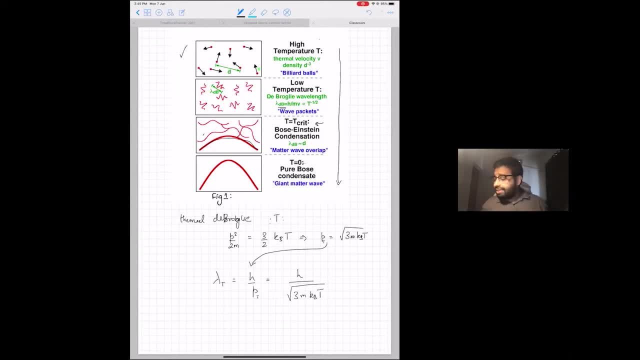 when such a thing would happen. so to do that, let's simply consider: uh what? why does this happen? there is an important feature that I did not mention here, which is since I have completely non-interacting particles and I have no potential in this picture. the only quantum thing that I have is statistics. so when I said once this be Broglie wavelength. 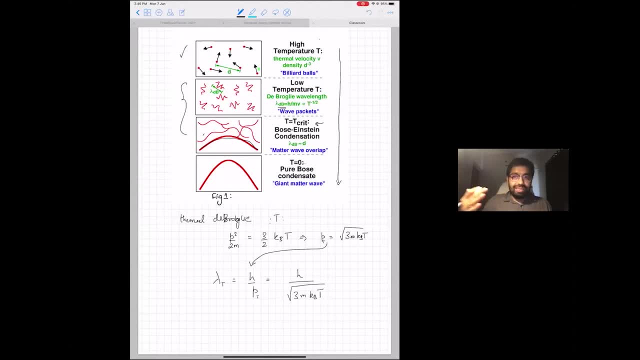 becomes larger, I cannot distinguish. this comes within. this is the idea that these particles are identical and they are statistically indistinguishable and they have this bosonic statistics. okay, so that is an important feature that allows you to, that prevents you from distinguish between, distinguishing between these particles. okay, so with that, let us now do a little. 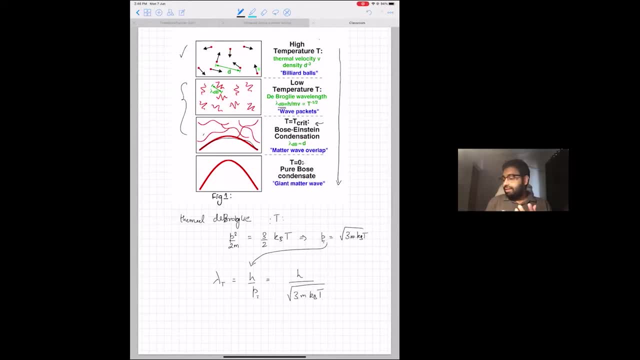 bit of uh back of the envelope. estimation of what is. how does temperature affect things? what is the typical inter-particle spacing and and how would you make a? how would you if you wanted to make a Bose-Einstein condensate? what are the challenges? okay, because this is. this was originally proposed. 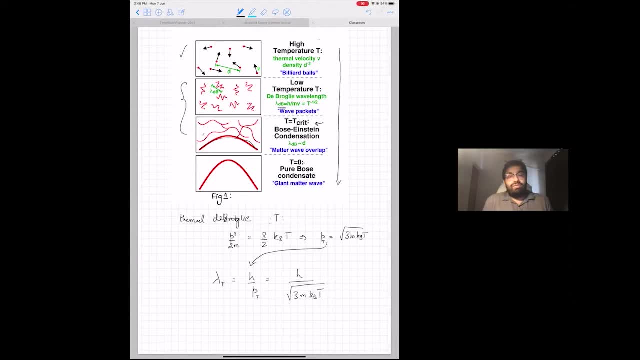 the state was originally proposed by Einstein in 1924-25, but the first Bose-Einstein condensate in a lab completely- uh, controlled manner it was made only in the 1990s. so it took very long, and the first sort of thing I want to emphasize is what is the hard. 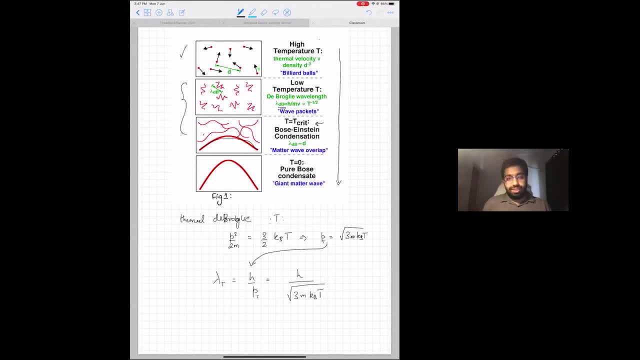 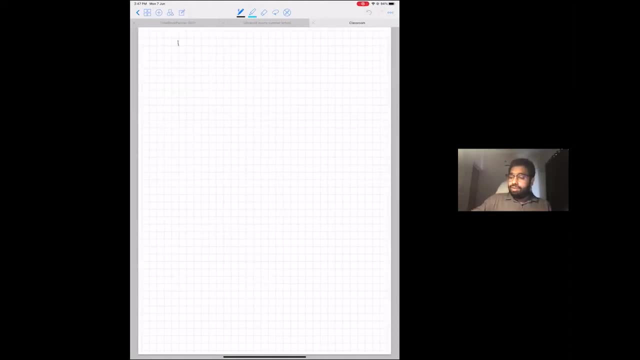 aspect of actually making and studying the Bose-Einstein condensate in the lab. okay, to do that, let's estimate. basically, let's just take air, our air, which is mostly made up of nitrogen, at room temperature and pressure, right. so at this room temperature and pressure, you can do this estimation. 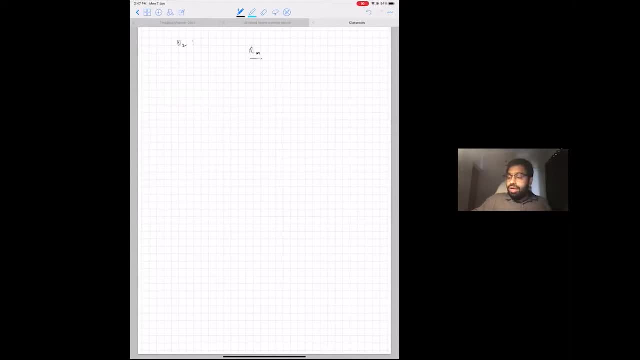 assuming roughly ideal gas behavior, the molar density. so the number of moles per unit volume is simply T over RT and after a little bit of work you can check. if you put in the standard room temperature and pressure you'll be able to see that this is about 40 moles per 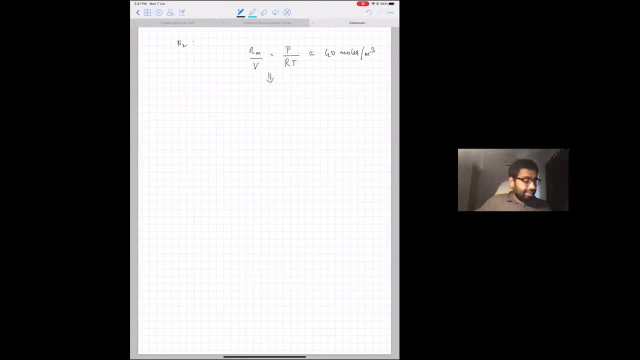 meter cube and if you actually looked at the particle density, so the number of particles per unit volume at room temperature of your nitrogen molecules is roughly of the order of 2.4 into 10 to the 19 per cc. just divide this by the average. 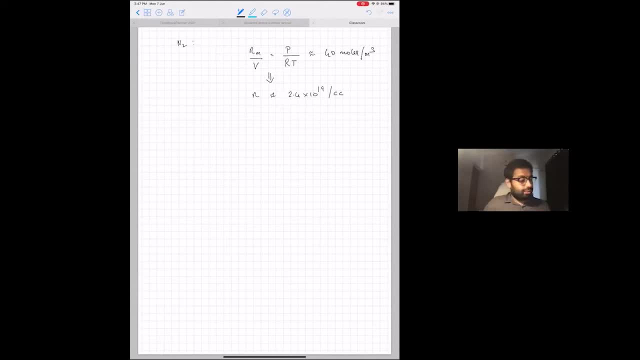 number of particles, number of Avogadro number. okay, so now, if this is the density, I can estimate the inter-particle spacing as, simply, if I take an inter-particle spacing of size D and take a volume of a sphere of size four by of this size D, the volume of that sphere is roughly going. 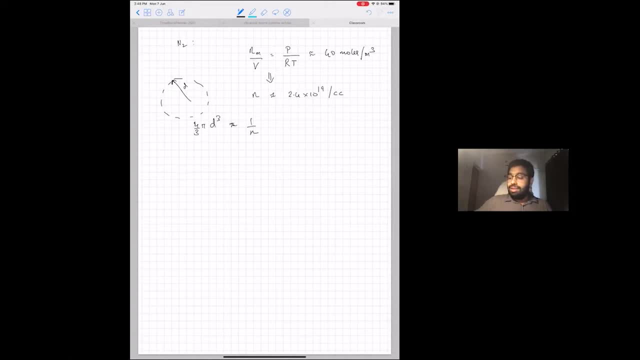 to go as one over the inter-particle density, right. so the inter-particle spacing is going to be set by the inter-particle density. so if this is one particle and this is another particle, so the rough in average inter-particle separation. I can simply get that by taking a sphere of volume D and 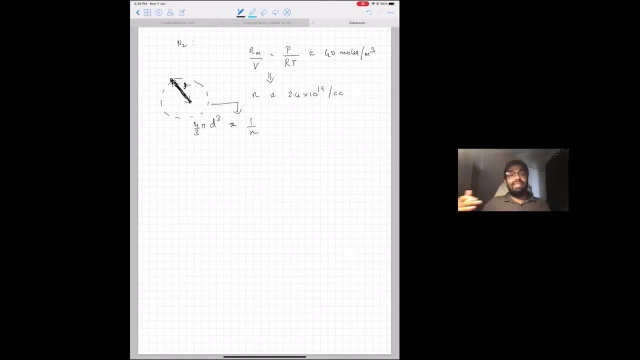 equating it to one over the density at that situation. okay, so, which means my inter-particle separation basically goes as the density to power minus one. okay, just inverting this relation. so now, if I look at room temperatures, I immediately see that for this nitrogen atom, for room temperatures, 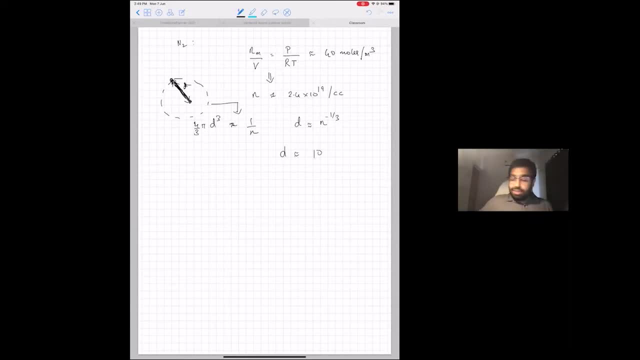 I basically have inter-particle separation of very large inter-particle separations of many meters, right? so I mean, of course, this assumes that I have such a large room. let's imagine for a moment. but main point is, this is over many, many meters. okay, so that's my inter-particle spacing at. 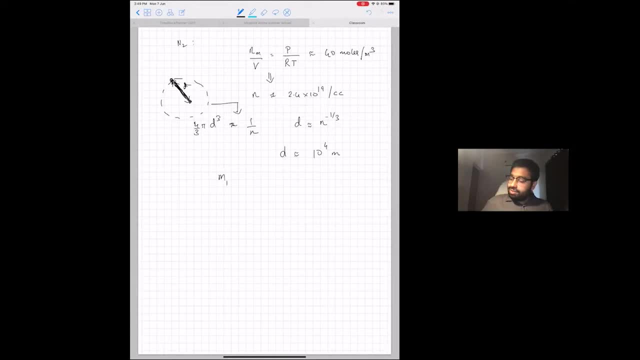 room temperature. now, if I basically take the mass of a nitrogen atom and then from that I can take the temperature, room temperature, and I calculate my thermal de Broglie wavelength, one sees immediately again after some algebra, that this is really really tiny. so it's of the order of 10 to 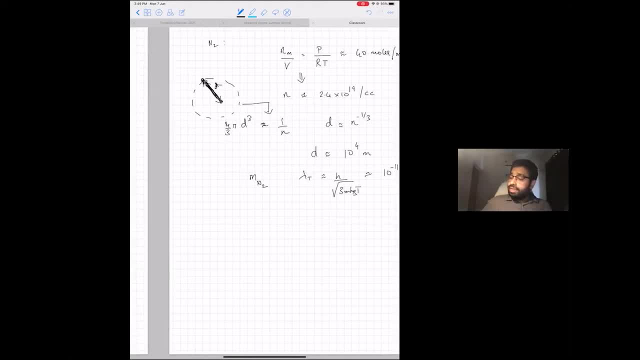 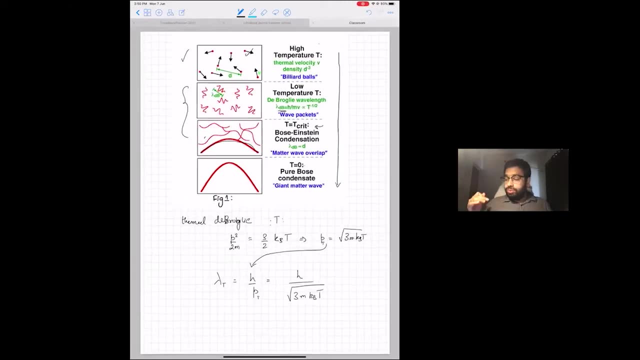 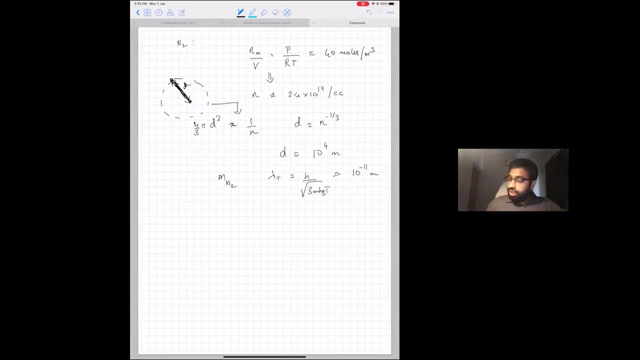 11 meters. okay, so this really at room temperature, you can, this picture is completely valid. okay, now, what can we do? so now, if you want to see Bohr-Einstein condensation, as I mentioned, one has to keep lowering the temperature, right? so if you keep lowering the temperature, this de Broglie. 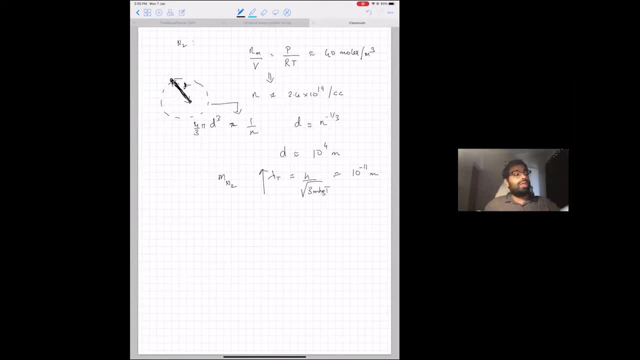 wavelength will start raising and at some point it's going to become comparable to D. okay, so now? how will you estimate what temperature scale will this happen? a very simple way to do that is to ask the following question: how many atoms can I fit in within a sphere of radius Lambda T, right? how many atoms are there? how many particles are? 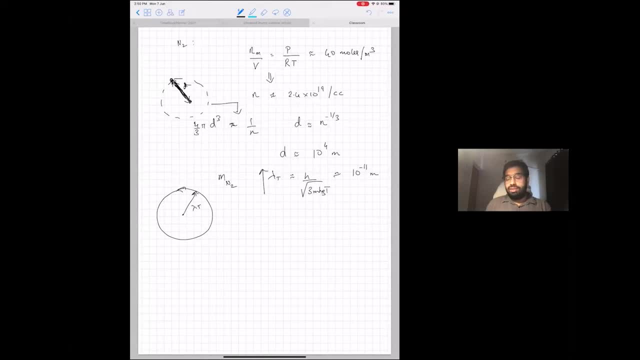 there within a sphere of volume, Lambda T. it's very simple: I just take the density and multiply it by Lambda T. okay, so now, in order for the de Broglie wavelength to be comparable to the atomic separations, I want this number to be less than or equal to one right. so only when, sorry, I want this to be greater than or equal to. 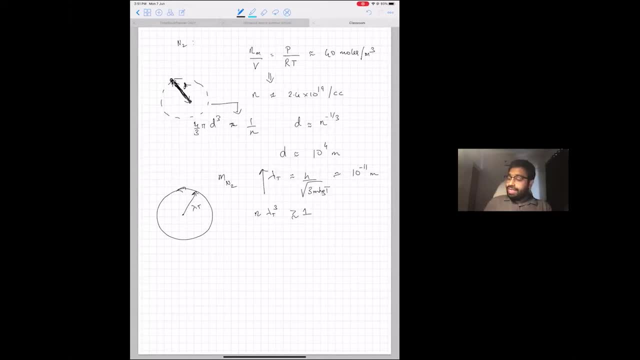 it. so the point when I actually have many atoms within this de Broglie wavelength cube, that is the point where I can start expecting this Bohr-Einstein condensate state to form okay. so this is a very, very important sort of back of the. 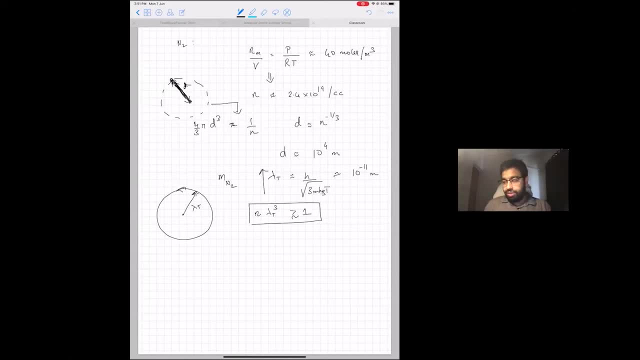 envelope number that will tell you whether you will have a Bohr-Einstein condensate or not if you take a bunch of atoms and try to lower their temperature. okay, so now we can do an estimate for the nitrogen atom things that we were looking at as to what should be this, at what temperature scale. 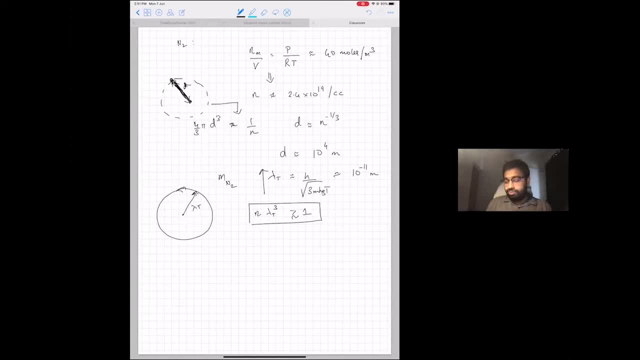 will you start seeing some effects of Bohr-Einstein condensate forming? so for that let's just say that n Lambda Tc cube equal to one. so once temperature is small enough such that n Lambda Tc cubes becomes equal to one, then there are at least many pairs of atoms with overlapping and de Broglie range. so, and you would expect from: 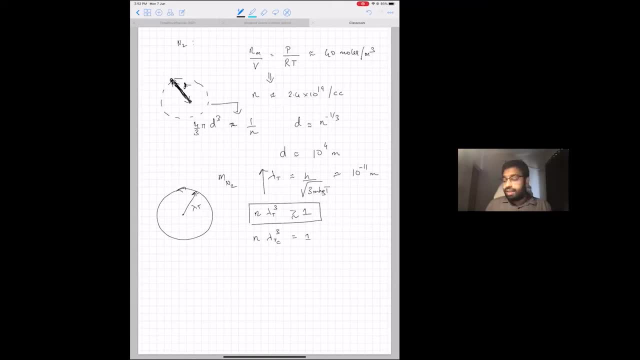 a very heuristic way that I've introduced Bohr-Einstein condensation so far. at this point we should see some interesting physics of Bohr-Einstein condensation happening. so if you take this and then you can then estimate basically Tc as n to the two by three. 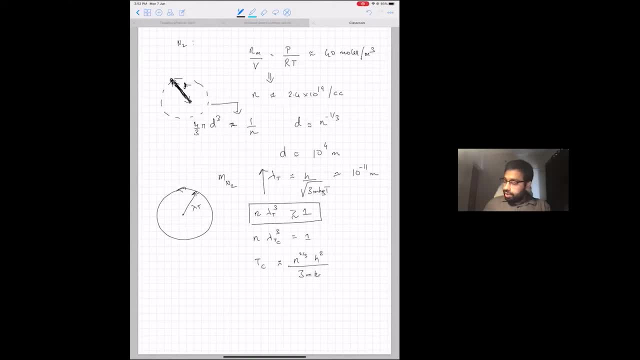 h squared by three mkb, and this once T is below this temperature, Tc, you would expect that you would have an Bose-Einstein condensate. okay, now what is the difficulty in reaching such temperatures? let's just do this estimate of what this should be for: basically, nitrogen atom. 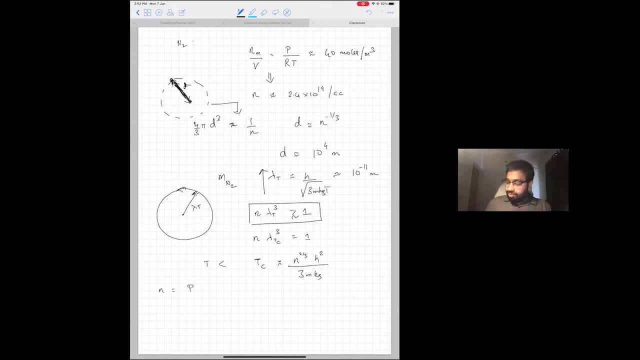 let's still pretend as though it is ideal gas, even at this temperature, and you can write the density in terms of the pressure and volume. let's still be in some standard room temperature and pressure and then you can basically plug in this density into this expression and one sees: 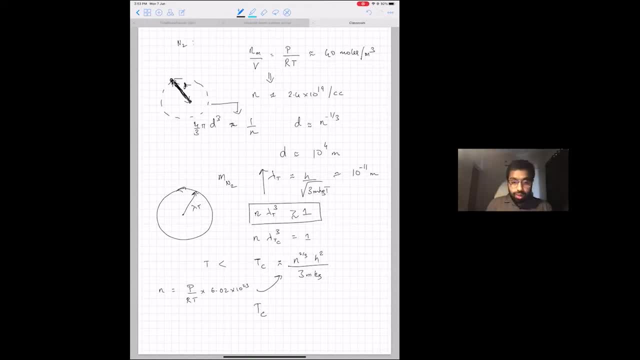 that for nitrogen atom at room pressure you, your Tc comes. so this is just some number. but to get a sense of why this number is difficult, one can ask a very interesting question, which is: what is the solidification temperature of nitrogen? that is actually quite high, that is a that's about a hundred trillion. 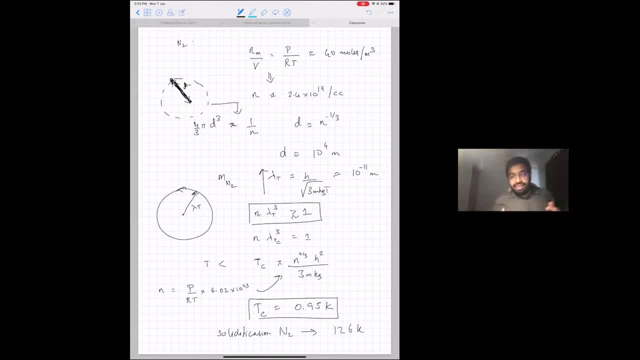 so what is this telling us? this is telling us something very important: that if you take most matter and start cooling it down, it will first solidify before it forms a Bose-Einstein condensate. what does it mean? it will solidify. remember that solidification of any matter is basically: 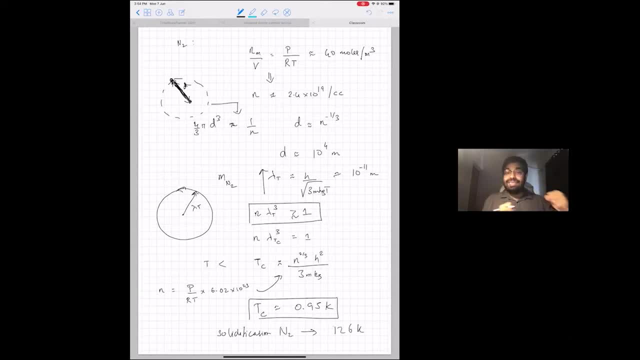 arising from the competition between interactions and entropy. basically, your map, your map, your collection of uh particles at some point refers to fix themselves and not be in a sort of liquid state to lower their entropy. So clearly what this is telling us is it is extremely hard to keep matter completely non-interacting as you keep lowering its. 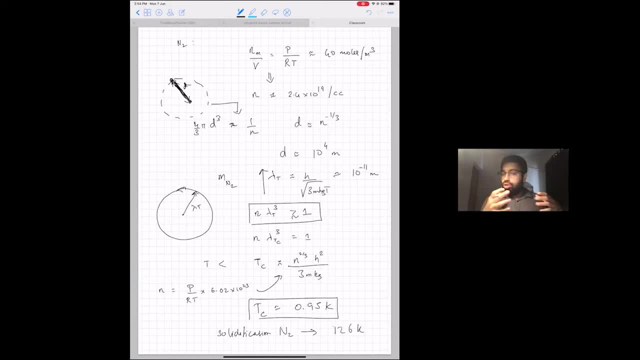 temperature. Most matter, regular matter, if you just look at lower and lower temperature. instead of forming a Bose-Einstein condensate, they are just going to solidify, So it's gas, liquid and then solid. This is why this concept of Bose-Einstein condensation. 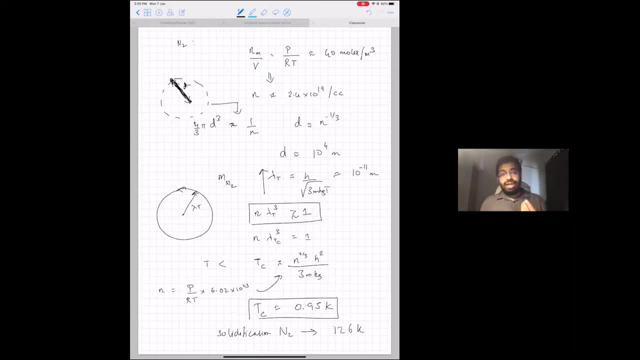 which was introduced originally for non-interacting particles or non-interacting bosons, was very hard to realize in practice. So you have to somehow engineer a condition where you lower the temperature but still continue to be as close as possible to a non-interacting limiter, And that's the challenge in making 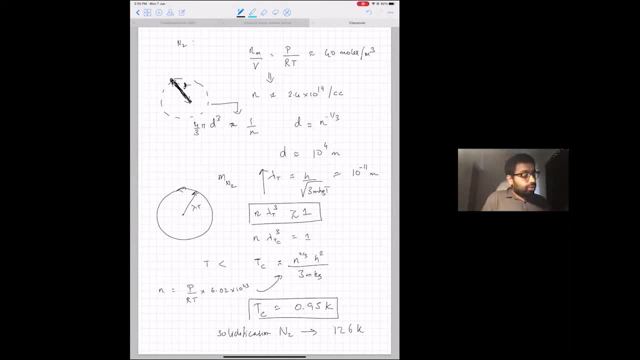 Bose-Einstein condensates. So with that, let me then say something else that is interesting. that happened in this quest for a Bose-Einstein condensate. So it was announced in 1920's and people were thinking of: how would you make one? 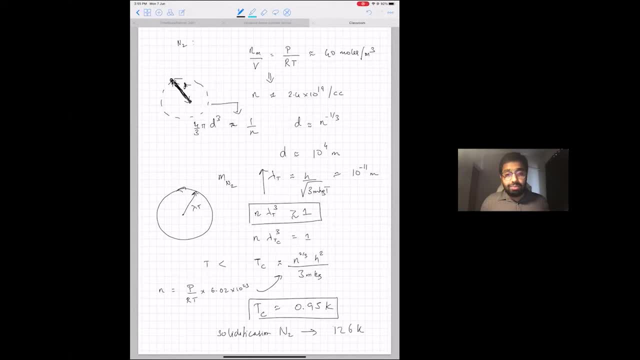 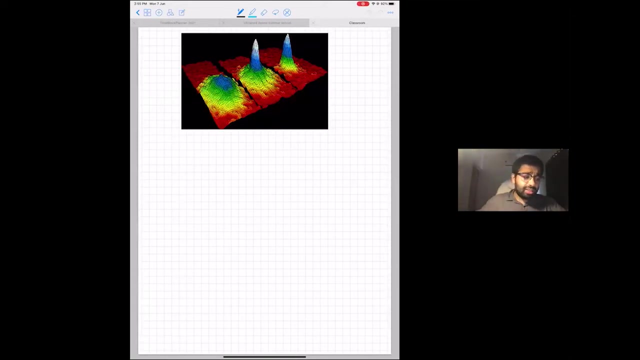 At that time, just this issue that you would solidify before you would ever pose condense meant that it was just a very theoretical thing, So it was not very clear how you would end up making a Bose-Einstein condensate. So in this context, a first clue: 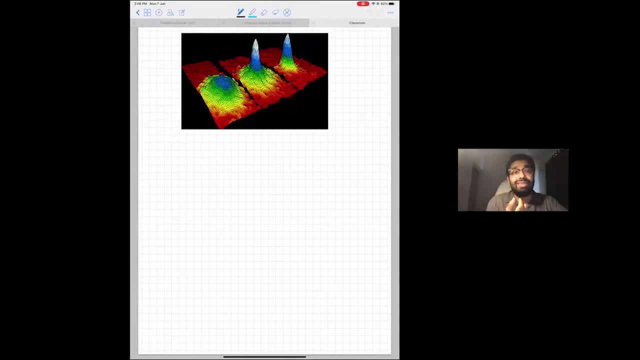 as to how you could make a Bose-Einstein condensate, or the fact that Bose-Einstein condensates could be really viable to be made in the lab, came when people were studying another very interesting set of collective phenomena of particles, basically in the study. of liquid helium. So what they found is that liquid helium, as you keep cooling it, cooling a sample of liquid helium below a certain temperature, which is called the lambda temperature, which is about of the order of 2 Kelvin. what happened is that this liquid helium stopped. 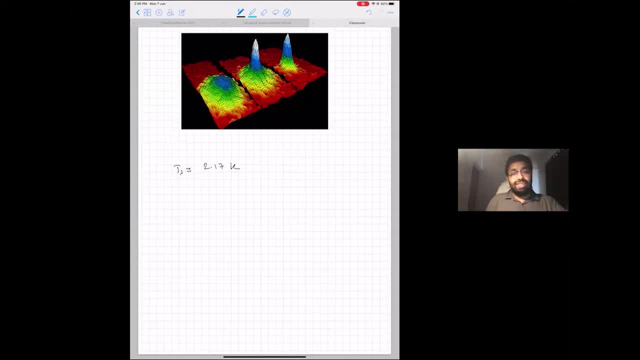 facing any resistance to flow. So basically, if you put this liquid helium in a capillary, it would flow Without any resistance. So this new resistance-free flow state of a liquid was called a superfluid, And this was puzzling people a long time. And at some point in 1938, along came Fritz. 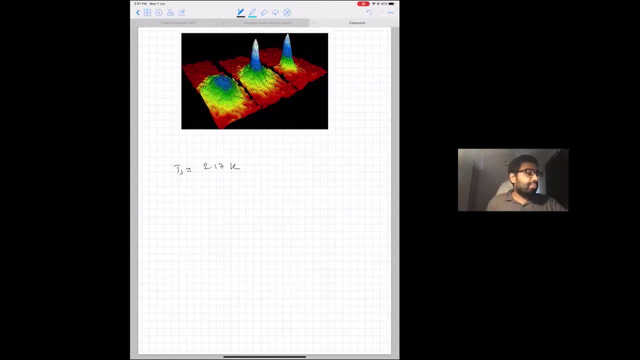 London who said there is an interesting connection between superfluidity and Bose-Einstein condensate and that at least part of the sample of liquid helium should have some Bose condensation And this can explain this frictionless flow. This was a very interesting clue, but there was a small problem. The problem is that liquid 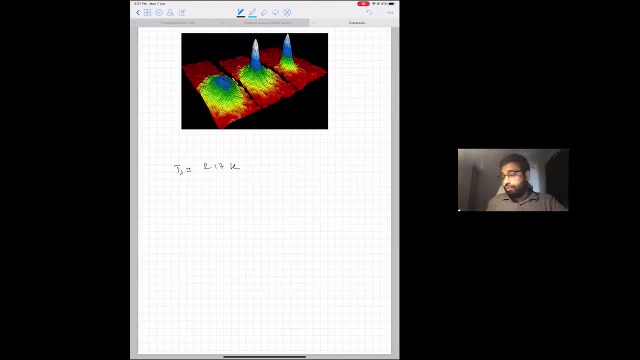 helium at the densities, that one In fact, if you want to see why this claim by Fritz London, which was made with a lot of theory, and it was quite an interesting suggestion, but it had some theoretical backing. but So, in the case of the formula, what you can do is you can just plug in into this expression: 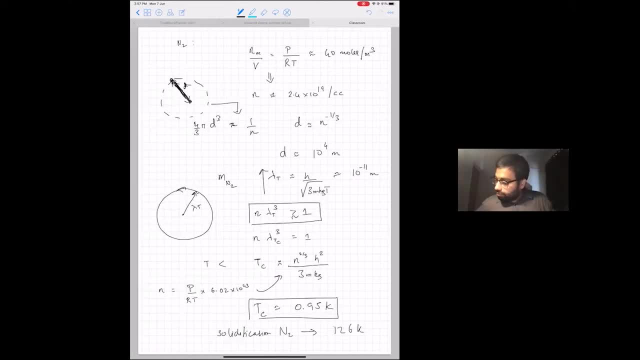 I have for TC in terms of the density. Yes, into this. if you plug in mass of liquid helium and the density of liquid helium, when it makes just the regular density of liquid helium, you see that this DC comes to about 3 Kelvin. So this is a very tantalizing suggestion because 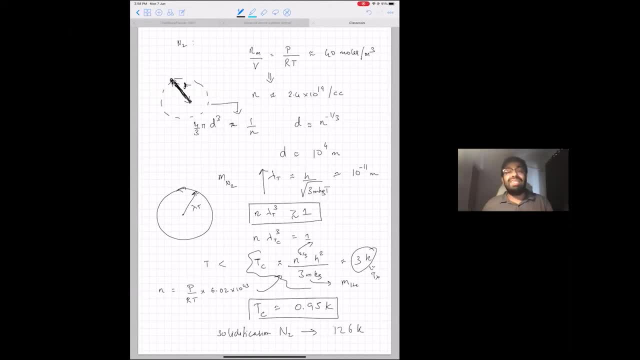 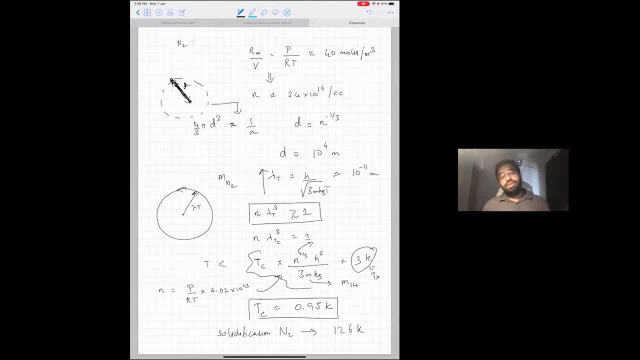 But what is the catch? The catch is that liquid helium is very strongly interacting, even though- And that is the very interesting part of liquid helium- that, even though it's very strongly interacting, instead of just solidifying it continues to be a liquid. Not only that, it. 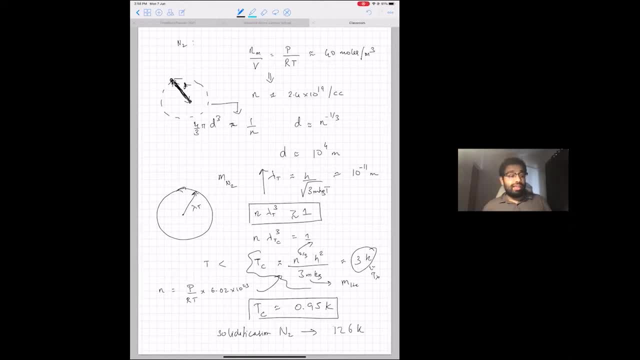 becomes a super fluid, And this told the community that, well, you could have Bose Einstein condensation, but you can't have Bose Einstein condensation, So you can't have Bose Einstein condensation, So you can't have Bose Einstein condensation. 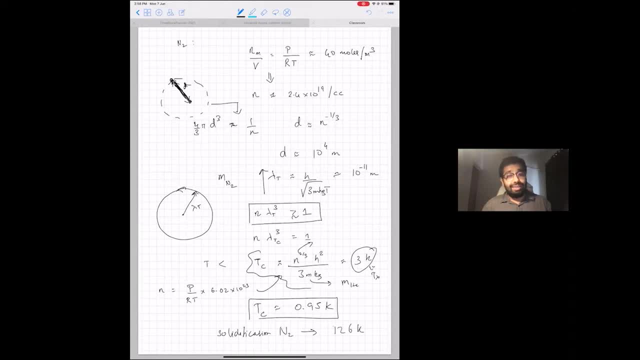 So you can't have Bose Einstein condensation. You should not restrict those to interactions. You have to understand how these go to base into Bose Einstein cond menstruation. We will get into some of this aspect at the end if there is some time left. 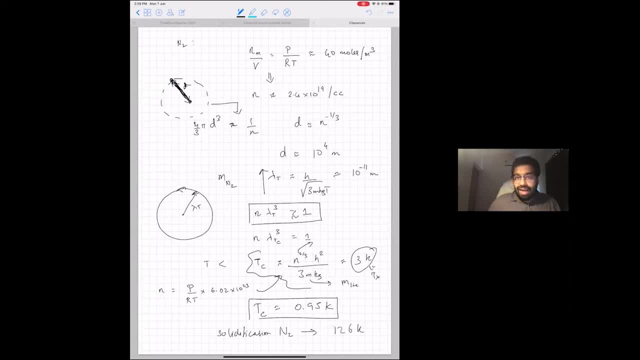 But the combination of this original non interacting suggestion and the original prediction using non interacting bosons and these possibilities that is suggested by this liquid helium therefore meant that bunch of people said heroically that we should really try and make a BEC with weakly interacting 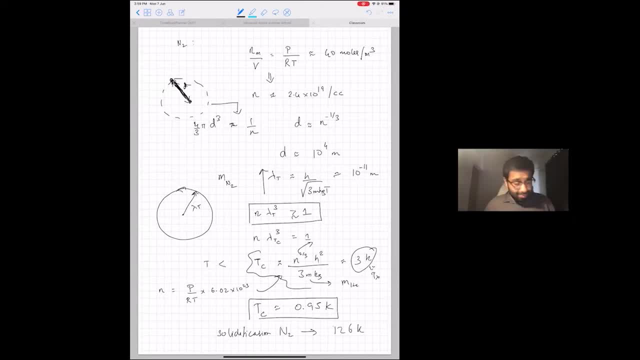 diode gases of atoms. right, so if i keep making my density small, i can be as far as i want from solidification. okay, but what is the price i pay? of course, there is a small thing that you can do. you want to make your density small and you also want to choose particles of as small a 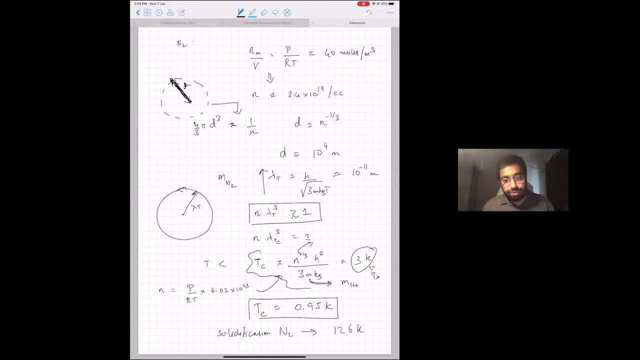 mass as possible. of course, one of the first things that people tried was to make a boson condensate with hydrogen, and it was eventually done. but the first bosion condensate was not made with hydrogen for some slightly more technical reasons. but the key idea is that i want to ensure 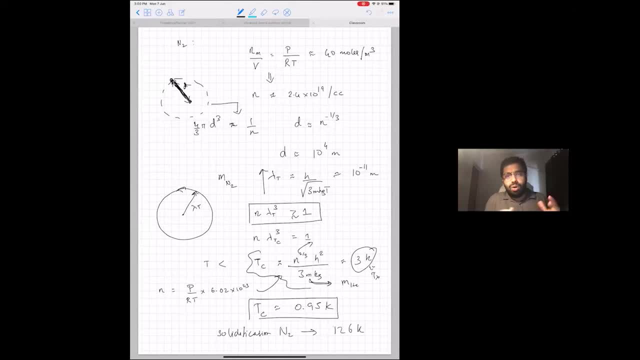 that i can make a collection of bosonic atoms- our atoms, goes on it, by the way, because they are made up of fermions and they are made up of even number of fermions. atoms are made up of even number of fermions. bosonic statistics. We just wanted to put that out there. So now, what did they want to do? They? 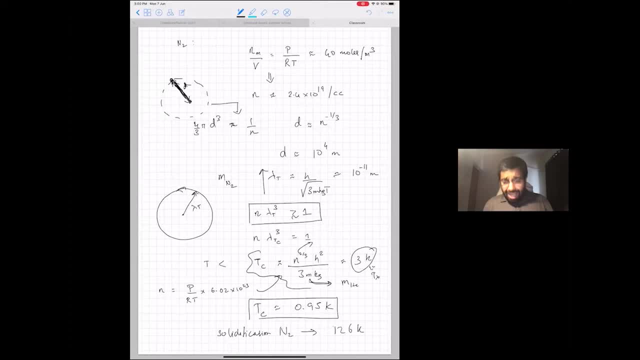 want to keep the density as small as possible and still try and make a Bose-Einstein condensate. If the density is small, you will not get solidification, but on the other hand, this expression already tells us what is the major challenge. then, If you keep the density really. 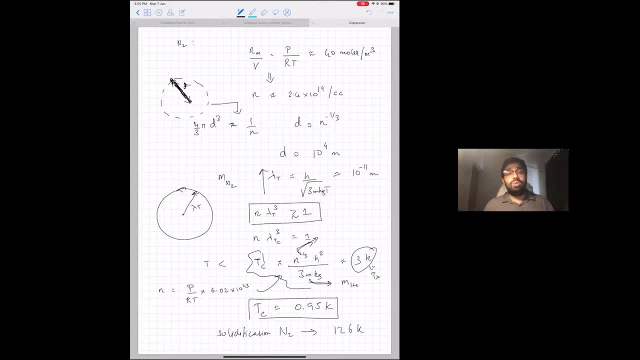 small your temperature. Tc, at which you will start seeing Bose-Einstein condensation, is going to go even lower. In fact, how low does it go? Hundreds of nano Kelvin. So, which meant people have to figure out how do you take regular atoms and regular matter and cool it? 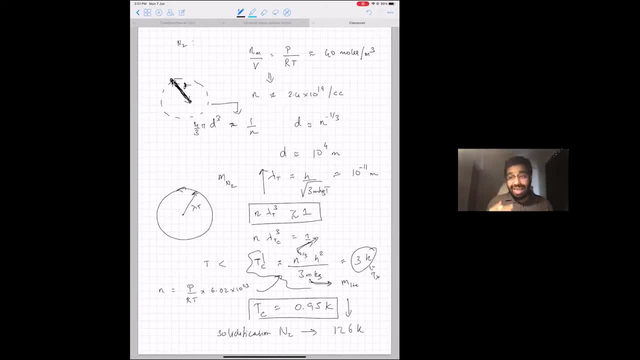 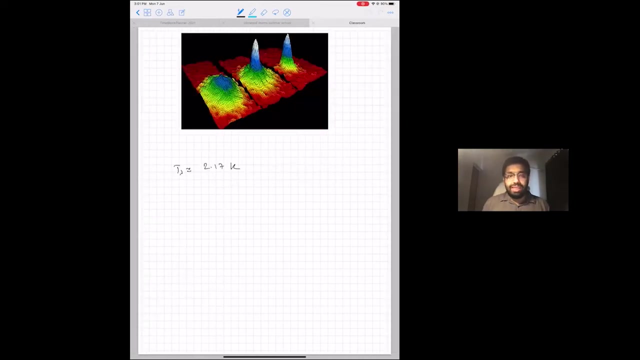 to hundreds of nano Kelvin, which is roughly about 10 orders of magnitude from room temperature. How do you do that? Which meant you have to understand how to cool atoms first, and in this manner I'll talk a little bit about this cooling in eventually. 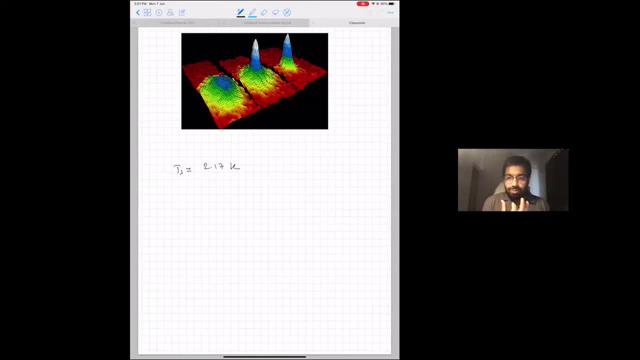 So, but basic elements of this cooling. let me just put out these words there and we'll tackle one by one. The idea is that I've been now talking about very simple bosonic point particles. Of course, atoms have internal levels and these internal levels are usually, in many atoms, split by some. 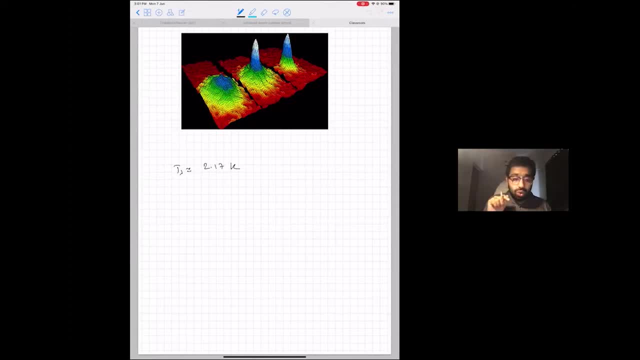 optical tracings. So these are the internal levels, and these internal levels are usually in many atoms split by some optical tracings. So you can see the この Z-man effect. if you have learned an atomic physics, you can exploit that to create the. 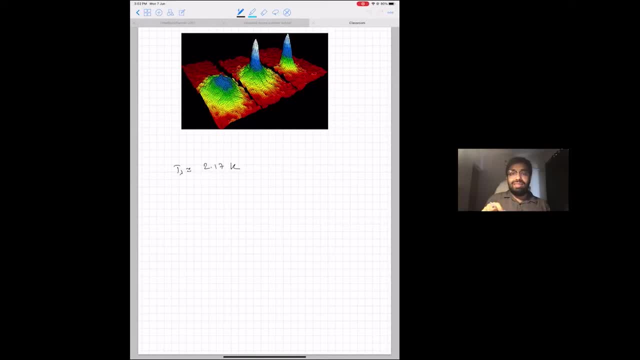 configurations of magnetic fields in space which are preferable for atoms to occupy, or in other words, you can trap them by using magnetic fields. and finally, the last thing that one needs to do after cooling atoms with lasers and putting them into magnetic traps, is a very, very, very 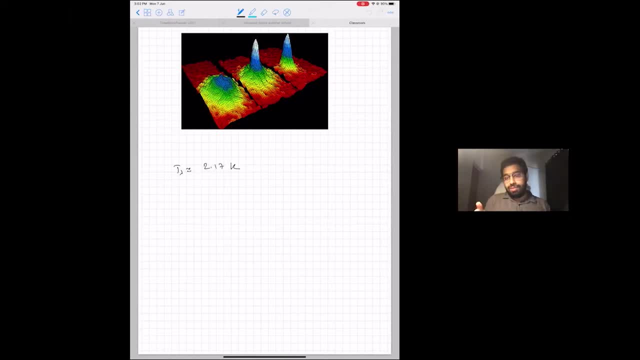 old idea of how cooling works. for example, if this is summer in India, you might have a earthen pot at home. how do you make cold water in earthen pots? the idea of evaporative cooling, where you let very energetic particles in your sample to leave and whatever is left is going to. 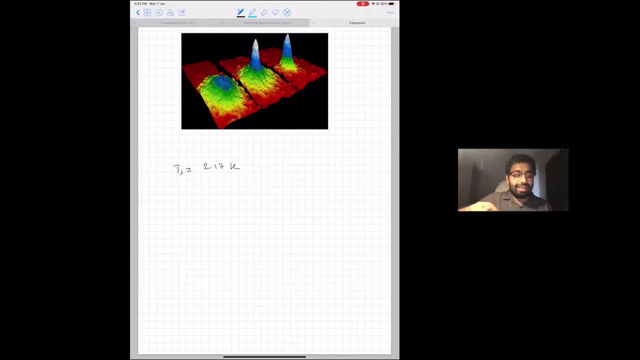 naturally be at lower temperature. and just after this last step of evaporative cooling, I realized that I summarized in like one minute basically experimental and theoretical advances of cooling that took order of 20-25 years. So I mean, we will get a little bit into it later, but the idea is that you one was able to do that. 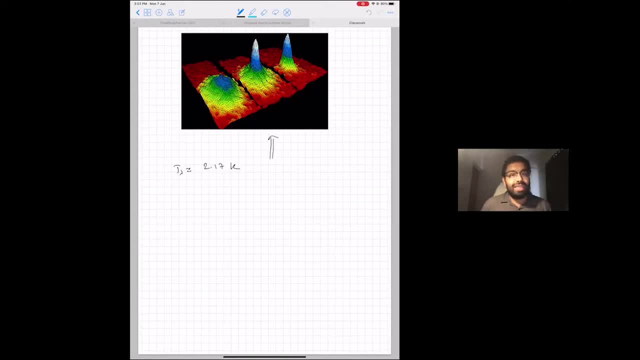 and this picture that you see finally here, which you might have seen many times, shows how in 1995, after doing these different stages of cooling, the first cosine-stein condensate of rubidium atoms was achieved by Tal Griemann and Eric Cornell, and then later with rubidium atoms. these are 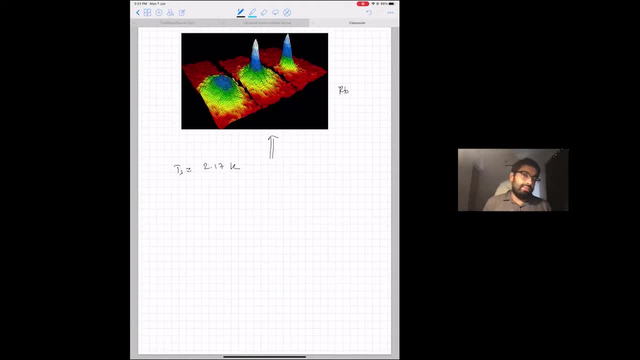 the rubidium atoms And eventually with sodium atoms by Wilke and Ketterle. We will unpack what exactly is this picture? one of the things we will do today is unpack what is this picture and what this is showing. rough, just as a trailer. what this is showing is basically the. 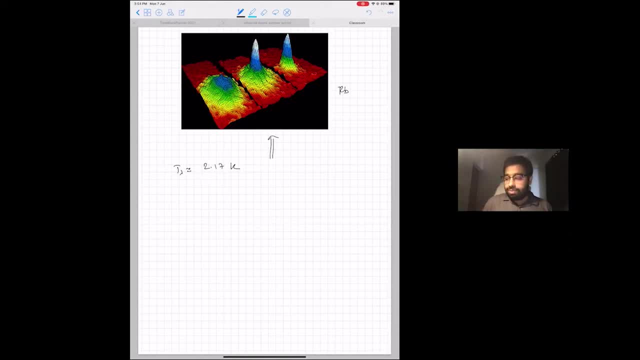 momentum distribution of a trapped cloud of atoms and as you go from left to right you're lowering temperature and in the left corner it is still a thermal gas with some Maxwell Boltzmann distribution and eventually the momentum distribution becomes very anisotropic. and this is literally the ground state wave function of an harmonic oscillator in 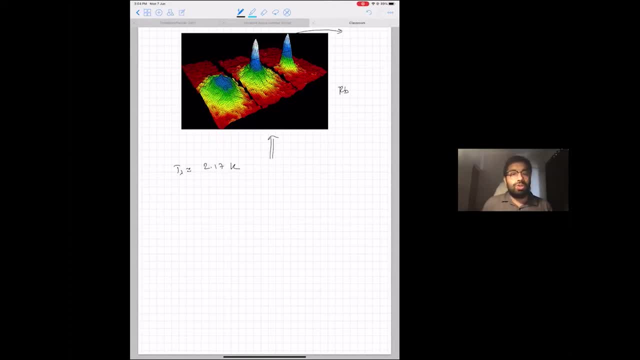 momentum space. This density distribution corresponds to that and it shows that all of the atoms have gone into the ground state of this graph. okay, and the last thing I'll say before I take some questions is basically, the density of this graph is the density of this graph. is the density of this graph? 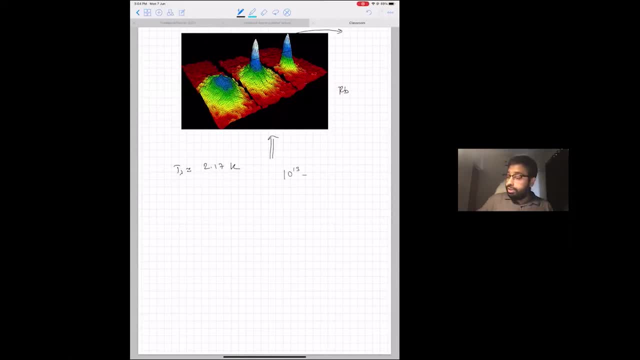 The density of these cloud of atoms is about 10 to the 13 to 10 to the 15 per cc. you see, that's like four to six orders of magnitude less than as that we have been doing right now. so it is really low density and that is why things don't solidify and, at the end of the day, the aim of these lectures is: 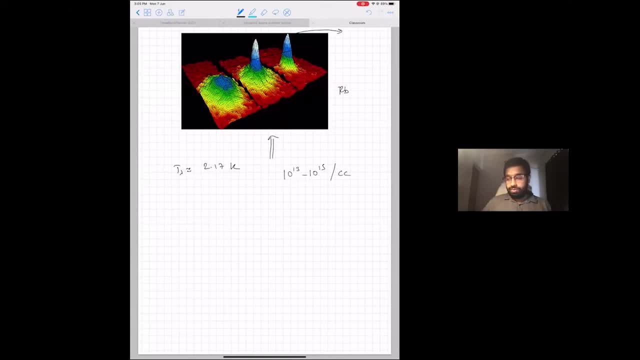 to develop a theoretical understanding of some of the fascinating properties of these Bose-Eickson condensates. how to describe them and how, how? what can you do with them? So let me take a quick break here and answer some questions, if okay. so there are. 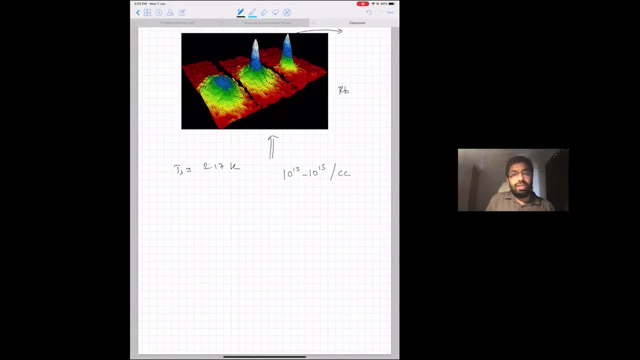 at least a bunch of questions here. let me begin by looking at the chat and, unless someone has a immediate question that they want to unmute themselves to ask, Okay, so while people consider unmuting themselves, let me just read. so there is a question from Swagata which asks: explain once more why you equated one over the. 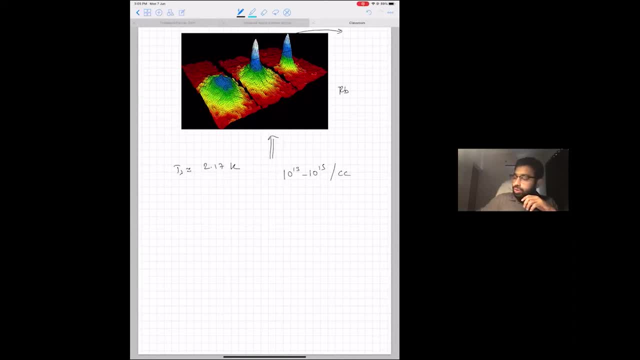 particle density with four by three, by dq. so all that I'm saying there is, if I have a collection of atoms in some volume, if I have a separation, if I have a density of n, then on an average the separation is going to be such that if I draw a sphere of 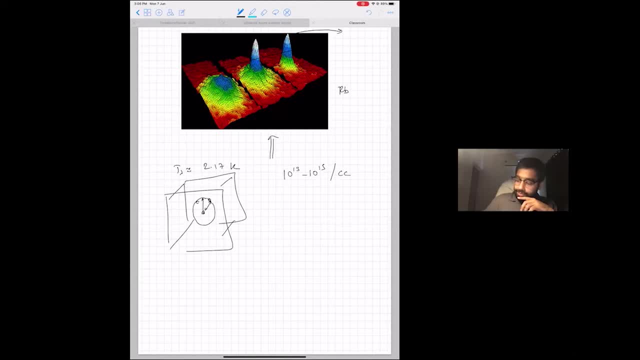 radius d around a particular atom. right, then this will give me, if d is the inter-particle separation, and I calculate the volume of this. this is going to be of the order of n over d. right, sorry, this is going to be of the order of the total volume over the number of particles. 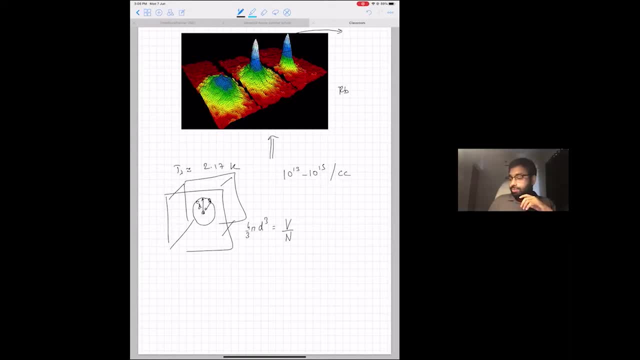 right, because that is precisely the definition of the inter-particle space. so I will not find one more particle within this volume. that is my inter-particle separation right, or at best I find one particle within this volume. so this volume over n is the specific volume that is allowed for each. 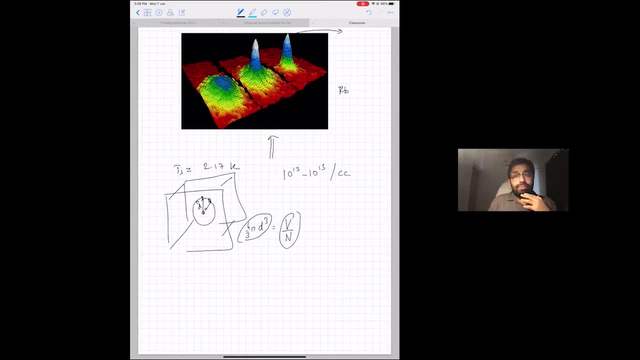 particle. so that's the idea. okay, then the next question is: can we find Bose-Einstein? No, Okay, Yeah, I'm Swagata, Yeah, Yeah, yeah, I understood your point. and I had one more question about your comment that in a Bose-Einstein condensate the wave function gets. 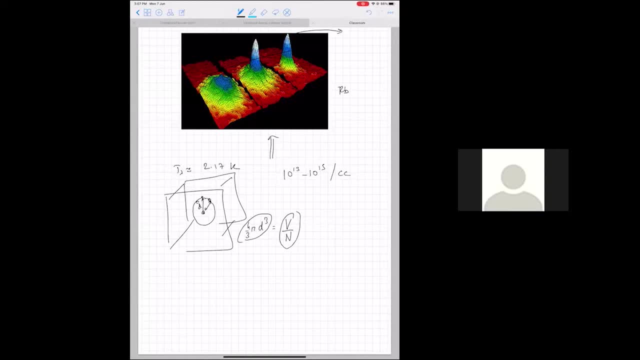 is the total wave function of a group, many number of particles. so the advantage is that the different hidden, non-intuitive quantum aspects get amplified. so can you please elaborate on that? Okay, so let's see what is the best way to elaborate. Okay, so one example let me. let me just give you one example of what happens with such things. so 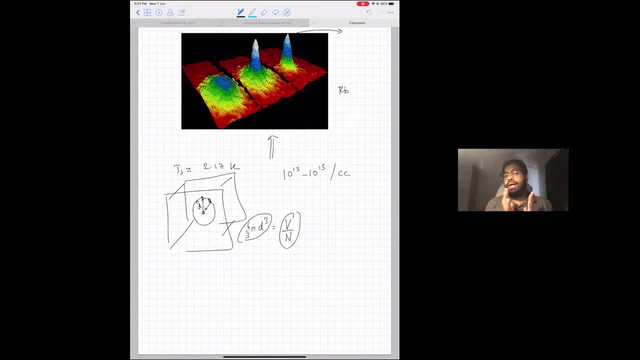 what is the best example of okay, so I can actually take a Bose-Einstein condensate okay and apply a potential on it. so this is like a part. this is a bunch of particles. I can apply some potential so I can make very interesting potentials. one very interesting potential I can do is I can. 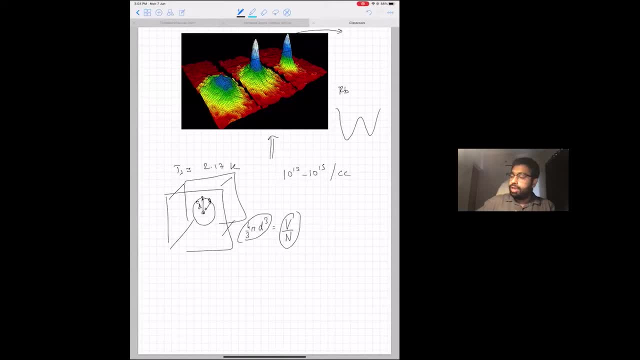 take a Bose-Einstein condensate and put it in a double well. okay, so there's a double well potential. this is just v with two minima. okay. and I can actually trap a Bose-Einstein condensate, not in just a harmonic oscillator like is being done here, but I can put it in two wells. and now what I? 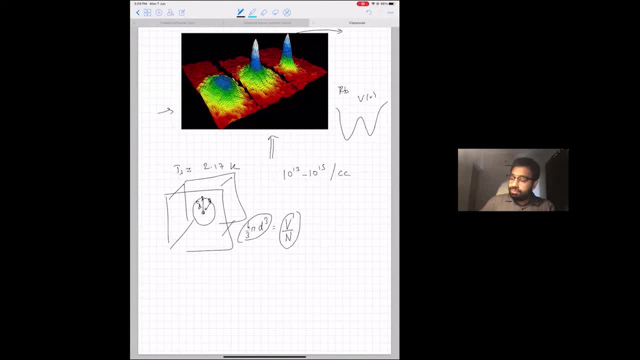 can do is I can start with a Bose-Einstein condensate with this barrier, very small, and slowly raise a barrier- okay and very interestingly such- and I can trap millions of atoms- okay, 10 to the 6 atoms- in such potentials. and by raising this barrier I can really go. 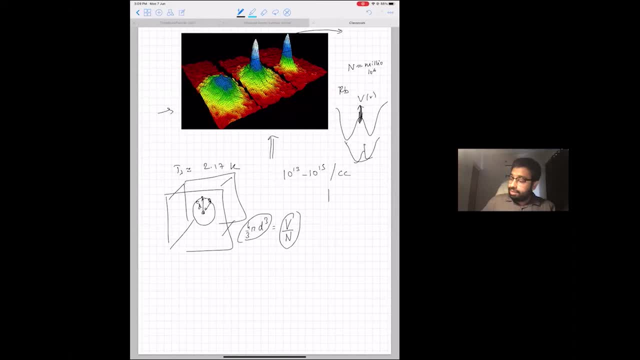 after a point I can go into a state like: so, where there are n atoms on the left, well, zero atoms in the right, well, zero atoms in the left. well, n atoms in the right, well, okay, one over square. so this kind of a state if you are, if you've been, if you've looked a little bit at quantum mechanics. 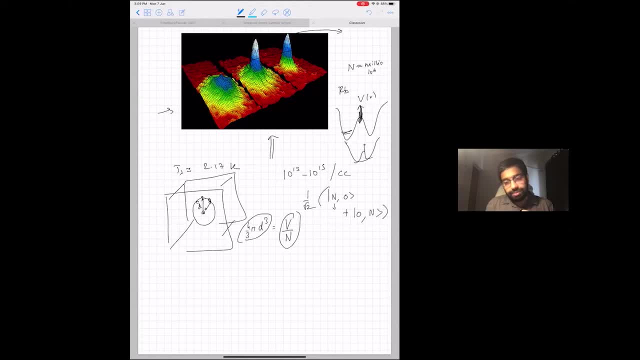 this is a very, very, very interesting quantum state. right, this is basically a superposition of two very distinct macroscopic states. okay, this is no big deal with an electron if you can make a special superposition of a single electron. that happens all the time when the electron is occupying some orbital in your hydrogen atom. but what this is is. this is: 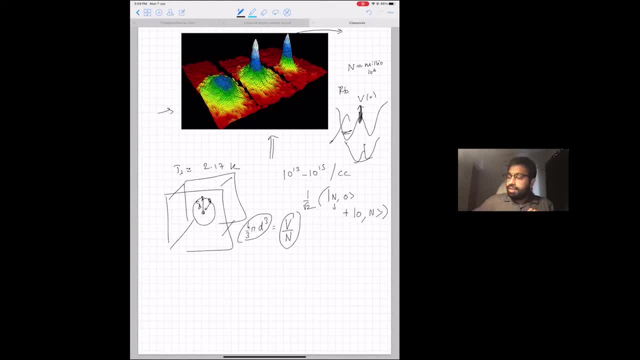 really a very strange spatial superposition of a million atoms, okay, and this is sometimes called a, a version of what's called the schrodinger cat state, because clearly these are macroscopic potentials that i'm applying, so this would be of the order of microns. this is very large length. 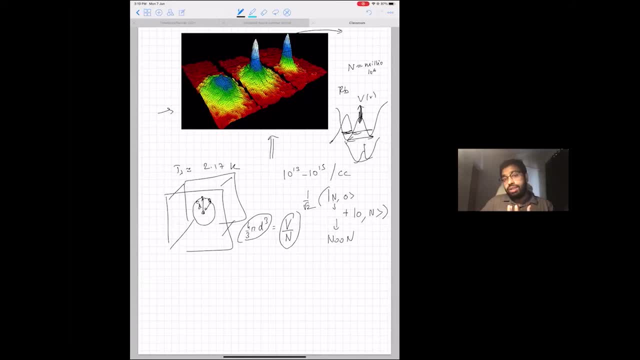 scales and i'm delocalizing a large quantum wave in this manner. right, so i'm amplifying a very simple thing that i know works very well. spatial superpositions of small quantum particles works great, but i can do it with a million atoms with the boson stand: condensate. then you can start. 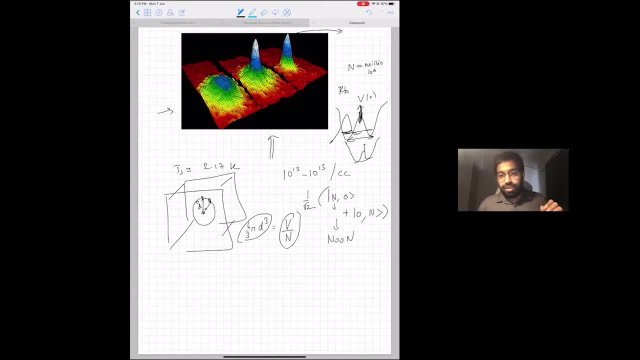 asking questions like- which is one of the questions that someone asked- can we find such superpositions in nature and why do we not find such superpositions in nature? such questions can be addressed by pushing quantum mechanics and quantum effects to larger scales. i don't know if i answered you. yeah, yeah, thank you. thank you very much. i just wanted to pick one, okay, uh. 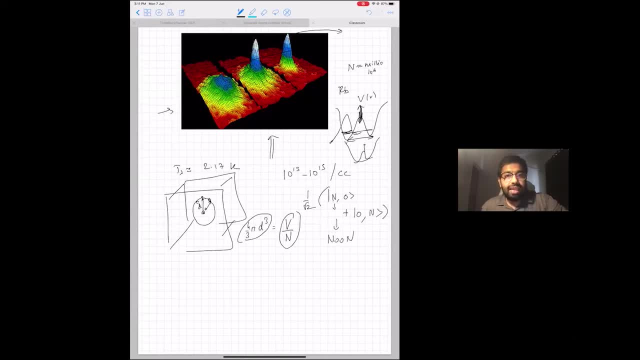 so let me quickly take a couple of questions and then come back. can we find uh boson string condensates in nature? as i said, uh, not very naturally. you have to cool matter down to very low temperatures, of course, and and you should have enough, um, the density shouldn't be zero. 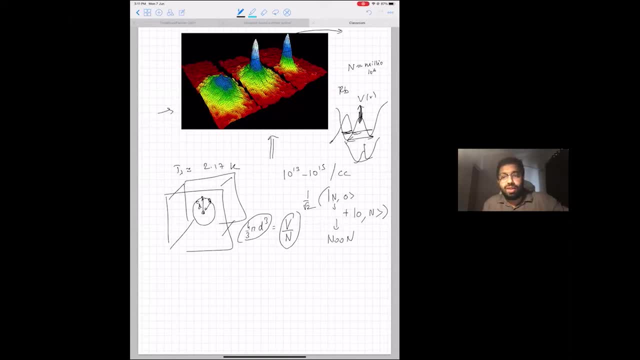 because you can ask: uh, go to space, there is. there are no particles, the density is essentially vacuum, so then you can of course not have a bc there too. so it's, it's definitely an engineered thing. the closest to a natural boson stand condensate you can find. 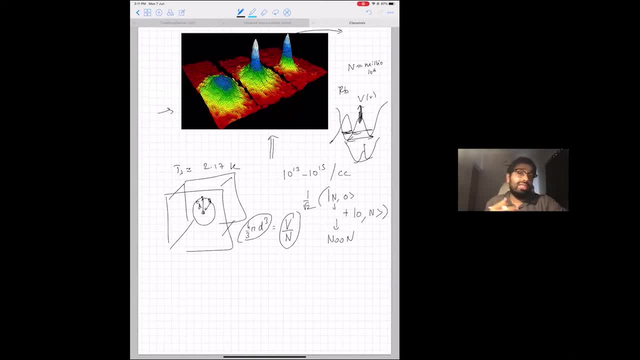 is this super fluid, and in some sense you can think of superconductors, also in terms of a boson stand condensate, but that's a story for later. okay, uh, good. so then there is uh, another question, which is uh. when you said we can exploit zeman effect for cooling, do we essentially make 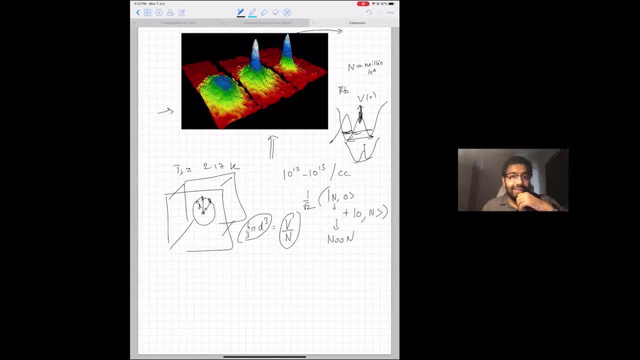 magnetic traps which keep the zeman effect for cooling, or do we essentially make magnetic traps which keep the zeman effect for cooling? do we essentially make magnetic traps which keep the, the atoms, far enough? um, i think i just meant magnetic traps. of course, the density of the atoms in the magnetic traps, that will depend upon how much. 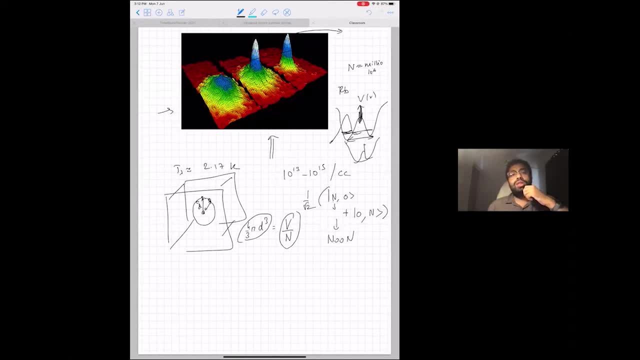 atoms you started with. what is the efficiency of your trapping and so on? okay, then how does entropy change as gas goes to a cosine stand condensate, okay. so i think this is somewhat of a very detailed question. i will address not the entropy change, as you have a bc. 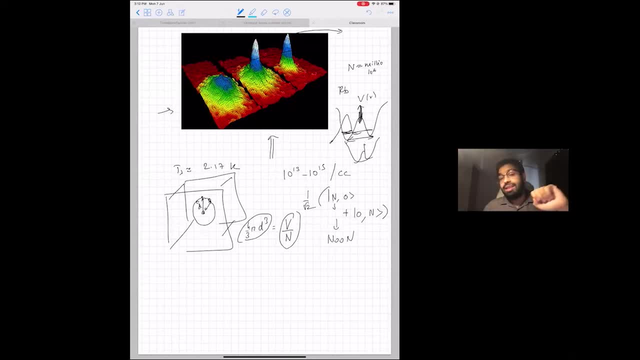 transition, but another thermodynamic absorber, which is the uh, the specific heat um i i will i'll point to references where you can actually see how the entropy changes. so there is a non-analyticity in uh thermodynamic variables. as you go through the 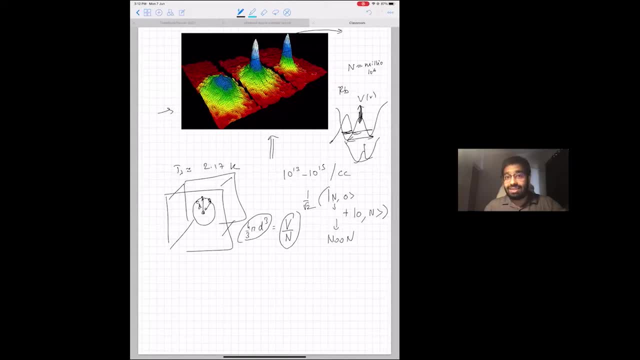 bc phase bc transition and that's why it's a phase transition. but the non-analyticity we'll see depends very uh markedly on what density of states you have for your sydney trap. so very soon saying we get markingesteven, or in the last second here, like straight around, what is the density ofcorrected? 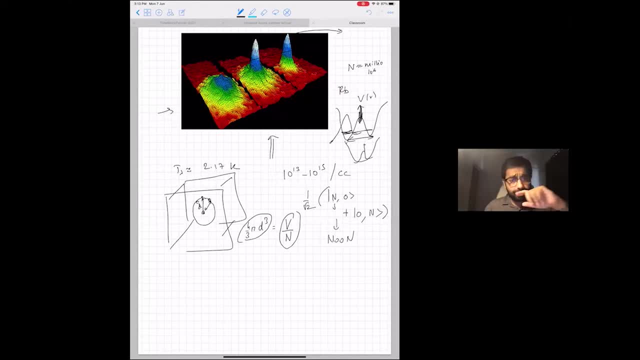 density of states, you'll see, depends very uh markedly on what density of states you have for your sydney trap, you have for your single particle protection. So now I think the other question is: can you explain once more the non-interacting idea for Bose-Einstein condensate? 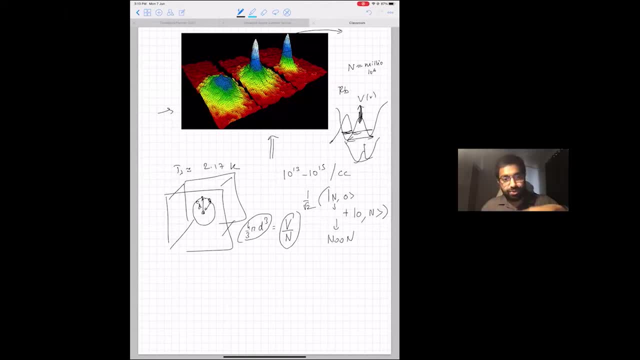 We are going to go into it in very gory details next. So that's good. Can we see Bose-Einstein condensate for photons in nature? That's a very interesting question. Yes, there are two things. One is in some limit. one can very, very, very loosely. 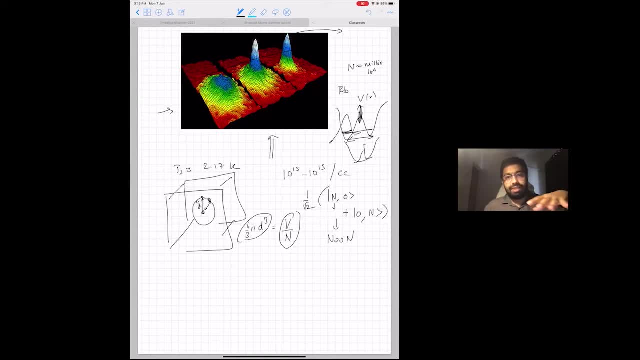 make an analogy between lasers and Bose-Einstein condensates. That is one way in which one can talk about photons and Bose-Einstein condensate. But really, if you look for photonic disease in literature, the thing that people are thinking about- 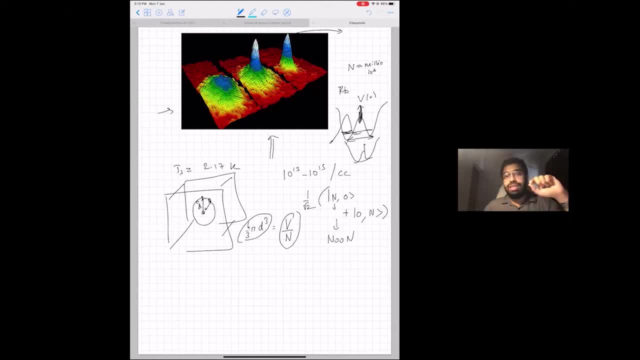 are certain systems where you can introduce effective interactions between photons. That is more similar to what happens in these atomic systems. These will have interactions, as we will see. So in those cases you can also see a Bose-Einstein condensation of photons. 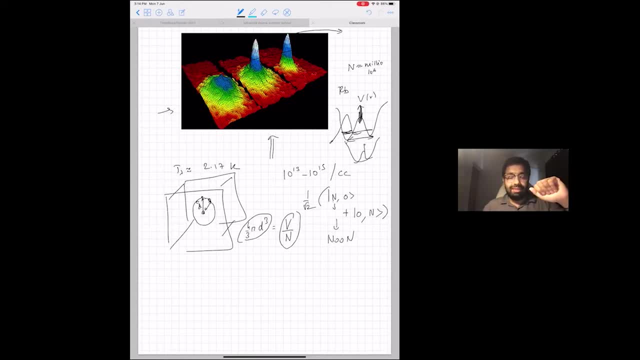 So it is possible to do, But that is for you have to have a very special kind of system where you can introduce interactions between photons, And so this is not very- it's not in the sense of it's not exactly like a photon gas. 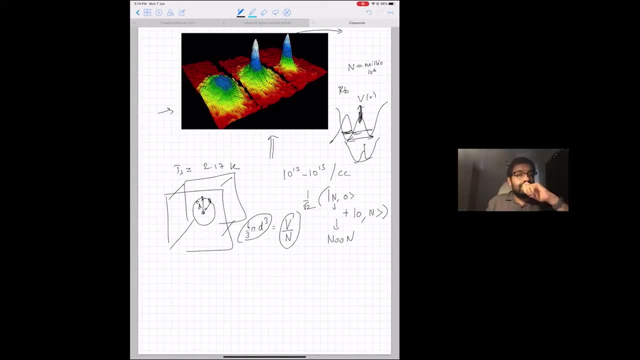 OK, All right, So I think I've taken a few questions, If there are, I think. since it's almost again 3.14,, I move on now, Let's. I'll come back for more questions later, OK, Good? 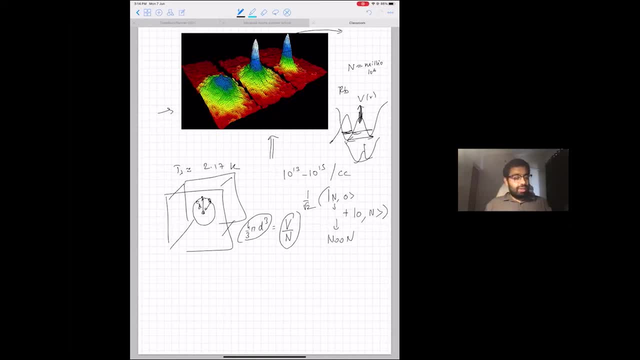 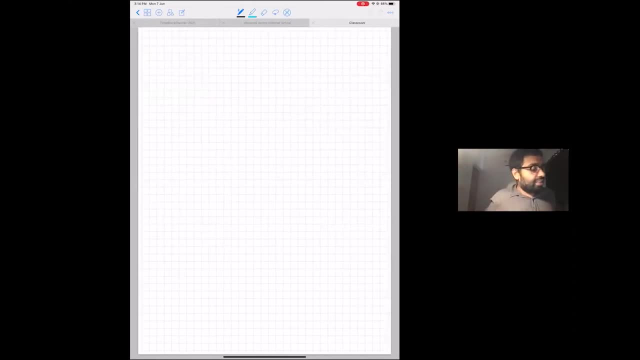 So we've answered a bunch of these questions, So now let me, before I go on to answering the next part, so finish off this introduction. let me just finish Bye Bye, I guess. OK, So I'm going to just end it by saying what. 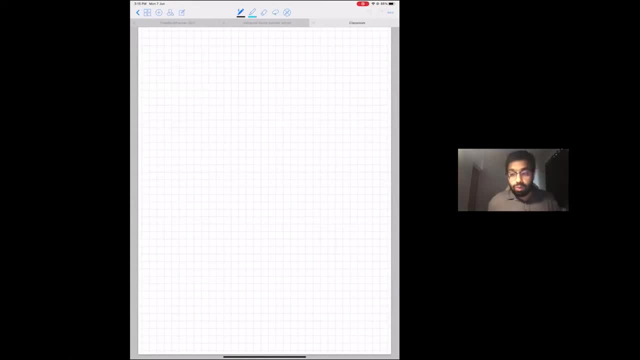 is really interesting about VCs. I already answered a part of it, which is to Swagata's question. I said these are macroscopic quantum systems and you amplify quantum effects. I gave an example of that already, And so this will help you understand fundamental aspects. 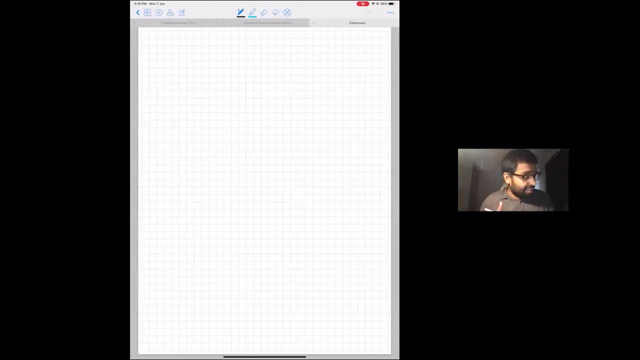 of quantum mechanics? Why do we not find naturally occurring Schrodinger-Pat states And such questions? quantum effects is we've known to understand now that we can make extremely good sensors with quantum systems, and so you can use Bose Einstein condensates to sense very small physical quantities. 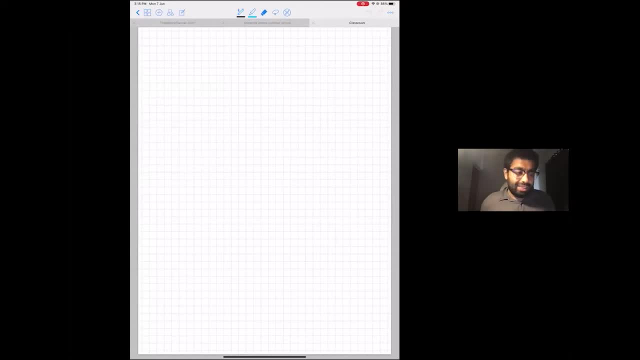 okay, so that's a very sort of applied reason why it is interesting. then, something a little bit more fundamental that you can do with Bose Einstein condensates is that with these Bose Einstein condensates of atoms, species of atoms, cold atoms, you get extreme control over every aspect of this. 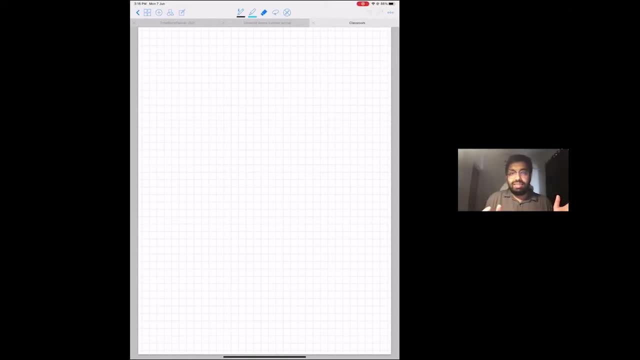 system that you make in the lab. this is not like liquid helium, where you just take liquid helium and just cool it down in a devar. this is really state-of-the-art quantum optics, state-of-the-art atomic physics- which I will briefly describe later- where you can control everything you can. 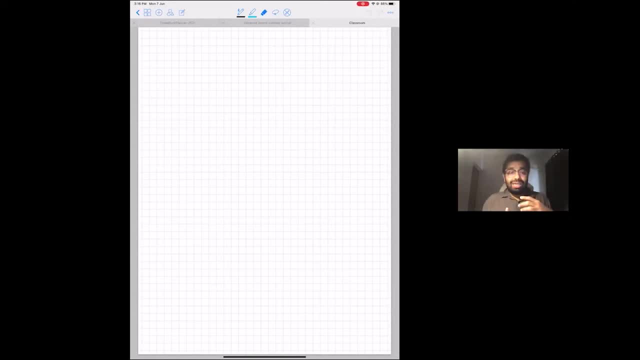 control the strength of the interactions between the atoms, you can control the effective dimensionality. so because I can make traps of different sizes and shapes, that's again. I can go from effectively 3d to sorry 3d to effectively 2d to effectively 1d, study very different dimensions. then I can also put very interesting. 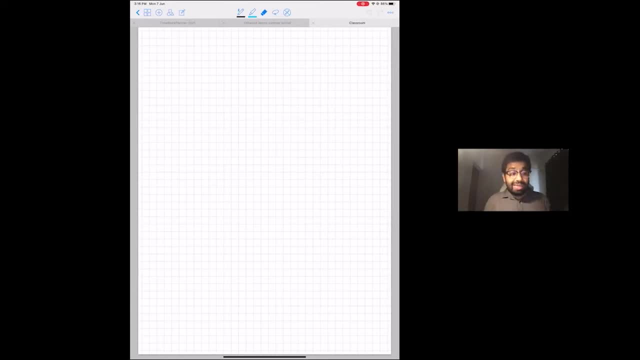 external potentials, one that I just talked about, a double well, or you can even put another potential, that is, periodic potential, which is called an optical lattice, which you'll get to in the final lecture. and what? what one can achieve by doing this control is that, at the end of the day, this system is really a 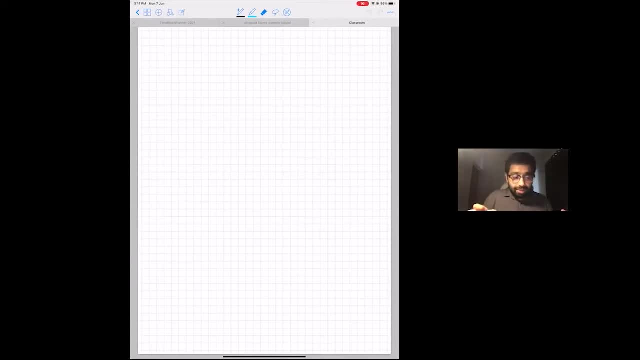 many body system with many particles, many atoms that are cold and are very controllable. okay, now, as a result of this control, you can essentially make any desired many body Hamiltonian that you are interested in. okay, why is this interesting? this is interesting for this very important reason: as condensed matter physics, which is the study of electrons and solids, became 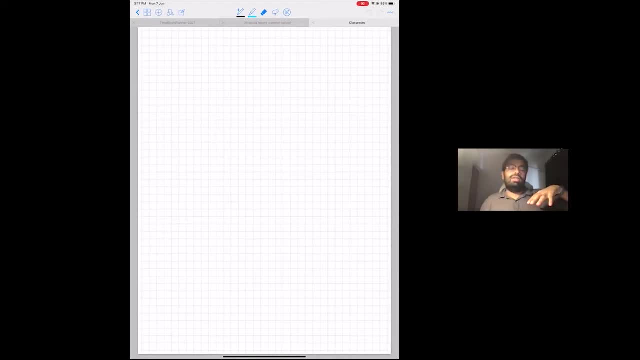 more and more interesting and complex. people saw a host of interesting phenomena just of solids based on magnetism, superconductivity, and this whole field which has been going on for a long time, is called strongly correlated matter, where everything, the degrees of the fundamental degrees of freedom, are well known. it is just electrons and they are notь speaking about fé. iseg is not a l'estat. 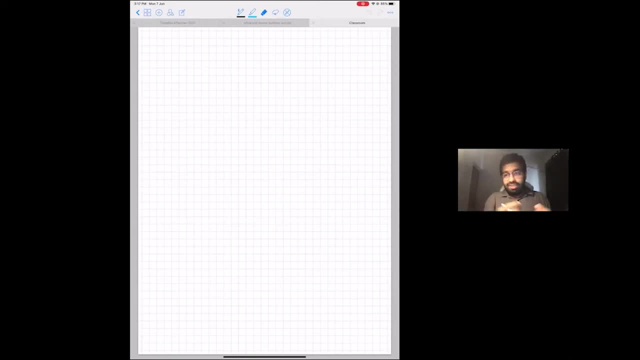 and it's just interacting electrons in some lattice. Now the problem is: this is very easy to specify, but in order to actually understand the thermodynamic limit phenomena that you get from such simple fundamental interactions is extremely hard in such strongly interacting correlated systems, For example. one big problem there is if n is of the order of 10 to the 23. 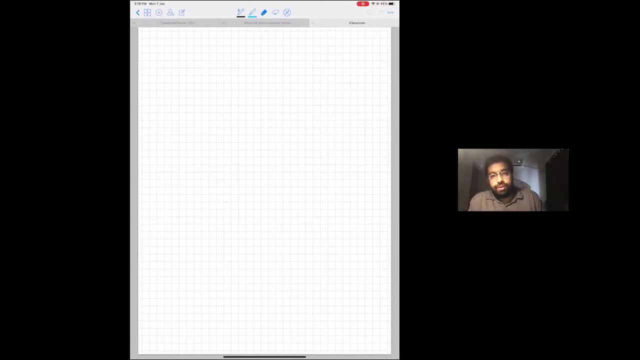 if you wanted to run the solution of a Schrodinger equation for the electrons in a solid. that's going to just be impossible to do on any classical computer. So there was a very interesting suggestion. long before quantum computing became what it is today, there was a very interesting. 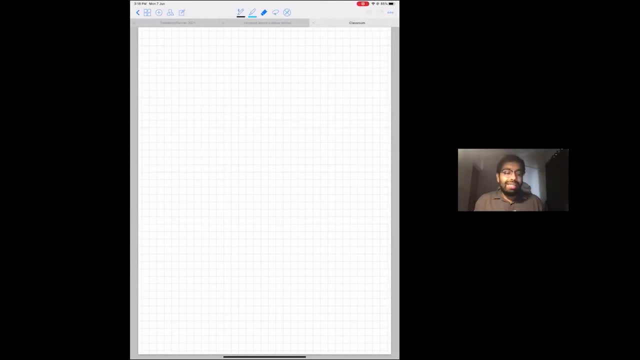 suggestion from Feynman to design a kind of an analog quantum computer, which is called a quantum simulator, made up of other quantum systems to actually study a hard to simulate quantum system. So now, since I have, with these Bose-Einstein, condensates in lattices, in optical lattices, with such control I can basically mimic the Hamiltonian. 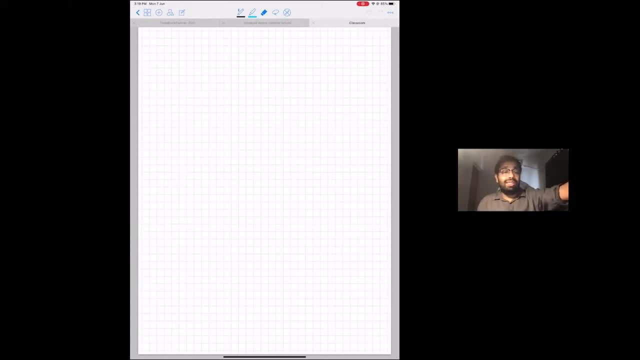 of any interesting system that I want to study and basically study it experimentally and understand the properties of the system which are otherwise impossible to do by, say, computation or by analytical methods. So this is a very big reason why Bose-Einstein condensates are fundamentally 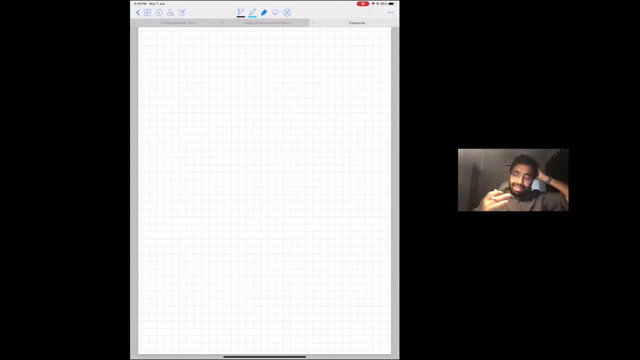 interesting. And then of course, in along these lines, there are also very interesting proposals to use Bose-Einstein condensates as, in some sense, the fundamental processors of quantum computers and so on, but that's sort of not, let's say, the most advanced platform right now for quantum computing. 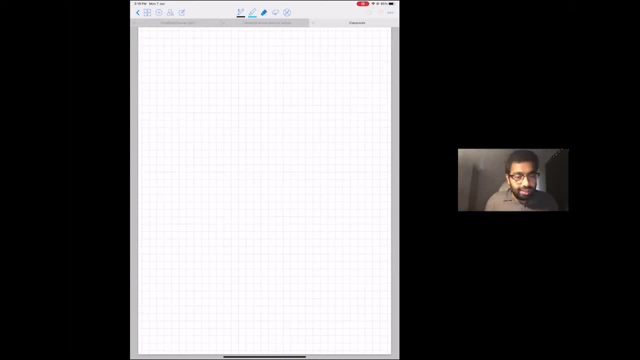 That's sort of the reason why Bose-Einstein condensates are interesting to study, okay. So now I think we can move on and start being less wishy-washy about things and be a little bit more rigorous and answer the question: what is a Bose-Einstein condensate? exactly okay. 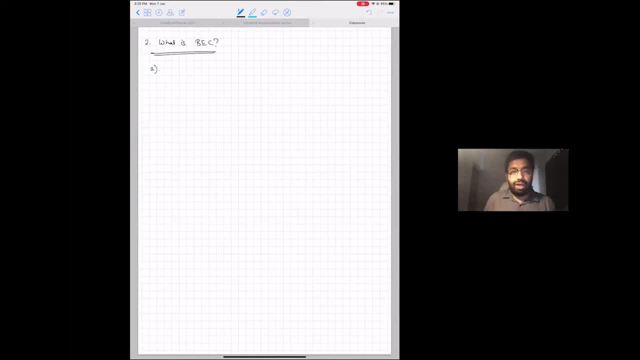 Good, so I'm going to give two answers, two long answers, for this question. The first part is going to be a little bit more familiar, especially if you've done some statistical mechanisms. So the first part is just a more rigorous and mathematical way to describe what I have been saying in words, which is a Bose-Einstein condensate. 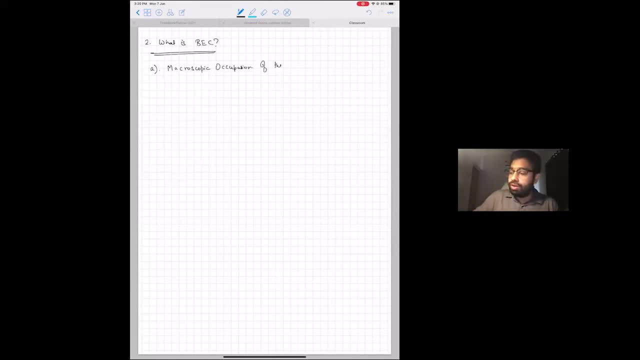 is just macroscopic occupation of the ground state of a non-interacting Bose gas, so an ideal Bose gas. So I want to qualify all of this by really studying the statistical mechanics, in some sense, of an ideal Bose gas and show how Bose-Einstein condensation comes about there. okay, So towards. 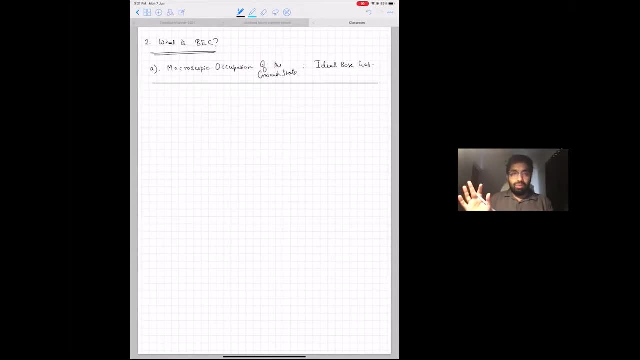 that. consider now a non-interacting, indistinguishable bosons just point particles at thermal equilibrium in some grand canonical ensemble at some temperature. T. okay, and let's call β1 over kdT. okay, and it's also in equilibrium because it's grand canonical ensemble. it also has 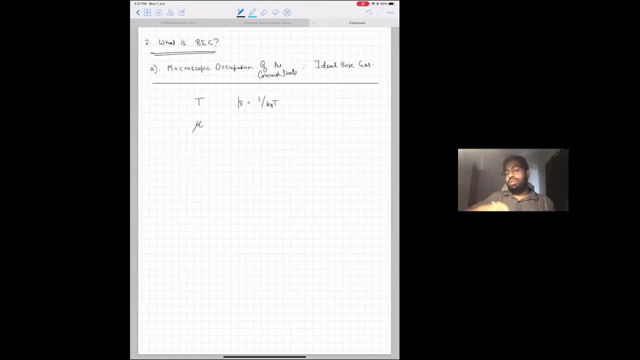 a chemical potential μ, and so it's in equilibrium with some chemical potential bar. Of course, the idea is that we are using this for the theoretical description, but because all ensembles are equivalent when the number of particles is large, this is largely a trick to make our life simpler in term of 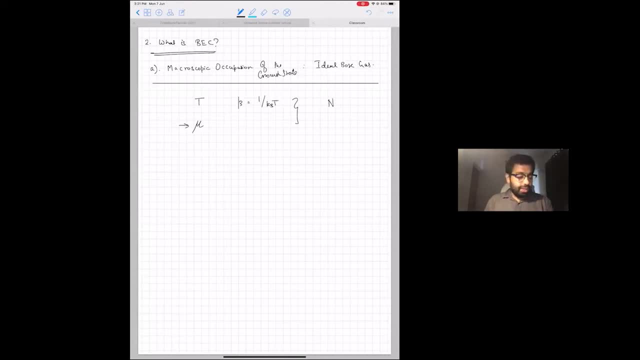 terms of calculating partition functions and so on. okay, so in this situation, in describing ideal, non-interacting bosons in the grand canonical ensemble, one knows that the microstates of the system these are not. you no longer specify them by telling me what is the individual quantum state. 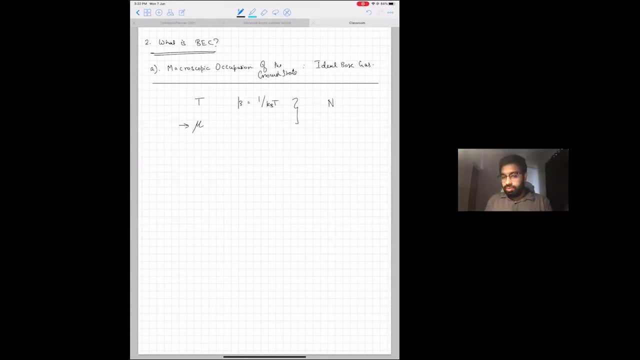 of each particle, but instead, because these are completely indistinguishable, you just have to specify the occupation numbers of single particle states. okay, so, let me use a symbol for this: sps. okay, so, in a quantum mechanical system, i've already told you what is the meaning of a. 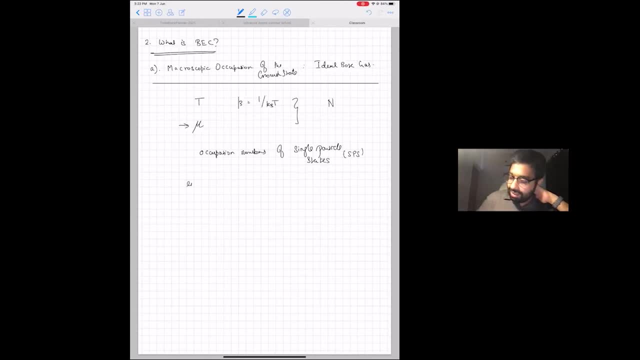 single particle state. these are simply, for our purpose, eigenstates. these are basically quantum states of each particle of this collection of bosons, but you can choose them to be anything but the most important class of single particle states that, when you do statistical mechanics, is just the eigenstates of the single particle hamiltonian. 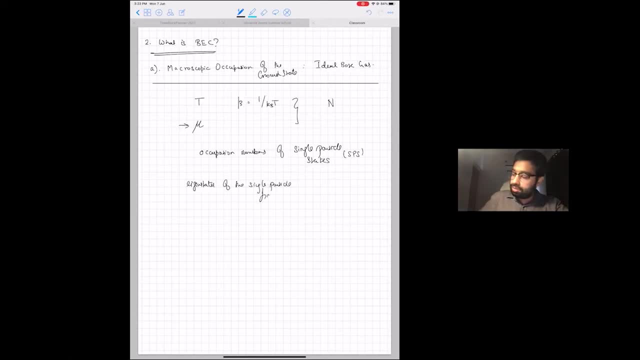 okay, so let's call the energy of these eigenstates e mu and let's call these- we don't need it for now, but you can call the states themselves mu. and let's look at a couple of examples of what are single particle hamiltonians and single particle eigenstates. 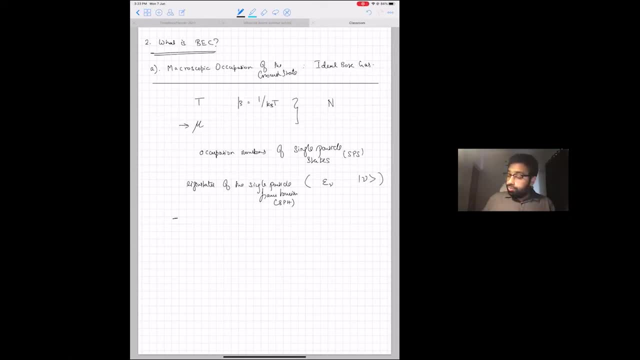 one example: three particles in some volume b- we just discussed them extensively. in this case, this mu, which tells you the quantum numbers describing the single particle states, are just wave vectors and or momentum is given by h bar k and energy is just h bar squared, k squared by 2m, and the single particle 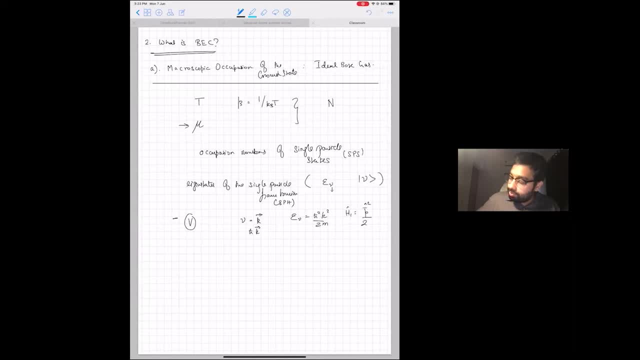 hamiltonian is just p squared by 2m. okay, this is the single particle energy and this is the single particle hamiltonian. and the eigenstates are just this, and these eigenstates are just plain waves if you write them in position basis. this is just e to the i k dot r over square root b. 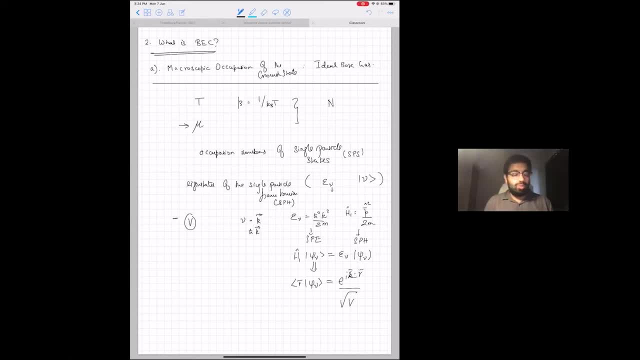 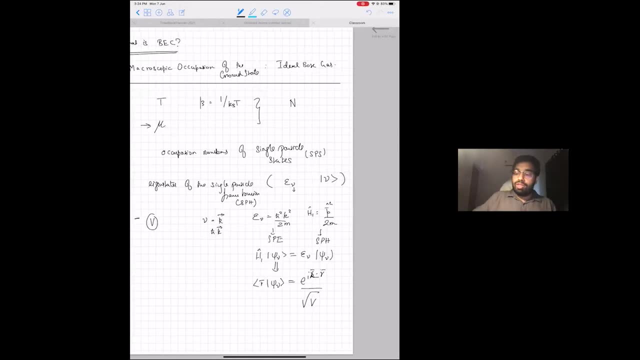 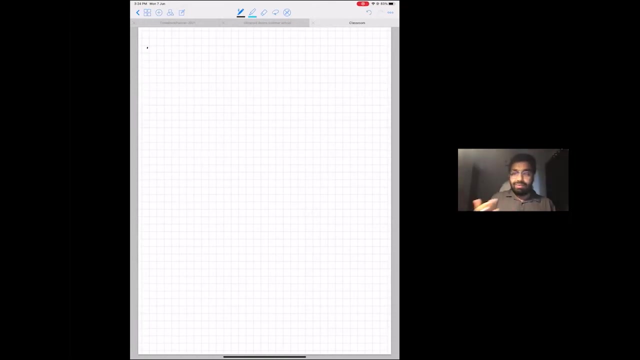 right, i hope this part should be really familiar to most of you. okay, so that's one example of a single particle hamiltonian and single particle energies. another important example, because we will actually consider particles in a trapped, particles in a three-dimensional harmonic trap, which is very relevant to the experimental boson strength condensates that i showed you. 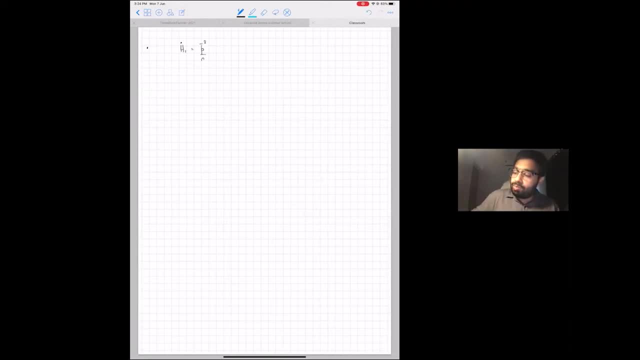 in this case my hamiltonian. the single particle hamiltonian is p squared by 2m plus half m omega 1 squared x squared, omega 2 squared y squared, plus omega 3 squared z squared right. so this is basically a harmonic oscillator with different frequencies along the x- y. 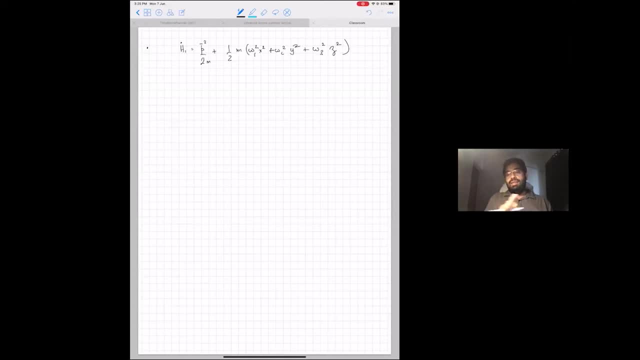 and z direction. so possibly, uh, not isotropic harmonic oscillator. of course, this is a very easy system to find the energy eigenvalues of. so the energy, energy is an eigenvalue, so the quantum numbers are just three integers and one and two and three right and my e nu, the energies. 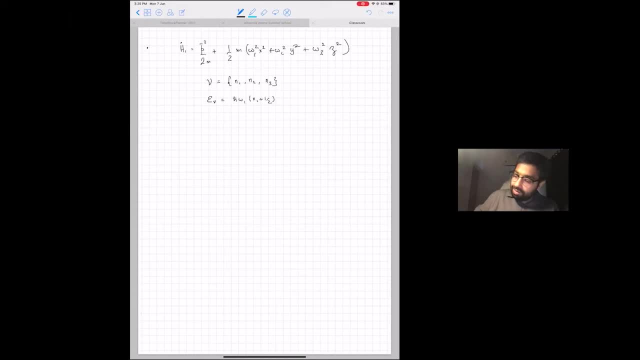 are just given by h bar omega one and one plus half. i can just write it as some override h bar omega i n i plus half, right, so maybe i like it a little bit bigger. those are my energies and of. i know the states as well. these are just the product of the three harmonic oscillator wave. 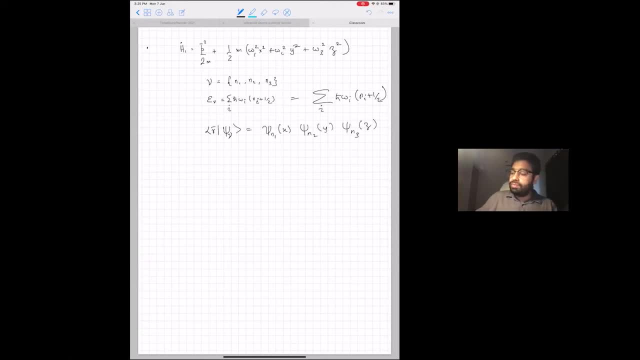 function along each of these directions. these are just the 1d harmonic oscillator eigenfunctions, right? so these are examples of some single particle states. okay, so now, as i said, our microstates are simply given by the occupation number of these different states and using the distribution function, using the probability distribution function for the 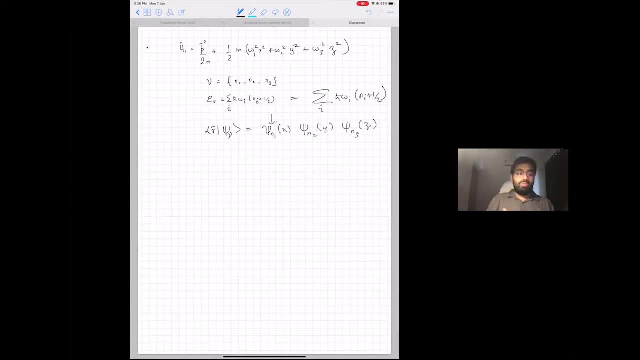 microstates, one can actually derive an even more important quantity, which is called the distribution function, right, okay so, which simply gives you the occupation number. what is the occupation number of a given single particle state? okay, because these are non-interacting. you start with a microstate and you can actually calculate. you can start with the probability of a microstate. 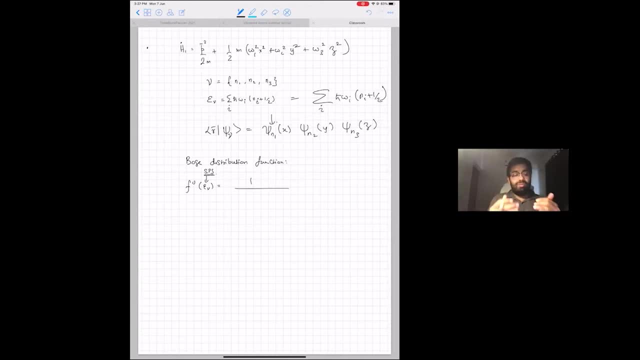 in a grand canonical ensemble and from that derive this both distribution function, which tells you the occupation probability of a single particle state, and from that derive the probability of each of these single particle energy states. okay, and this is simply given by this function. right, and this is again something that should be familiar. it's very famous both. 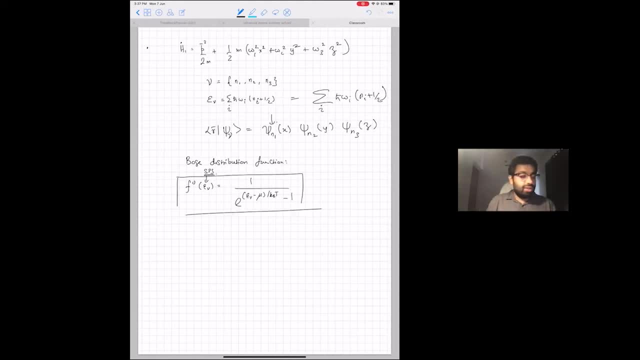 distribution function okay. so now it becomes very clear that if you look at, if you call e minimum the lowest energy, lowest sinkhole energy, the lowest energy, the lowest sinkhole energy, the lowest sinkhole energy, single particle energy, right, For example, in the harmonic oscillator, it is just sum over. i. 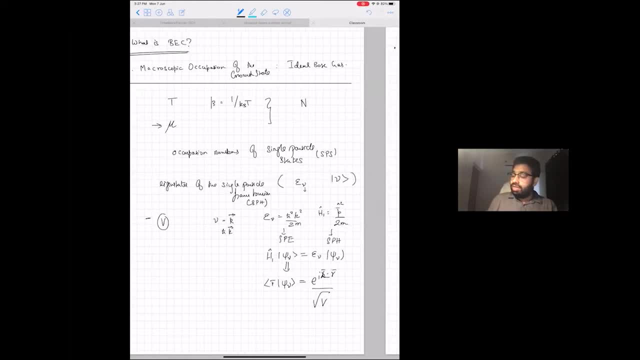 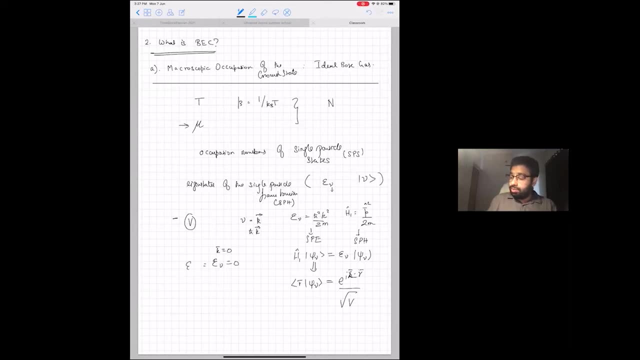 h bar omega i by 2.. For the plane waves it is just E mu equal to 0. So the k equal to 0 state, that is the E min right, And whatever it is, if you have a minimum temperature minimum. 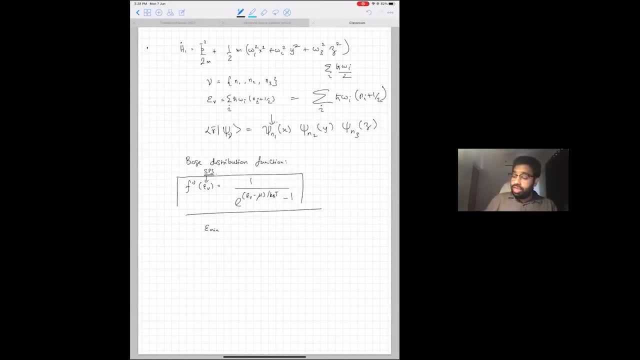 energy of E min, then your chemical potential for this distribution to make sense has to always be greater than this minimum potential right. Otherwise the occupation probability of the zero energy or the ground state this will be negative. So this is required for this to. 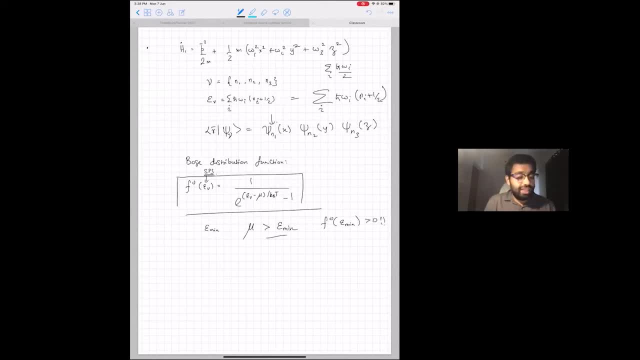 be positive, right, And otherwise it does not make any sense. okay, Another related quantity: so mu is always greater than E min. okay, And related quantity is basically called this fugacity, which is E to the beta mu. okay, And from this, using this distribution function, 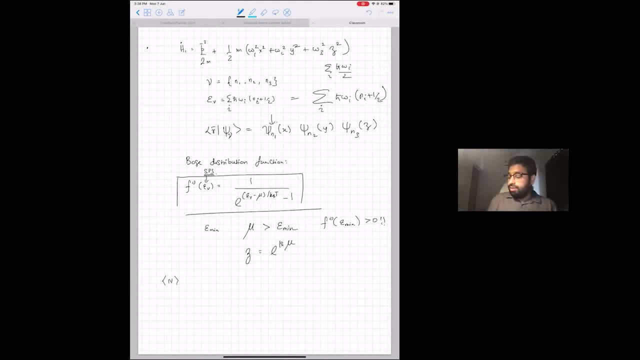 one can write the average number of particles, which is same, which is approximately just the number of particles. So this is in the grand canonical ensemble and this is in some sense in the canonical, Because ensembles are equivalent at very large n. you can think of this average n as basically: 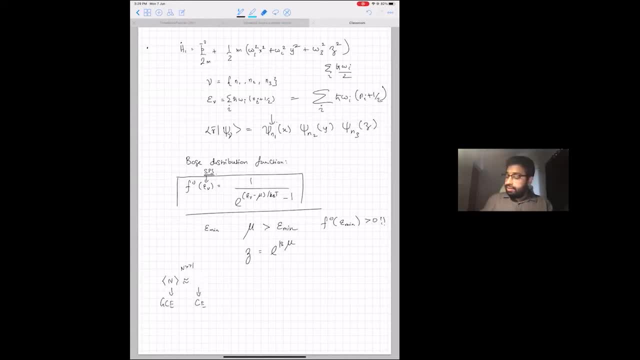 just the number of particles that we have, and we can write n simply as sum over mu, f0 of E, min right. So you sum over the occupation of each of these single particle levels to get the total number of particles. okay. 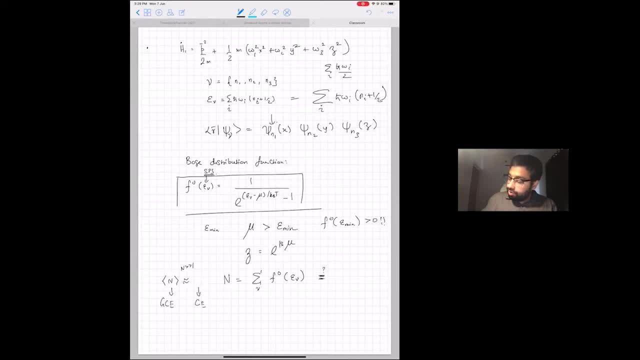 And we can convert. for many of these systems we can convert this sum over different energy eigenstates into an integral over energies with a factor which is called the density of states, right Times f0.. This is a very allowed kind of conversion, direct conversion under most. circumstances, but there is a reason why we are not able to convert it. So this is a very allowed kind of conversion under most circumstances, but there is a reason why we are not able to convert it. So this is a very allowed kind of conversion under most circumstances, but there is a reason why. 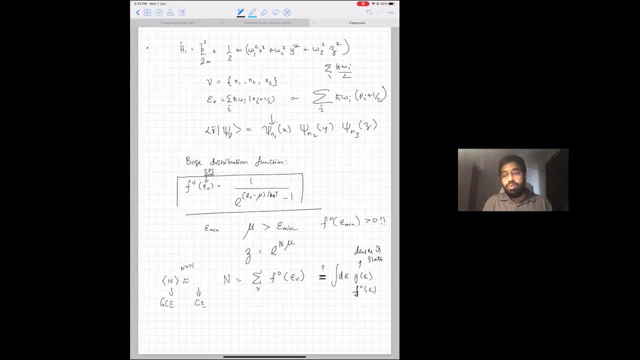 I am putting question mark about here that one has to be careful about this at extremely low temperatures. So we will come to this when describing the B's. okay, So now let's look at how basically this Bose distribution function behaves and what happens as you keep. 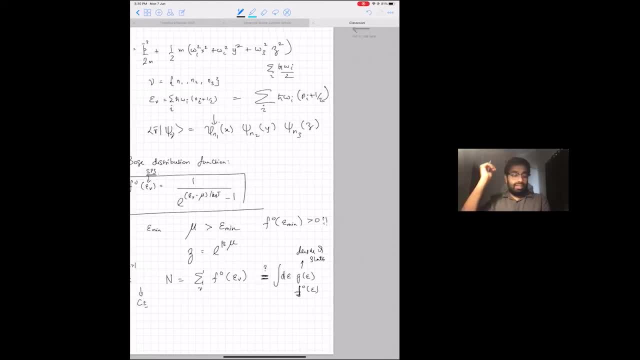 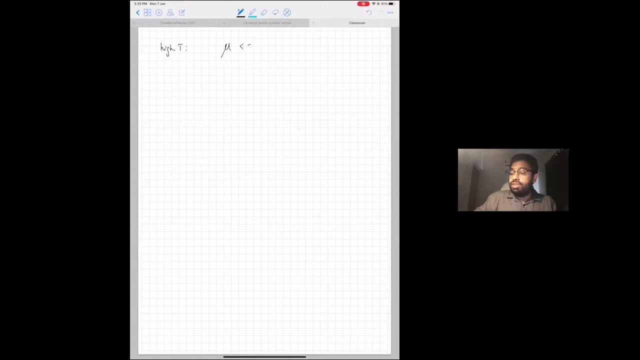 going to lower and lower temperatures to understand what a Bose Einstein constant is. Okay, So at really high temperatures, right, Okay, Okay, Okay, potential is much smaller than the minimum energy that you have in your single particle. basically, this is something that one can work out from the grand canonical ensemble, but for 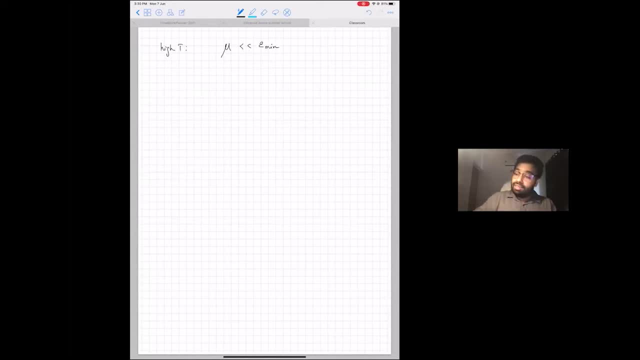 now you can take my word, but this means so. this means that if you look at the Bose distribution function at really high temperatures it takes a very familiar form, which is just e to the minus, e, mu, minus mu over k, B, T. why is this familiar? for example, if you take free particles, this: 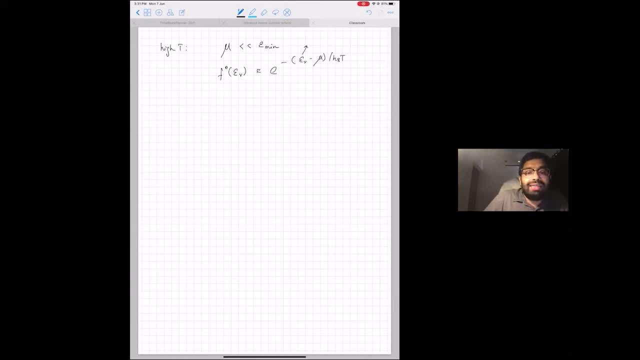 essentially e nu becomes p squared by 2 m, and this is really. you can use this to derive the Maxwell-Boltzmann distribution for p velocities. so at high temperatures of course, this is precisely the picture that we started with of particles bouncing around like billiards with some Maxwell-Boltzmann distribution for. 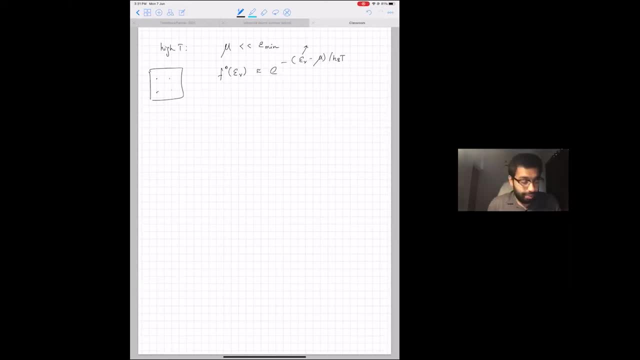 their velocities. okay, this is what happens at very high temperatures. okay, but okay, I think I might have made a mistake. let me, let me just check one thing: I might have said something wrong regarding mu. right again, I think I'm making the greater than or less than error. so 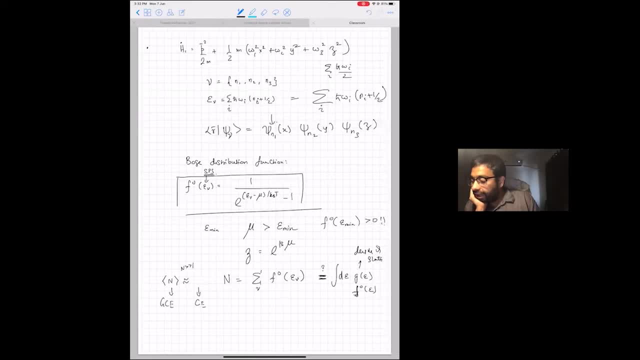 let me get to this part. so if I have mu greater than sorry, this is really stupid. so if mu is greater than e nu, then this would give me, of course, e to the e nu minus mu will be. this would be negative. so this would be less than one and then you would get a negative occupation. so 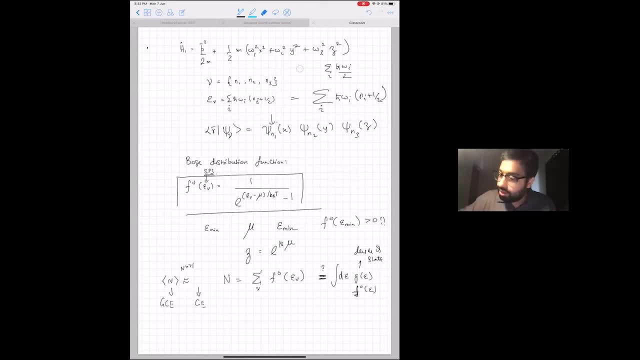 what I meant here- that was stupid- is that mu should always be greater than the minimum energy, So the chemical potential has to always be above the minimum allowed rate. Let me just think for a moment. So, yeah, Okay, So I do need a mu minus mu to be greater than zero, So mu. 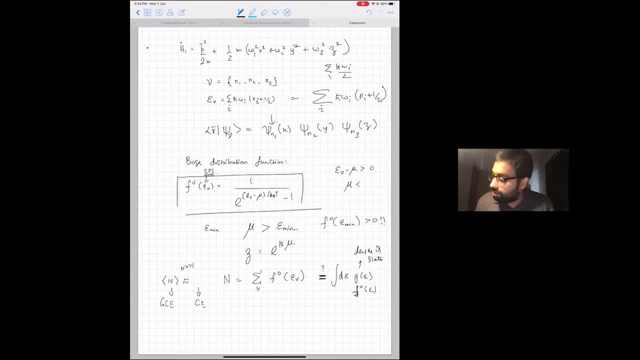 should always be less than mu. So I can ensure that by making mu less than the minimum. Okay, So this is my criterion, right? This is my criterion for Bose distribution function to be positive. So that's fine. And what happens at really high temperatures is that mu is. 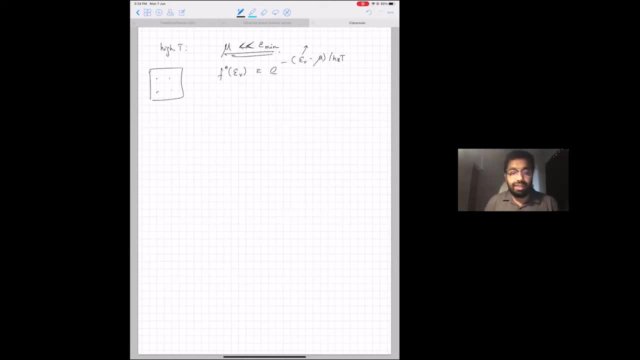 much less than mu. Okay, So sorry about that. That was an error from the phone. Okay, So now sorry, did I have a comment? Hello, Can I interrupt for a second, Sir? yeah, So the temperature here comes out as a common factor, right? So what exactly? 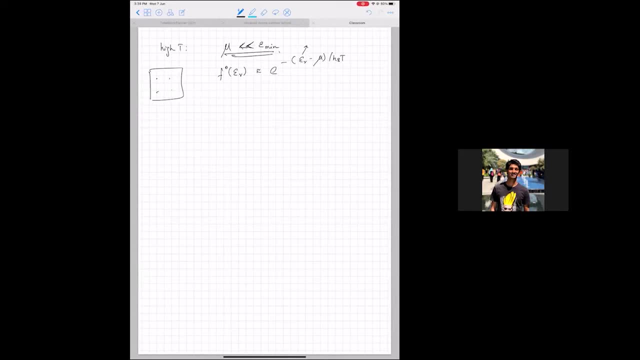 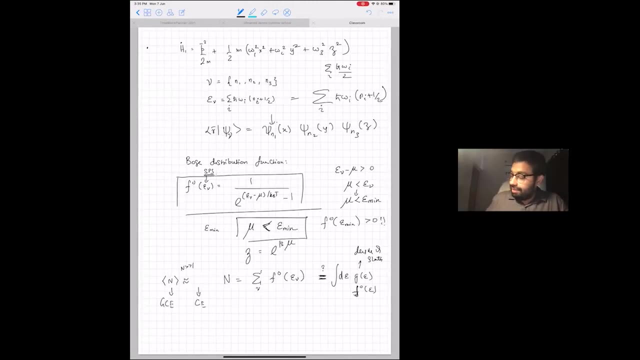 do you mean by saying that at high temperatures? So that is again a very good question. So the idea is as follows. So the idea is that when you look at this equation, when you actually plug in the Bose distribution function- which is something I should have mentioned- what you get is n in terms of mu and t. Okay, So if I 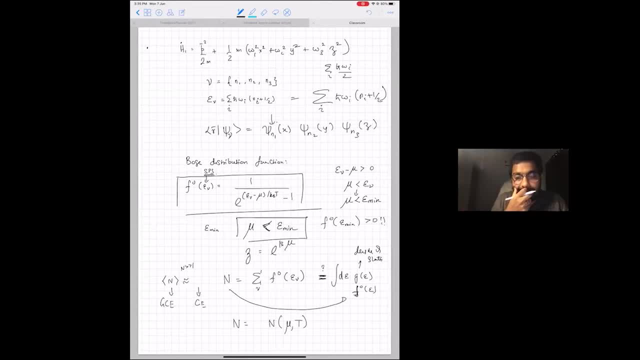 just plug in the Bose distribution function and if I'm able to evaluate this integral right, we'll get into that detail later. But this equation gives me the number of particles as a function of mu and temperature. I can invert this to write mu as a function of n and t. Okay, So this tells me actually which. 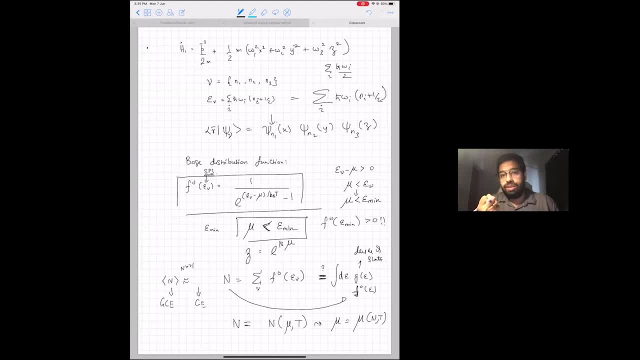 is very important that the chemical potential of course depends on the temperature, even in a non-interacting system, And the reason is you have to go back to what is the definition of chemical potential. It is the rate of change of energy with respect to the number of particles. 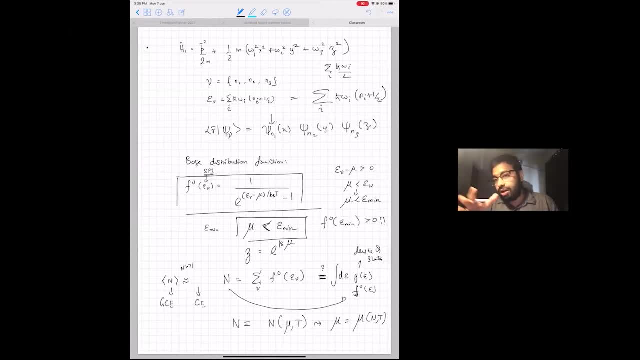 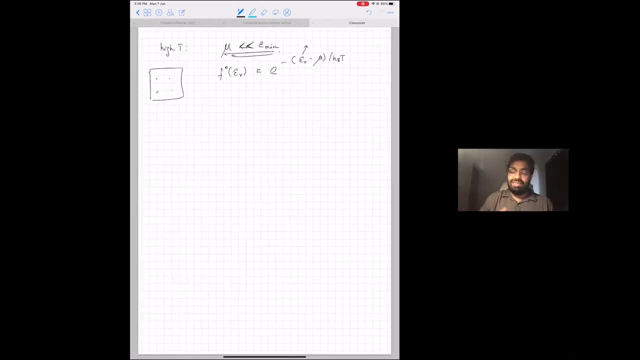 at fixed entropy. Okay, So now, as you go to lower temperature, the entropy is different, So mu will depend on temperature, even if it is non-interactive. Is this clear? Oh yes, sir, I understand What I mean by saying that mu becomes much less than e min. mu basically goes to minus infinity, as 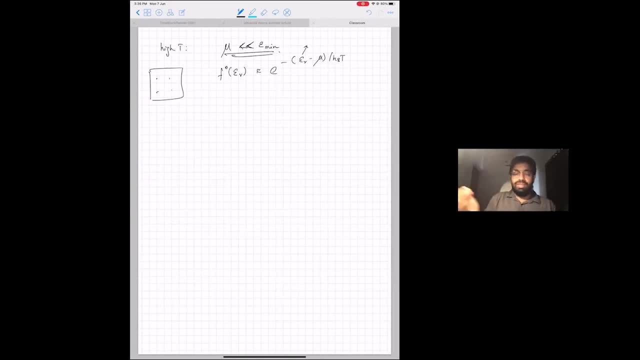 t goes to infinity. basically, That's the idea. Okay, So with this, of course, high temperature behavior is easy to understand. So now what happens? Okay, So with this, of course, high temperature behavior is easy to understand. So now what happens? 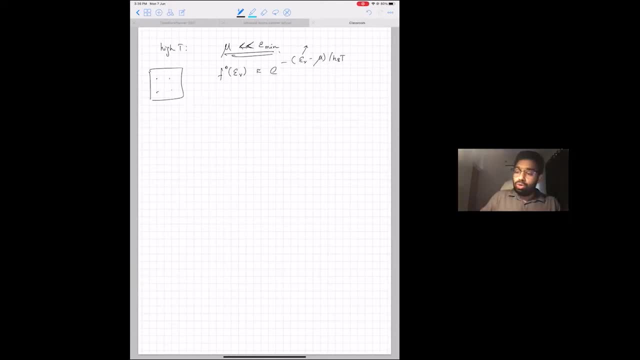 So now what happens If I keep going to lower? and so okay, one important thing about this high temperature behavior is, if you look at F0 of the ground state, which is e min, that is, e mu minus e min over kbp, And this when mu is much less than e, min is much less than 1, right? So that is the 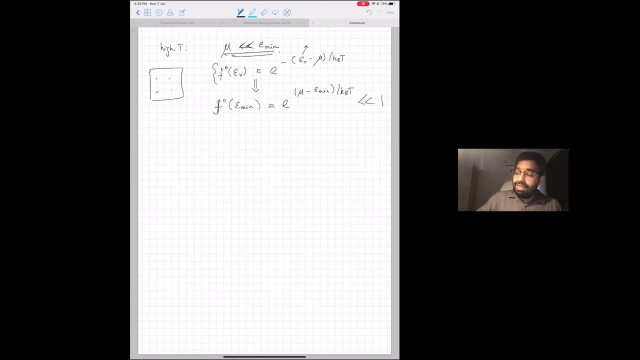 problem. Okay, So at very high temperatures there is essentially low occupation of the ground state And in general, the higher energy states I can really write down as some kind of Maxwell-Boltzmann-like distribution. Okay, But now what happens as I lower my temperature? And that is where the interesting physics is. 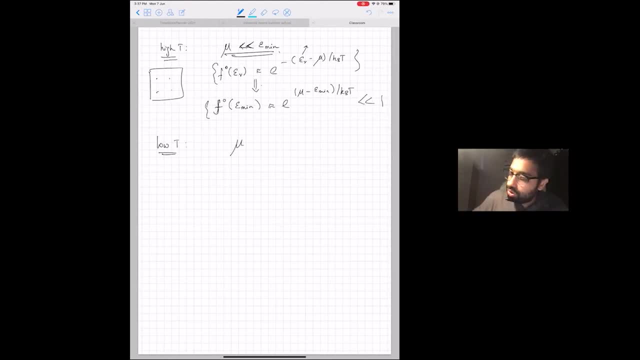 Okay. So now the issue is that mu starts increasing. Okay, But we are always bound by this. mu is less than e min Okay. So as t is decreased, mu increases, but mu is always below e min Okay. Therefore. 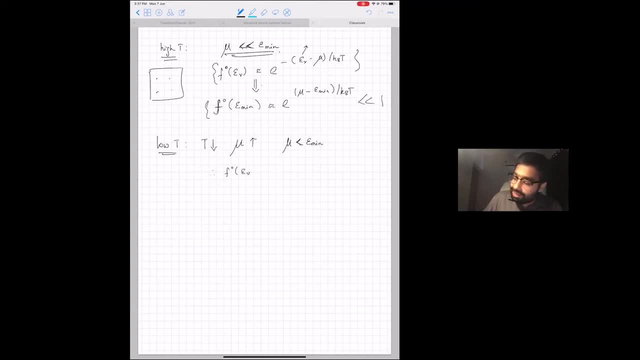 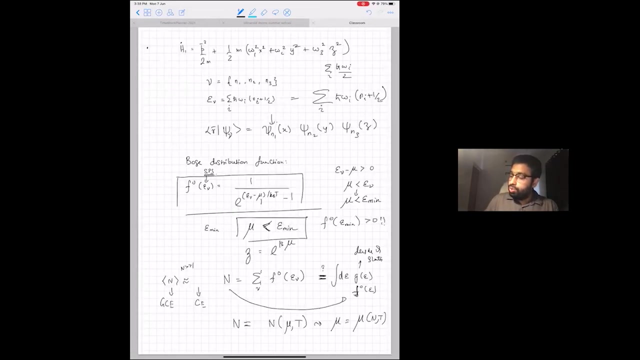 if you look at the occupation of any of the excited states, they have to be less than 1 over e. mu minus e, min over kbp minus 1.. Right, So I'm just plugging in in the Boltz distribution function For mu. I'm just plugging in the maximum value it can take. 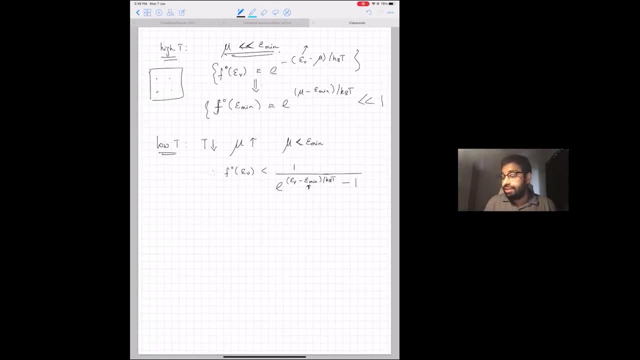 which is the lowest energy, the ground state energy. Right Now, here's where I can give you another heuristic explanation of a Bose-Einstein coincidence. What is happening? So, if I keep lowering my temperature, my occupation, probabilities of any of my excited states? 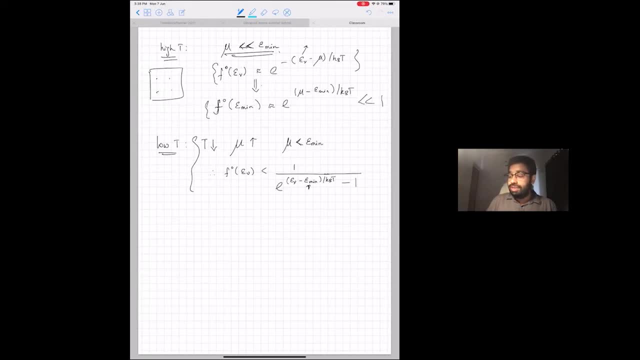 is becoming smaller and smaller and smaller, They will reach some saturation above which they cannot grow, Okay. And the saturation value is also getting smaller with as temperature goes. as temperature becomes lower- Okay, As a result, below a certain temperature. 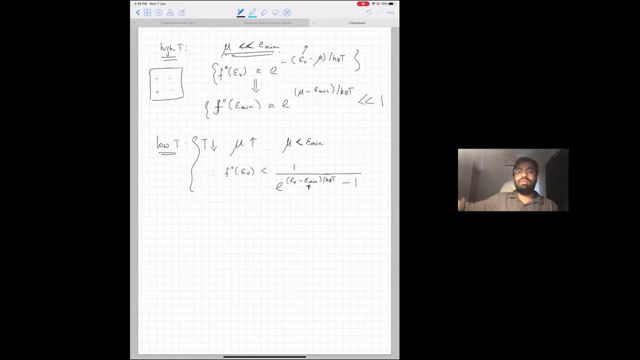 I will not be able to fit in all of my atoms in the excited states And I have to push not just one atom but a macroscopic number of them into my ground state. And I am allowed to do that precisely because there is no such bound. 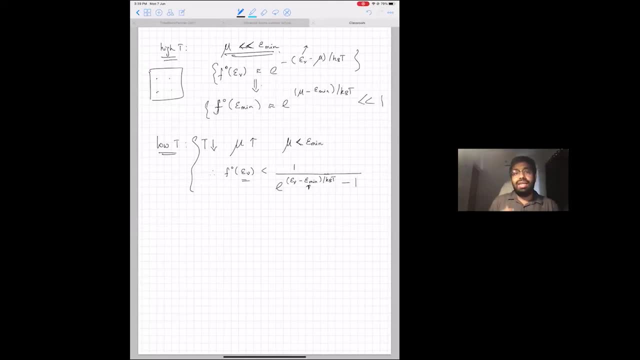 for the ground state Right. So the ground state occupation can continue to increase In principle at t equal to zero. as we will see, it will go to the total. all the particles will be in the ground state, So it can go as large as n, But the excited state. 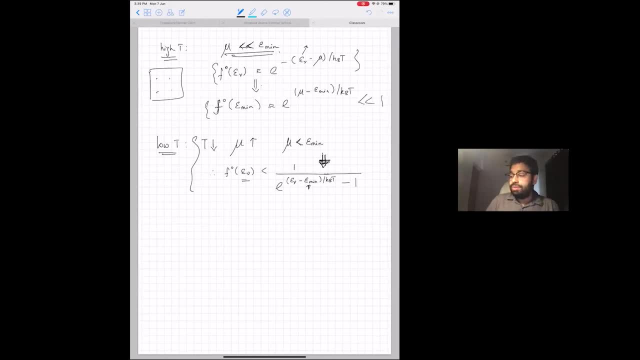 occupation is always bounded by this. Okay, So that is the key idea: that because of the Bose distribution function, you can push more and more atoms into the ground state as you go to lower temperatures. But that's not possible. You're not able to do that with the excited states. 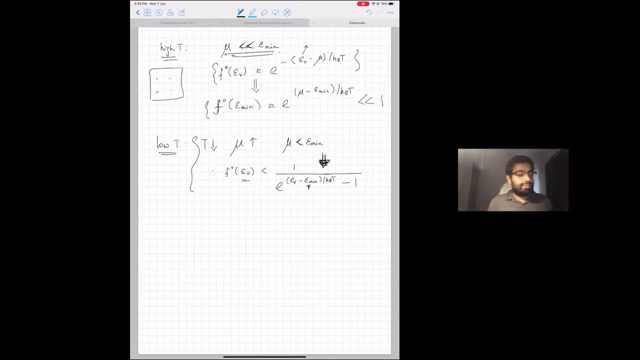 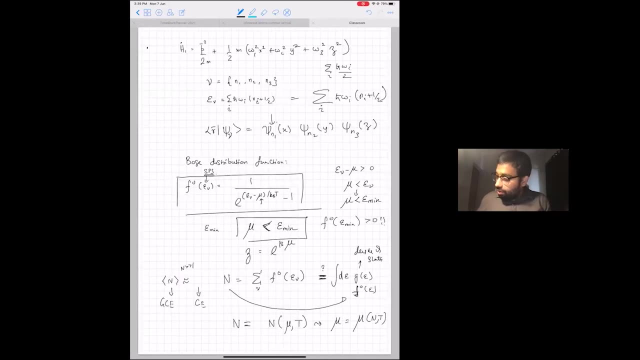 And that is at the heart of why you get a Bose Einstein function Okay, But of course, as we showed here, the excited state or basically the way that we are writing this function, it tells us a little bit about the fact that not only the Bose function 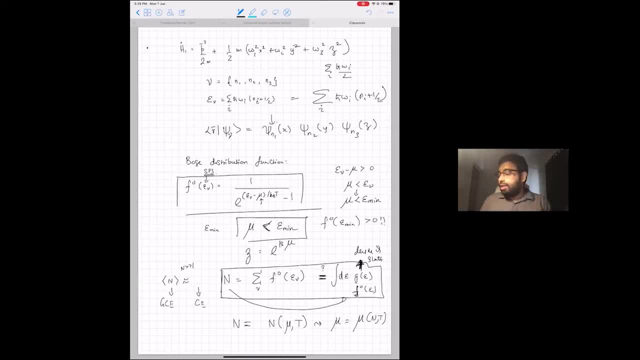 but also this density of states can play an important role as to whether you can, at what temperature you will have this Bose condensate, as well as whether you can have a Bose condensate that is set by this density of states. Okay, So now let's go and look at the 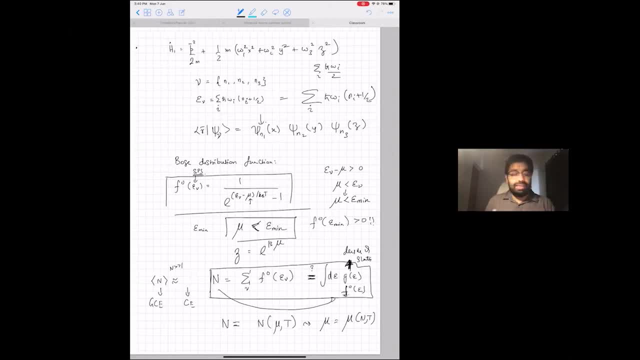 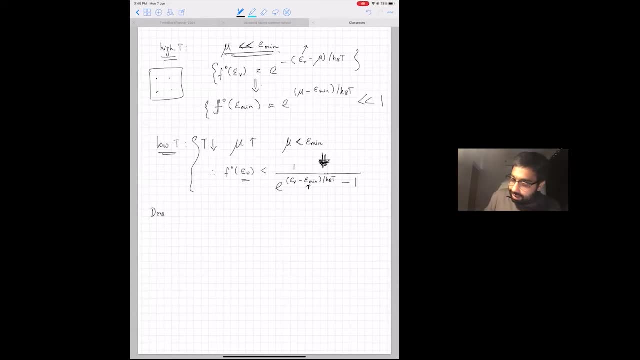 effect of this density of states and actually work out this Bose condensation temperature, for example, and the idea of this Bose condensation. Okay, So now this density of states is very simple. This is again something that is from basic stat mech, right, What is the density of states? So this g of e, d, e gives you the number of single. 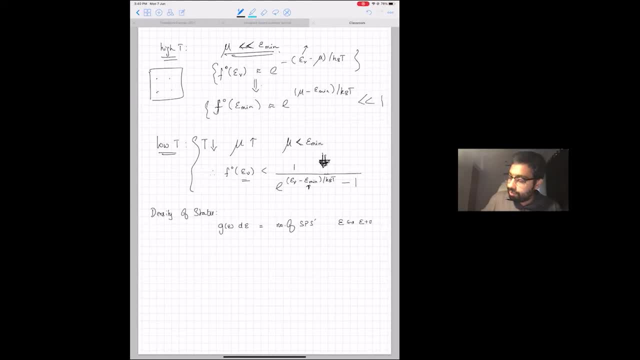 particle states between energy: e to e plus d. How does that work? How? this is the definition of density of states. How does one compute that? You first compute this capital G of e, which is simply the number of single particle states with energy less than or equal to e. 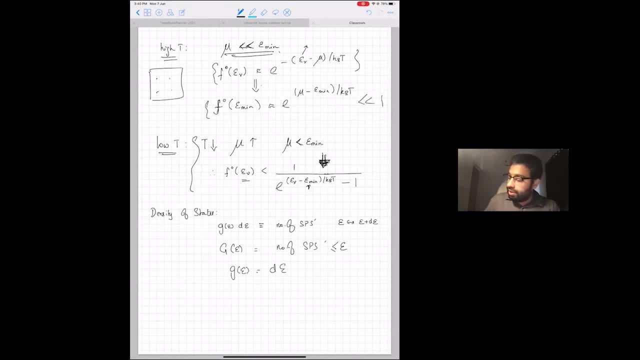 Then it's just very simple to see that this density of states is simply the derivative of this d g of e with respect to p. So let us quickly calculate it for two cases. I'll not do it in detail, I have it in the notes and this is very basic stat mech And I encourage you to go. 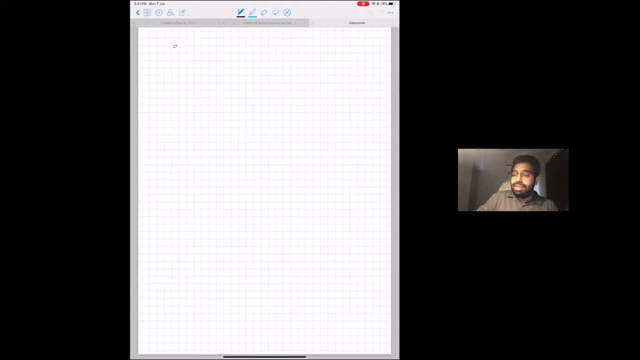 and see this. So for particles in three dimension right. So my energy e is given by p squared by 2m. G of e, for example, is the density of states between energy e to e plus d d e, plus d e plus d e. 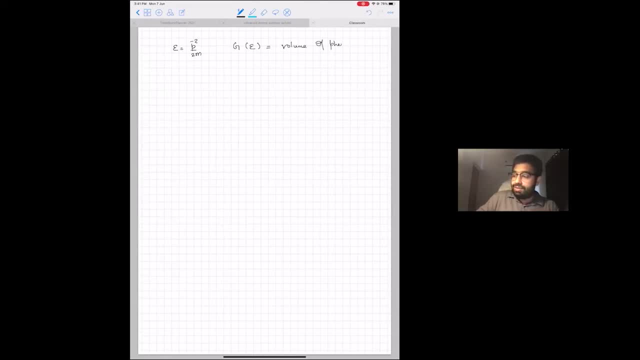 the volume of phase space or energy space, with less than e divided by the volume occupied by a single quantum state, which is essentially h cube right? so if you calculate the volume of phase space under this energy e, so realize that this density of states is essentially not a quantum thing, it's. it's something that is there in classical physics as well as soon. 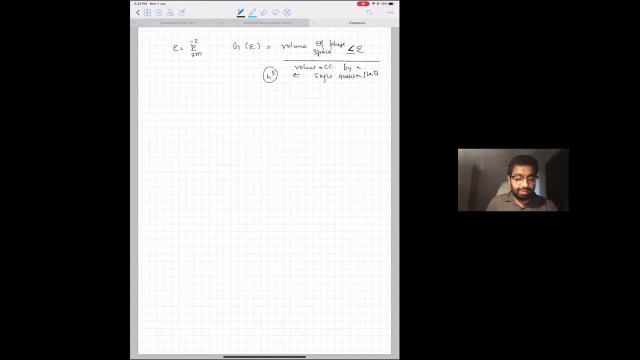 as you give me an hamiltonian, i can actually calculate this. and if you tell me the spectrum of the hamiltonian, i can calculate this right. and so this is for uh, for this, three particles. it's just v times four by three: pi, p, e cube where p? e squared. 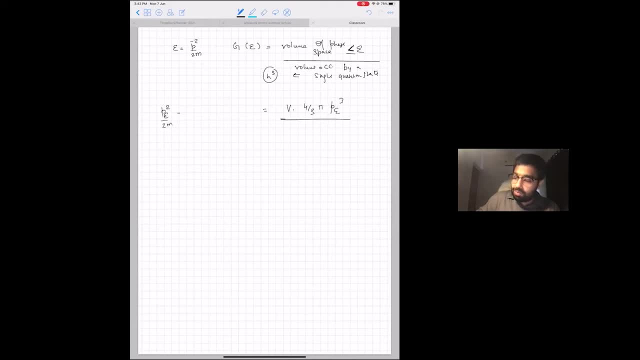 by two m is e. so it's essentially all. the this is the volume of a sphere uh of radius: two m e in square root, two m e in momentum space. right, that's all. and then i can calculate this very quickly after a little bit of work, and the answer for g of e comes out to be square. 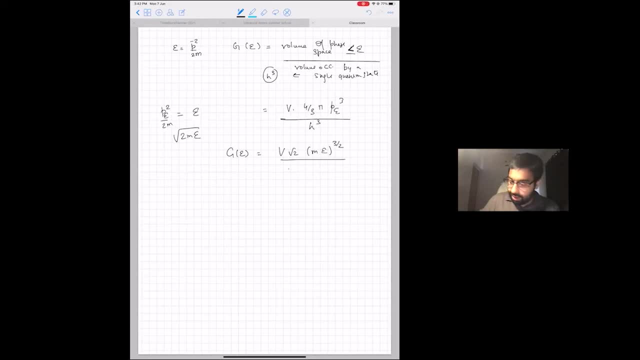 root two, m e to the three by two divided by three, pi squared h bar cube. okay, and from this the key quantity is: how does it scale with energy? it scales as e raised to three by two. this is telling you two things. the cube here is coming from the fact that we are working in three dimension. 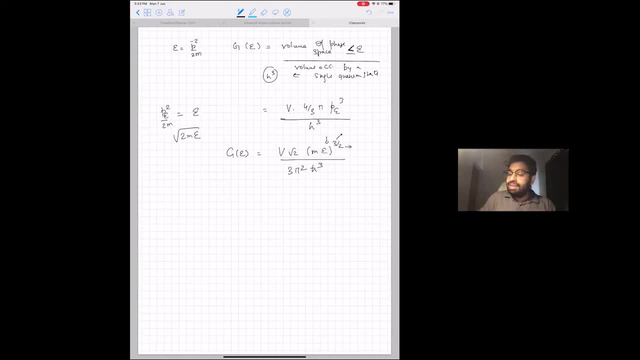 and the by two is telling us the relation between e and the momentum. right, it is p e square. okay, so using this one can immediately write the density of states for particles in a box. that's just v, m to the three by two: square root, two pi squared. 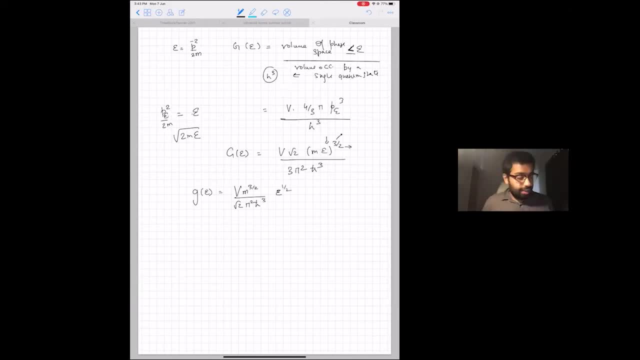 h bar cube e to the half. okay, and in the same vein, i'm not going to do this if i have basically a harmonic oscillator potential, which we just talked about, with this kind of energy: h bar omega i n, i plus half, i goes from one to three. 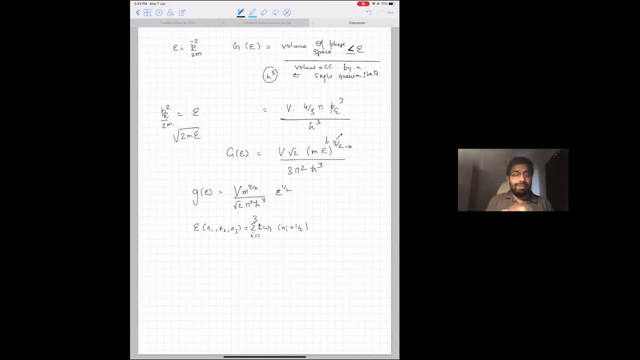 right, then again you can do the same idea. in this case, you have to calculate the volume of, not a sphere but an ellipsoid in in, basically, six dimensional phase space, which is, again, geometrically very easy to do. after a little bit of work, you will see, and if you want, you. 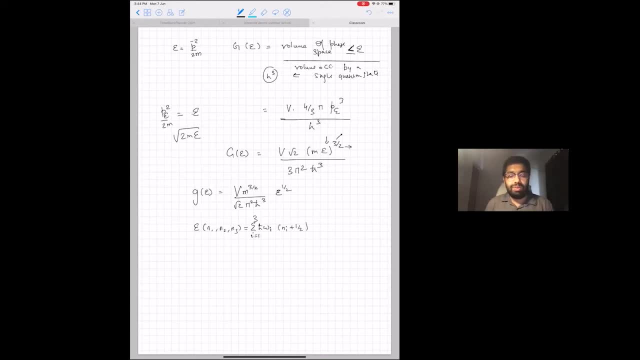 can look at the notes that will be available on the uh on the website and you will see that this leads to. so this is for free particles. now for a 3d harmonic oscillator, you get g of e. is some e cube by six, h bar cube omega. 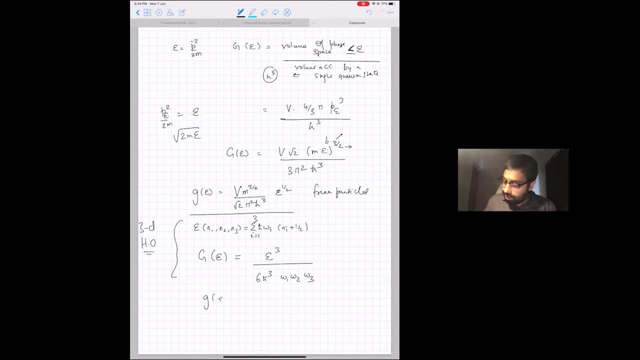 one, omega two, omega three, and g of e is precisely e squared by two: h bar cube, omega one, omega two, omega three. okay, so you get. i just wanted to illustrate two very different kinds of density of states, but this, at the end of the day, this gives us what is the correct form. we have to. 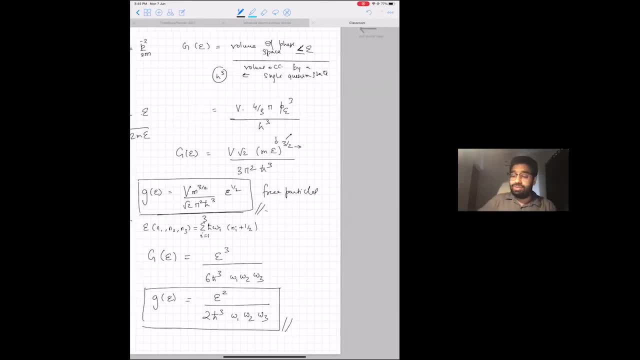 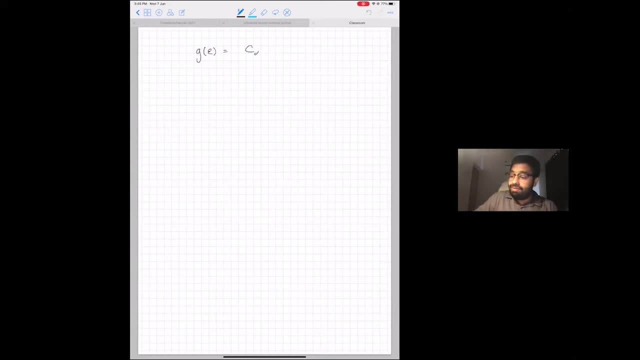 assume for the density of states. we are going to assume a general density of states and calculate this. bc transition g of e can be taken as c alpha e to the alpha minus one. for free particles, alpha is in three dimension. alpha is three by two and this constant c three by two is three by two and 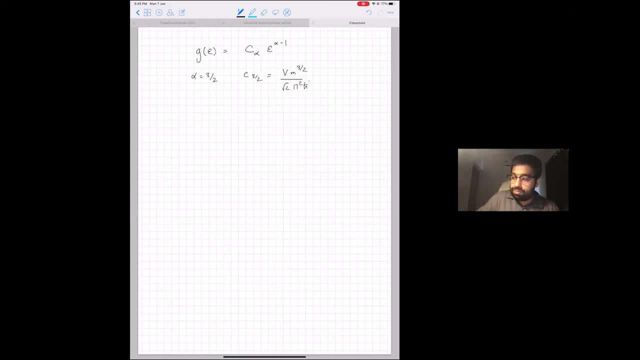 c is just this for a harmonic oscillator in three dimensions. alpha is three and this c three is one over two: h bar cube, omega one, omega, two, omega. now we want to take this density of states and go back to our expression that we had for the total number of atoms in terms of the 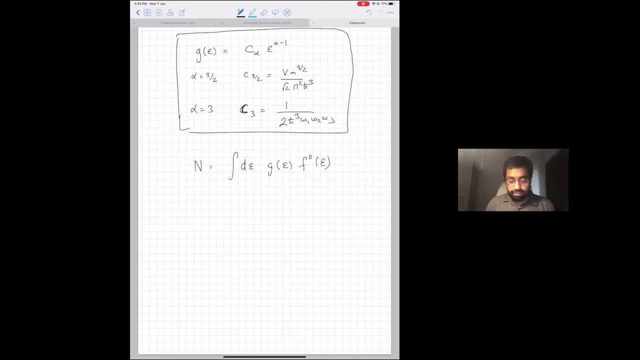 in terms of the bose distribution function, and look at this and look at what happens to this quantity as we go to lower and lower temperatures. okay, so now let's do that. now let's focus, for example, on on a case where we can ignore the minimum temperature, minimum energy, right? so i'm going to 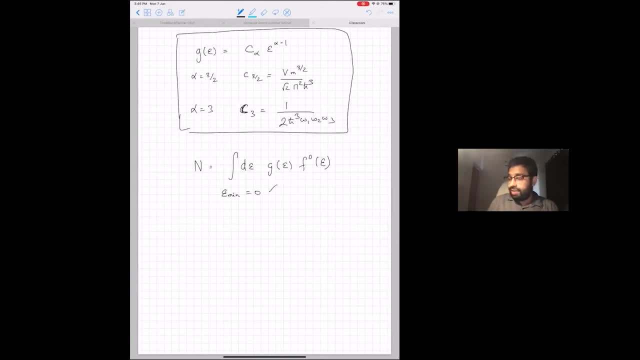 set this minimum to be zero. this is perfectly correct if i have three particles. k equal to zero has energy zero, but for the harmonic oscillator there is some vacuum energy. so e minimum is not technically zero, but it will only change things quantitatively slightly whatever we are going to do. so it's all right. so let me keep it at. 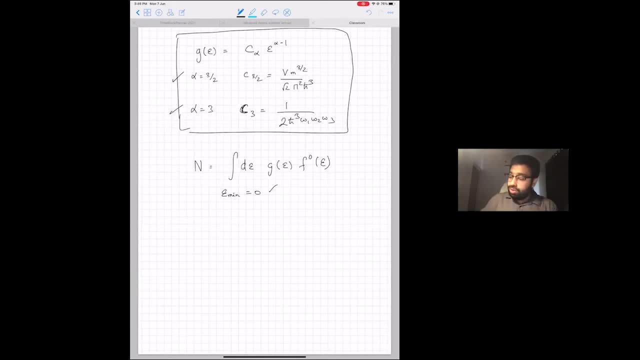 zero, and let me look at what happens then. so now this means that mu has to always be negative and the maximum value it can take is zero. right, with this, i can plug in into this expression for n, which is written now as temperature and chemical potential dependent. 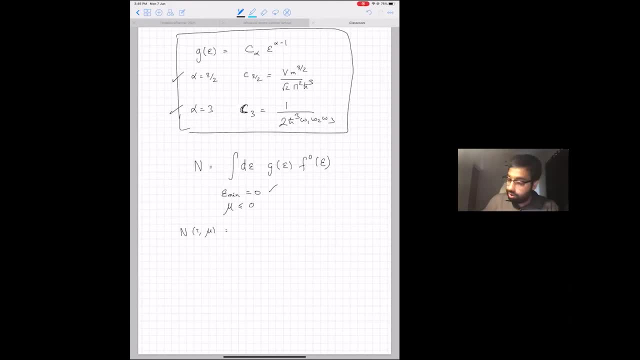 the expression for g of e, which will pull out a c alpha e to the alpha minus one one, over e to the beta e minus mu minus one. okay, so now, uh, what i can do is i can simplify the this integral a little bit. What happens is I can basically define a quantity x which is beta e. 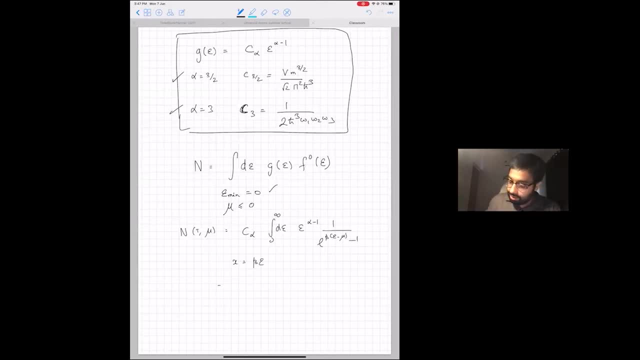 okay, and use that to write this n basically as c alpha. pull out this kt to the alpha 0 to infinity, dx, x to the alpha minus 1. let me call: bring back my e to the beta. mu right, that's my fugacity. and I have z inverse e to the beta, e to the x minus 1. okay, so I can write this: 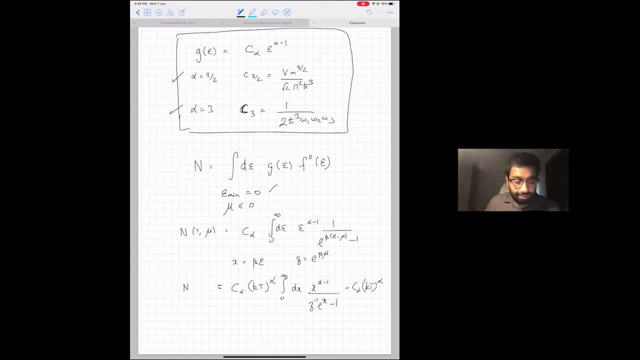 n, precisely as some c alpha, kt to the alpha times. some function purely of this z, because I'm integrating over x and depending parametrically on this alpha. so we have this g alpha of z. okay, and this is just some algebra. after doing this algebra, I can express this g. 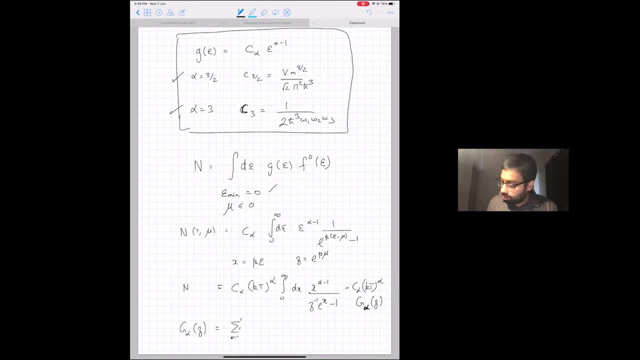 alpha of z as sum over m goes from 1 to infinity z to the m by m to the alpha times, the gamma function, where this gamma function, as you know, it's the generalization of the factorial function and it's simply given by 0 to infinity dx, u to the alpha minus 1, e to. 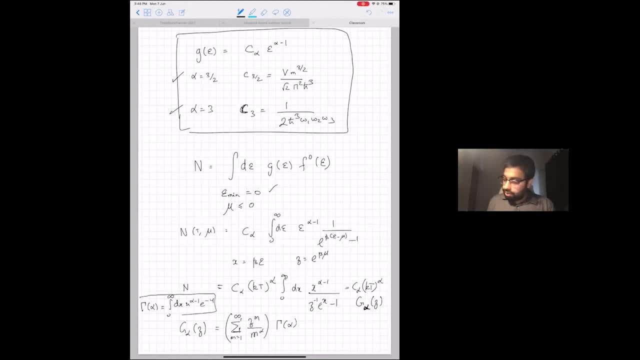 the minus 1. okay, so now this is the expression for g of alpha, so g alpha of z. now we can go back to this equation, because this is n is written as c alpha times, kt to power alpha times, g alpha of z. plugging this back in, now we can do some physics to see. 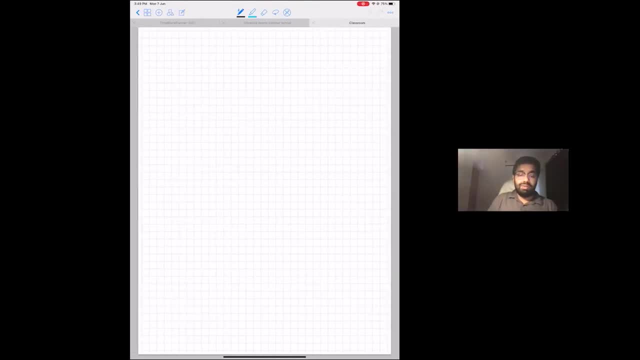 exactly what is happening as you go to lower temperature. so now, an important point here that I forgot to make is this: uh, integral, this integral. you can show that this integral 0 to infinity, dx, x to the alpha minus 1, z, inverse t, z, inverse m of xi, r, z, zero into new. 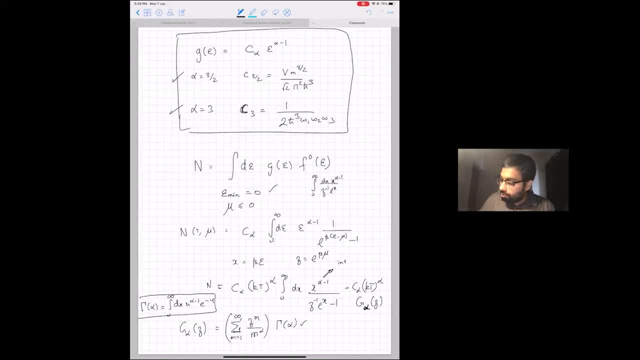 point here. so if the comparative analysis of this is really used in such situations. so what is the EST e to the x minus 1? sometimes these are called Bose integrals. this integral converges only when alpha is greater than 1. okay, so this is a mathematical property that will be very 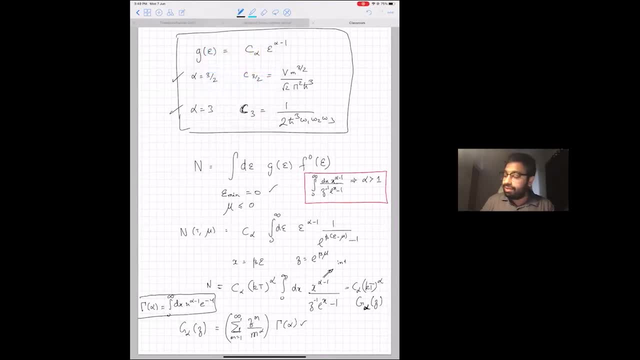 important when we discuss why, in certain cases, in certain dimensions, for example, you cannot have Bose condensation for non-interacting particles. okay, so let's keep that in mind, and now let's work with alpha greater than 1, which is true for both the important examples that we have. 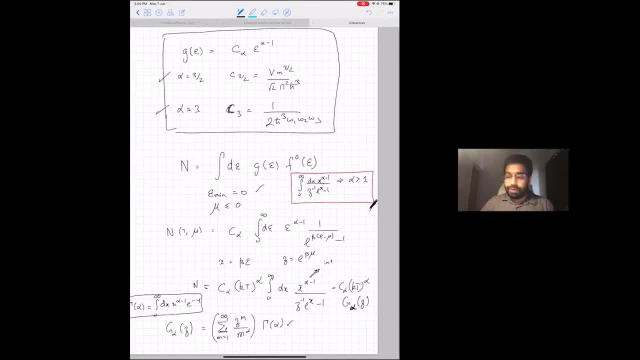 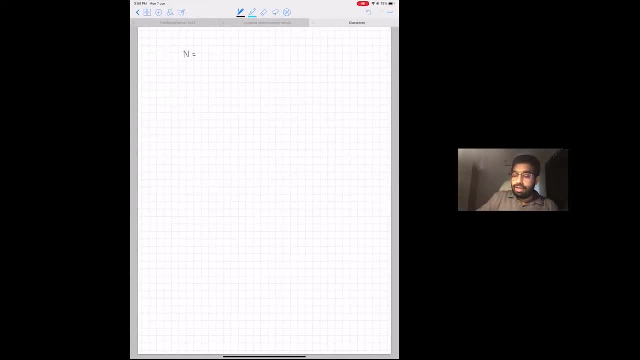 particle in three dimension, as well as our harmonic oscillator. so with that we can write our n as c alpha gamma of alpha divided by. I'm just bringing the kt to the denominator minus alpha sum over m. this is a series, in this fugacity, z of t to the power m. 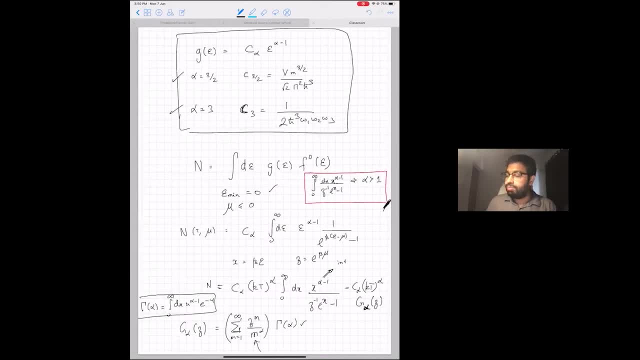 m to the alpha right. so that is exactly what we had. you can see that we have a series in this fugacity, z of t to the power, m, m to the alpha right. so that is exactly what we had. so that is exactly what we had: z to the m by m to the alpha. now, 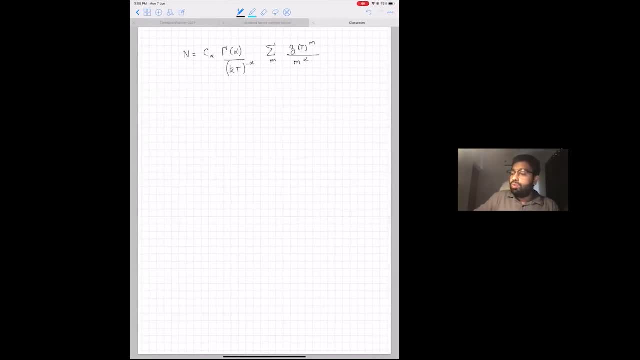 let's look at what happens to this expression as you go to lower and lower temperatures. so now, if you have the first point, is this function as a function of z? this is monotonically increasing as a function of z, okay, and z, remember, is e to the beta mu, okay. 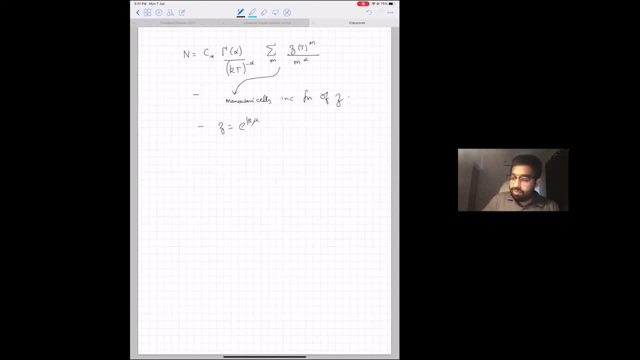 now, at very large temperatures, as we just saw, mu is very negative. mu is towards minus infinity, as t goes to infinity and z is much less than 1, okay, but now, as you go to lower temperatures, mu basically becomes larger. but mu has to always be greater than zero, right? so that's the maximum value it can take. sorry, mu has to always be less. 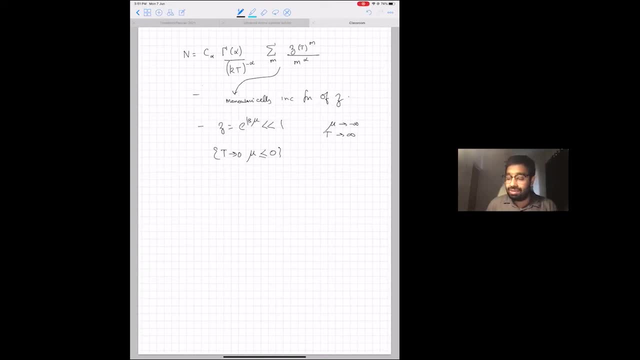 than or equal to zero. that's the best. that is the largest mu that you can take, okay, which means your z, basically, is increasing as your temperature decreases, but z is always has a bound. it is less than or equal to zero. okay, so that's the maximum value. 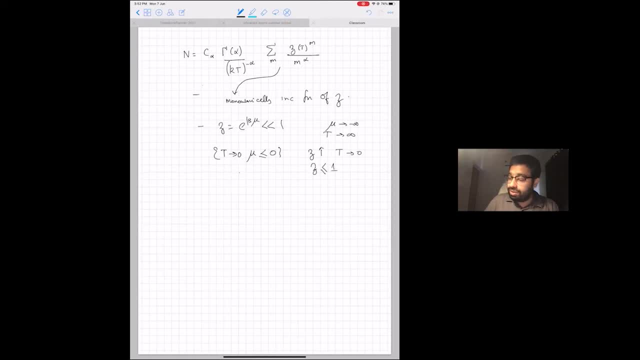 equal to one, because mu is at best zero. z e to the beta. mu has an upper limit, which is one. okay, so now, if we call and remember that mu is a function of temperature, let's call the temperature at which mu becomes very close to one, sorry, very close to zero, and hence z becomes exactly one. 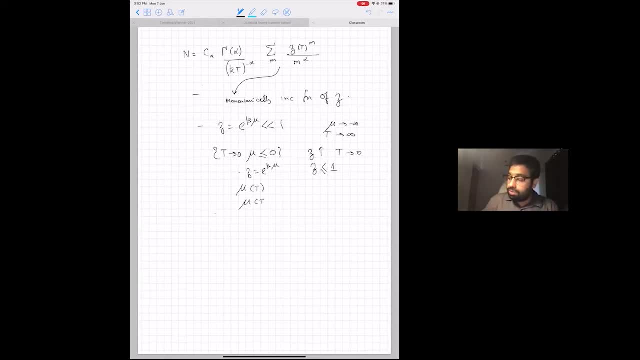 let's call the temperature when that happens, tc. okay, all right. so now, after this temperature, as you further decrease t to be less than this tc, what happens is basically your z is essentially frozen, z of t less than tc. it cannot become any larger than one. so z for all temperatures below such a temperature where mu becomes one. 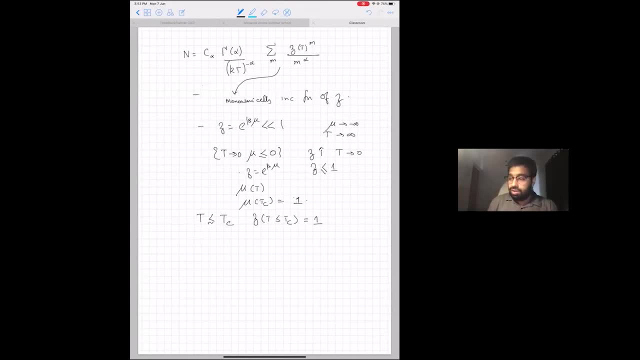 okay, it's just going to be frozen at one. what happens at t less than tc to this function then? so then you have this slightly absurd result that, okay, times kt to the power alpha when t less than tc. okay, what this is telling us is, as i keep lowering my temperature further and further below the 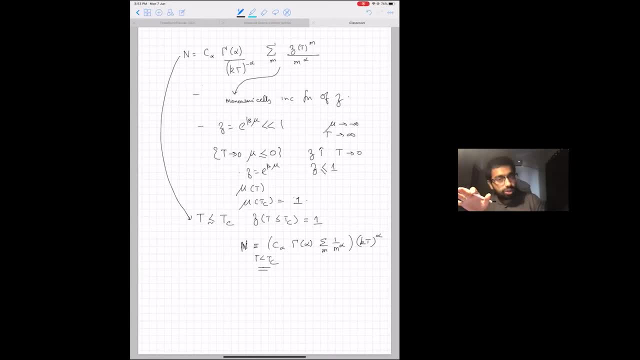 temperature after which my chemical potential has saturated to its lowest allowed value or highest allowed value, but lowest modulus, right new- as saturated to zero. as i go below that temperature scale, my number of particles really, because alpha is greater than one as t becomes closer and closer to zero, the right hand side of this function goes to zero, but the left hand side is a fixed number. 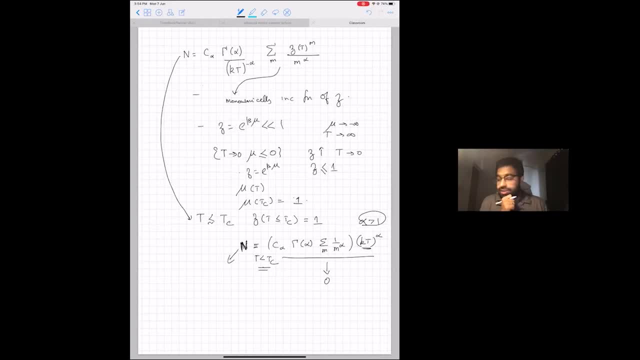 i have started with a certain number of bosons and it's very absurd now that this equation cannot be satisfied anymore. this equation predicts that some of my particles are vanishing. okay, what is happening? the answer is very simple. the answer is we made a very questionable decision here when we said n. 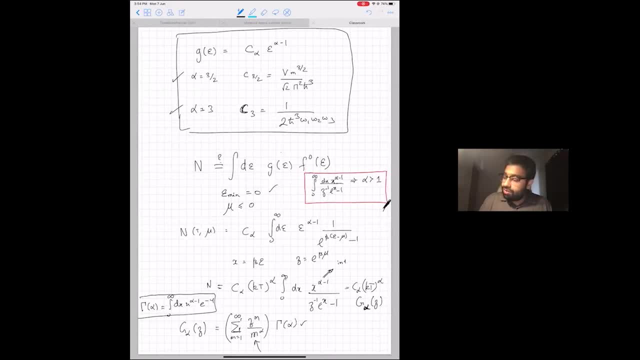 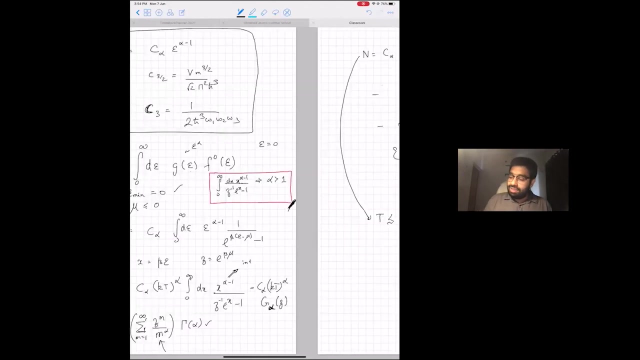 is equal to this. what have we done? because g of e goes as e to the alpha. this does not account for the occupation of the ground state, which is e equal to zero. so what we have to do, and what is happening essentially, is that once this temperature, 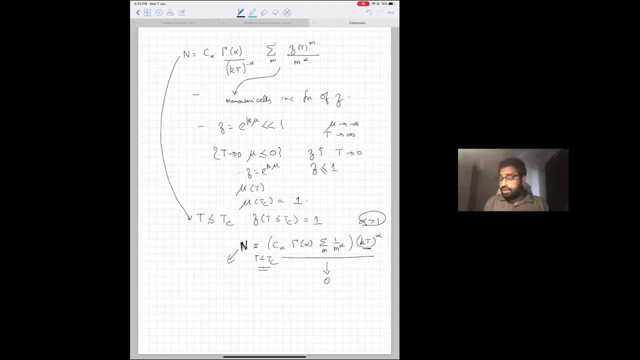 goes below this pc. all that is happening is particles are leaving the excited state and are disappearing into the ground state and they disappear into the ground state and, essentially, when that happens and when many particles start occupying the ground state below this temperature dc, that is precisely when you get. 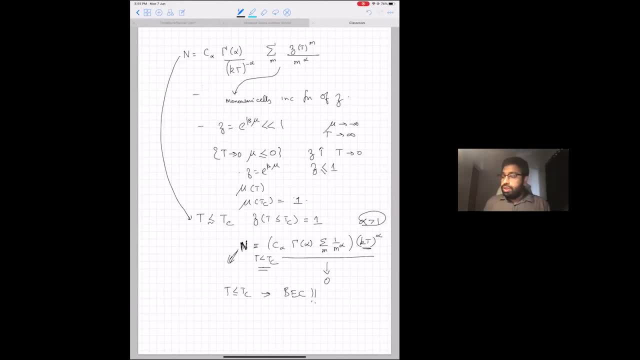 a, p, c. okay, so let me just finish by writing the final expression. for what is the transition temperature? first, by correcting the transition temperature and the temperature of the transition temperature. That is precisely pc. when you get a pc, the error, So the original expression I had was only the fraction of particles in the excited state. 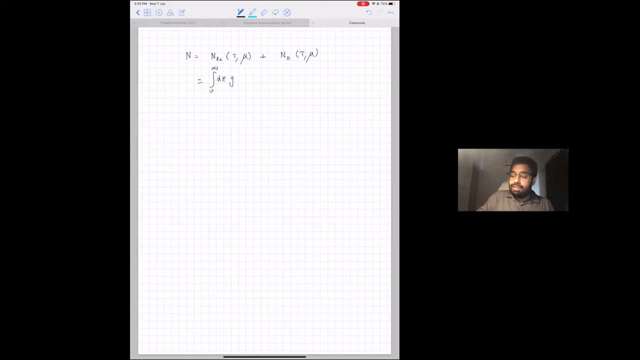 So this 0 to infinity, dE, g of E, f0 of E just signifies the number of particles in the excited state, but I can always have particles in the ground state. This part is essentially 0 at T greater than Tc, but it can become extremely large as T goes below Tc, and this is the right. 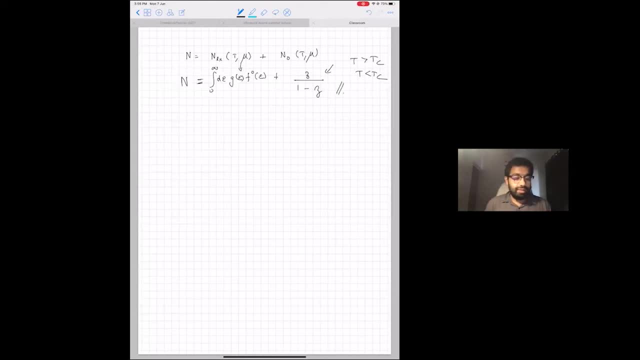 equation. to begin with, and this is valid at all temperatures, and this now- we define the transition temperature into Bose-Einstein condensate as the largest temperature at which, when we take mu of Tc equal to 0, we can accommodate all of our particles in the 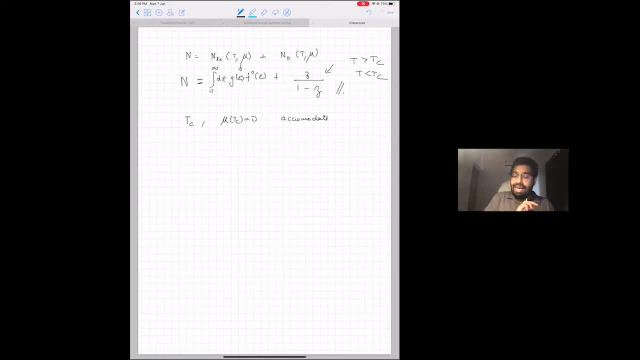 excited state. So basically we can essentially have zero occupation of the ground states effectively, ground state effectively and all the particles are in the excited states, which means I can write my total number of particles as precisely n excited Tc at mu equal to 0. okay, and once I just write this dE, g of E, 1 over e to the e. 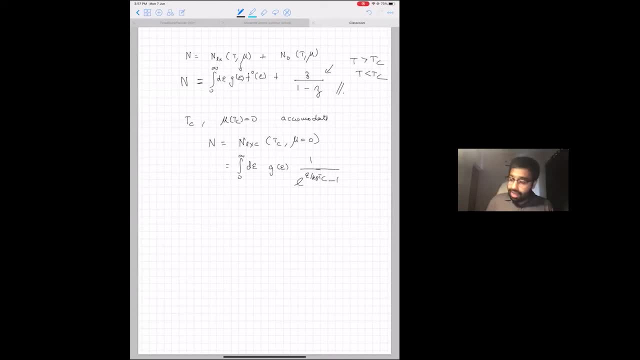 k, B, Tc minus 1. and I can use the same simplifications as before by redefining this integral, and instead of z is now 1, so 1 over n to the alpha, and from this I basically get C, alpha, gamma of alpha, k, B, Tc, and this is the famous Riemann zeta function. 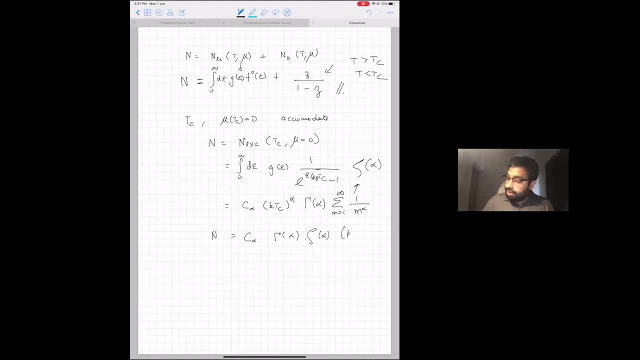 Zeta of alpha, k, B, Tc to the alpha, and you can invert this to write down the exact expression for the transition temperature for a Bose-Einstein condensate as n 1 to the alpha C, alpha gamma of alpha, zeta of alpha, and these are mathematical functions that 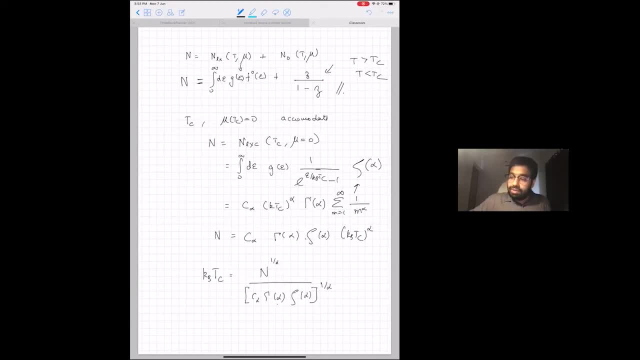 can be evaluated easily: Zeta of alpha, k, B, Tc to the alpha, and these are mathematical functions that can be evaluated easily. okay, so this is the transition temperature in some arbitrary single particle potential with density of states of C, alpha e to the alpha minus one with alpha greater than one. okay, 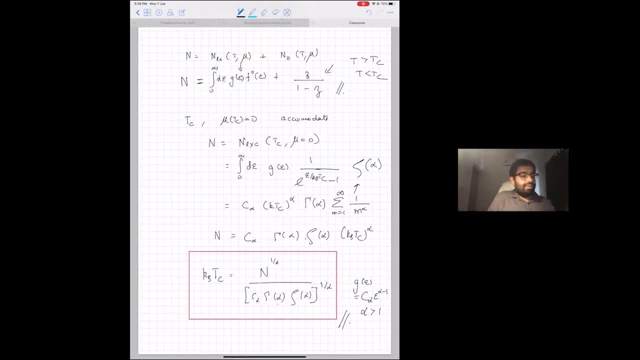 let me stop here and I'm happy to take some questions. sorry that maybe I took a little bit too long. I will be a little bit more conscious next time. if someone wants to unmute and ask questions, that will be easier and then I can also see some of the questions in the chat. 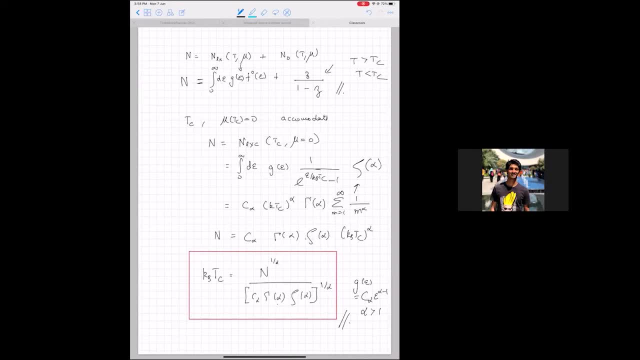 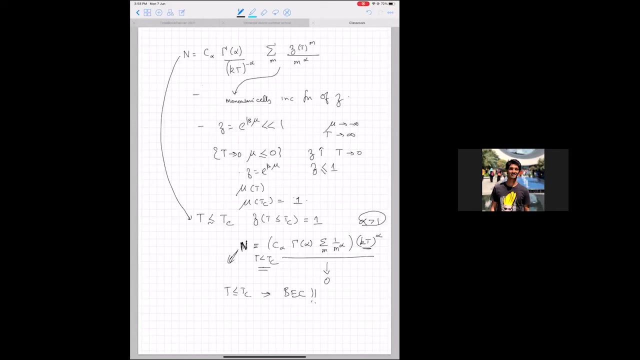 oh, so yeah. yeah, I couldn't completely follow where exactly we went from the calculation. we said that we had to add some ground state particles separately. I do not understand why this density of states does not account for the ground state. haha, so so it's. it's essentially because of the fact that the density of states 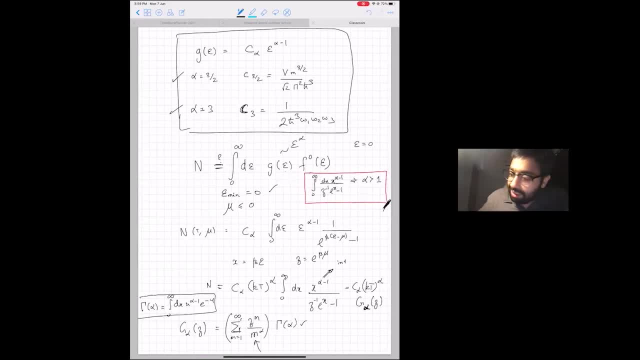 has this polynomial form right. so when e goes to zero, g of e goes to zero, that is only okay. okay, I mean, this is not some magic, it's just that I could have started exactly with this proper definition and given you this answer. but this is typically the way one introduces. 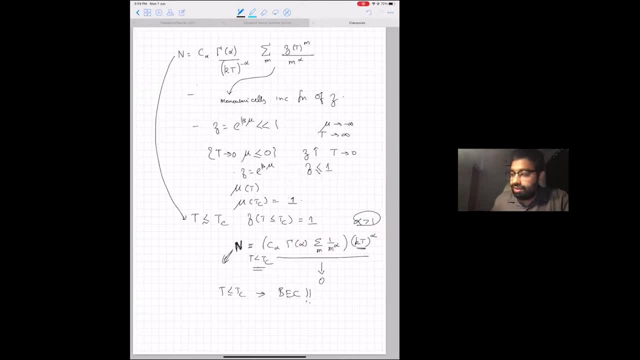 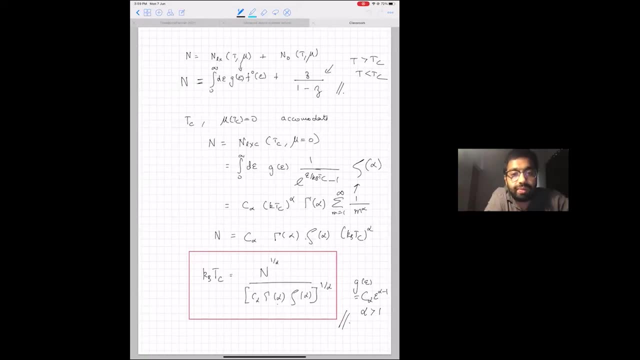 the Bose-Einstein condensate to show that, well, as long as you're about tc, you don't have to worry about the ground state at all. that is the main idea. any other questions? okay, so maybe I can just look quickly at a couple of these questions. 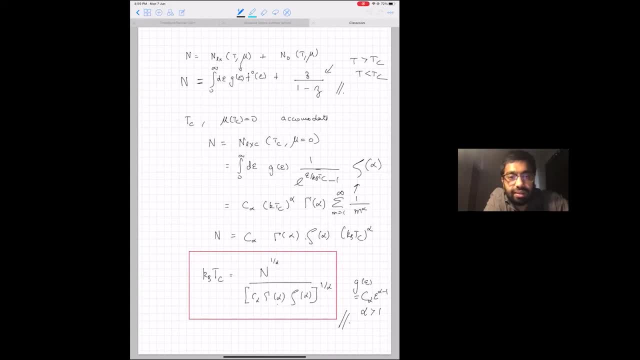 in the chat. so as the Bose-Einstein condensate is one giant function, will you be able to address the measurement problem of quantum mechanics using Bose-Einstein condensates? well, it depends on what one means by the measurement problem of quantum mechanics. well, if it is basically 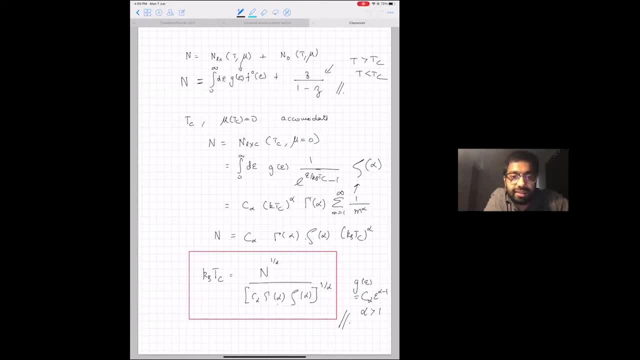 the fact that I cannot predict the result of individual projective measurements, then I will definitely know, because I don't think that philosophical, that that's a quasi philosophical question. there is not an obvious way to answer it using Bose-Einstein condensate, but one can learn about many facets of how to do a measurement and very novel ways to do a quantum. 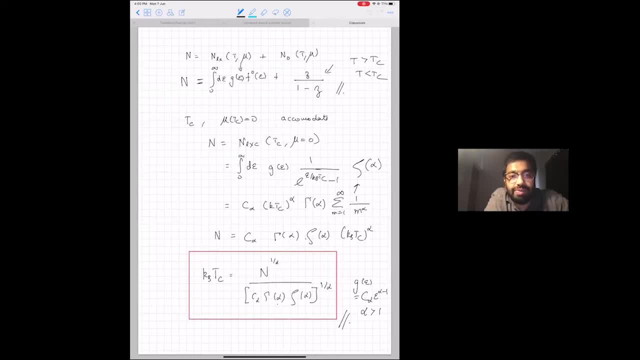 measurement with Bose-Einstein condensate. that is possible. we will talk about a little bit of that when we talk about BCs plus cavities. right then, then for the exponential to be greater than one, we would need: yes, that was my papa, I'm so sorry. yeah, that was my stupidity. okay, then Niyati asks: how do we ensure experimentally? 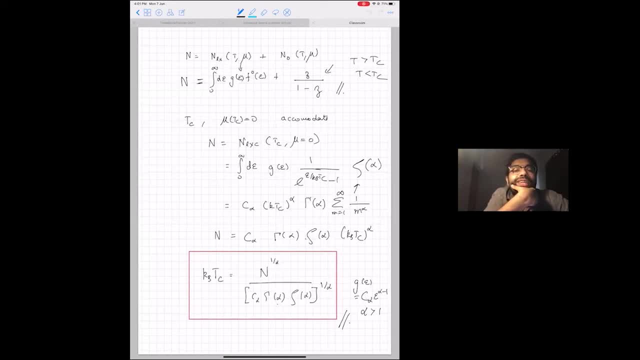 that mu remains less than E min always. I don't think we have to ensure that that is essentially satisfied by any bosonic. yeah, so our description- I'm it's theoretically when you describe it. we have to keep that in mind. it's not like you're keeping the 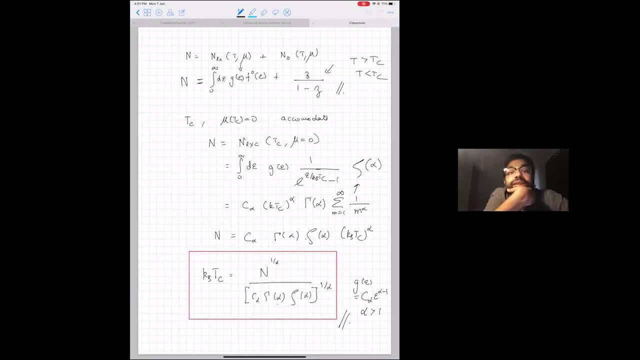 chemical potential less than E min. it is less than E min. okay, you are just assuming the general form of the density of states to be such a polynomial, right? yes, I am assuming the general form of density of states to be such a polynomial and of course this is valid for most single particle potentials. of course, if you put a very complicated 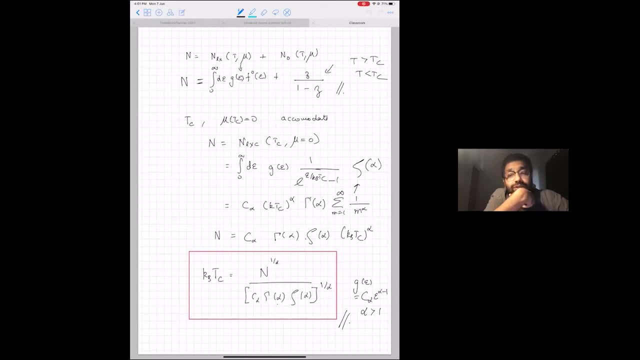 potential. sometimes you may not get such a continuous density of states and so on, but if you have a very complex potential, that's a very interesting question. if you have a random potential, for example, can you have a? you know that when you have a potential, that's over space. that. 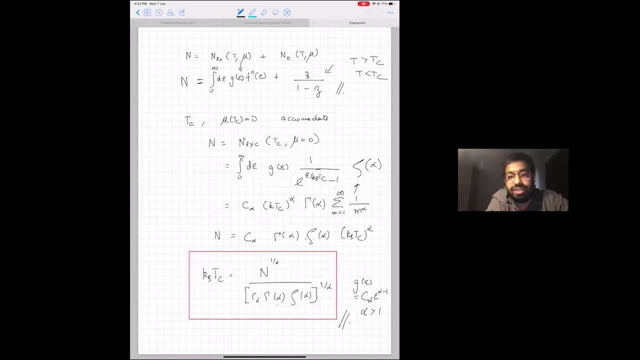 is random. this is very interesting in itself. can you have a boson instant condensate then that's? that's a very interesting question. but yeah, so we are assuming that we are not in such pathological cases, but generically this is the case, and I've also explained it by taking some examples that yeah.